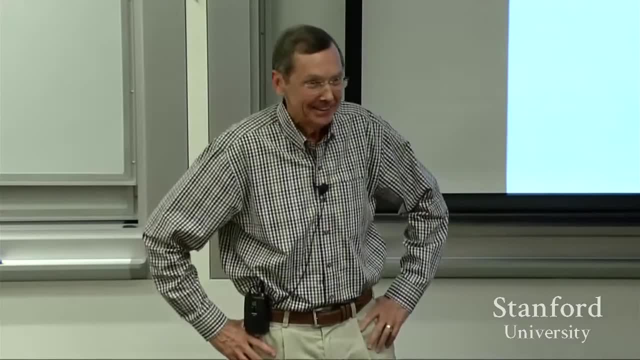 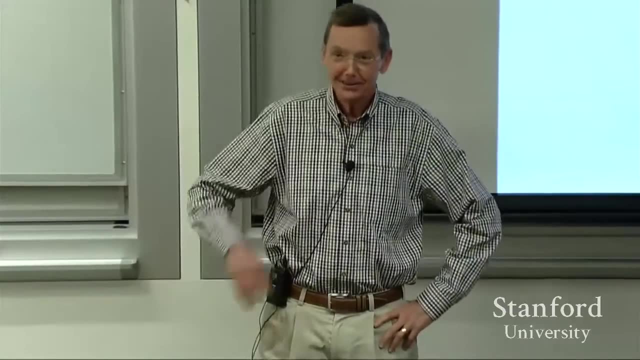 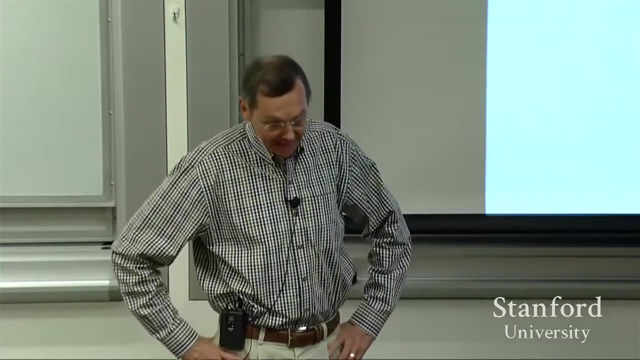 and see how it might play and cover the auditorium at 3.30 on Friday. So the title of this talk is Got Water. You know, that's like the mustache thing, you know. And the theme is urban water supplies in the arid west, And the subject that I'll be discussing is informed by that. 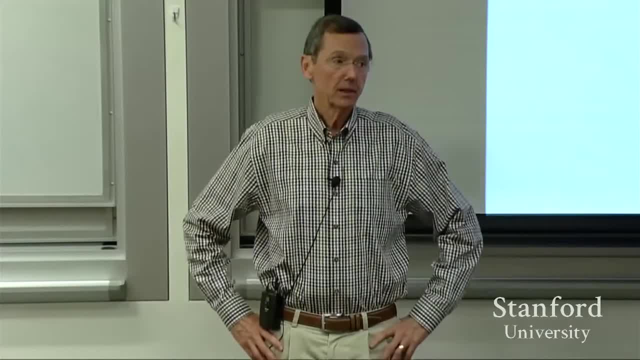 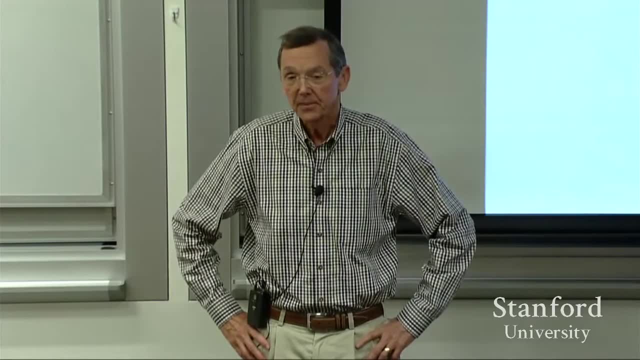 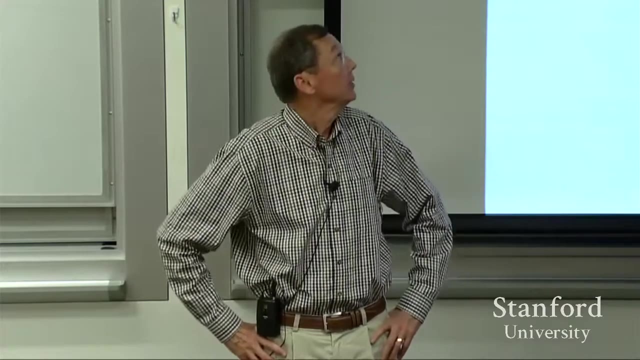 paper that I sent earlier and by our group of researchers, faculty graduate students, post-docs and others that are participating in a NSF engineering research center of which I'm the director, And the title of that center is Reinventing the Nation's Urban Water Infrastructure. 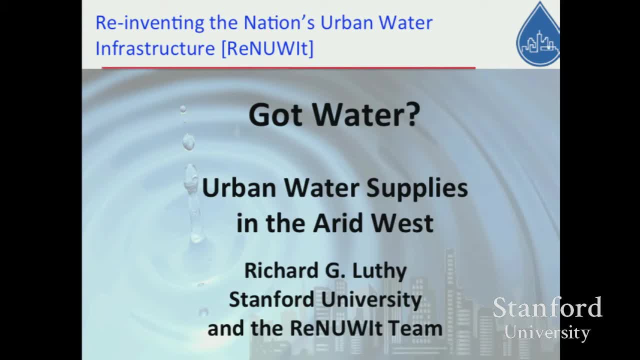 The center comprises Stanford, Berkeley, Colorado School of Mines and New Mexico State. So when I go through here I'll show examples that relate to the work in our center and I don't claim to you know, I'm not going to go through all the examples, but I'm going 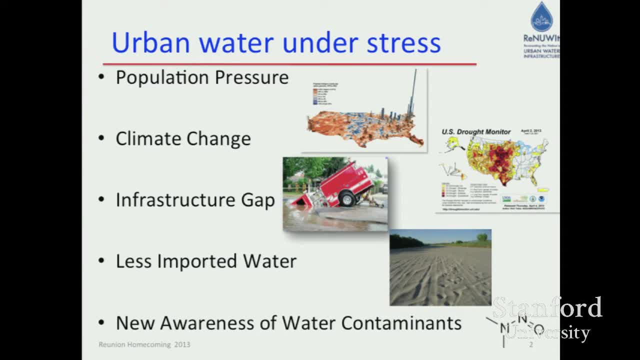 to show examples that relate to the work in our center and I don't claim to. you know, I'm not going to go through all the examples, but I'm going to show examples that relate to the work in our center and the person who does all this, but obviously I'm involved. So what is it that we think? 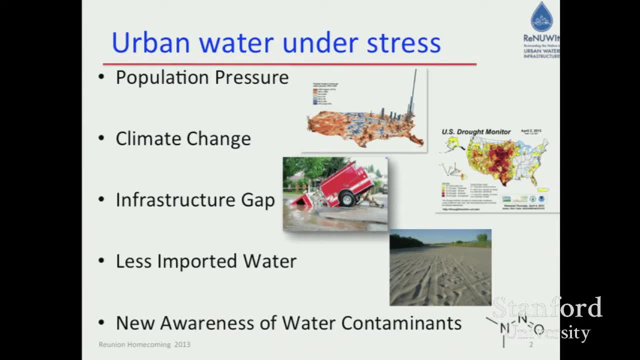 about in terms of urban water and in the west. One is that we have a population increase. If we were in Wisconsin or somewhere, there might be population decrease, or some parts of the Midwest We have people moving to what you might call the dry sunbelt. We also have 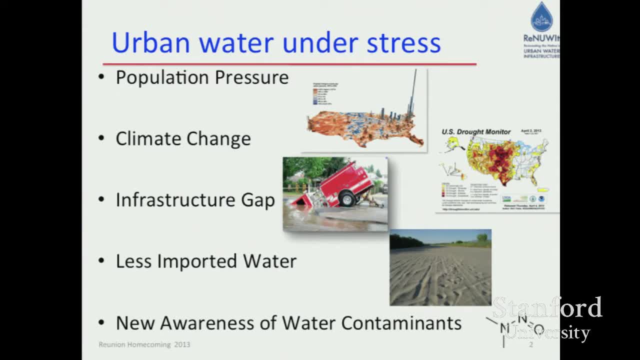 climate change, And up through the midwest we have people moving to the dry sunbelt, And up through the midwest we have people moving to the dry sunbelt. So it's actually been a deal that has got a rather dramatic effect during the last few years in its 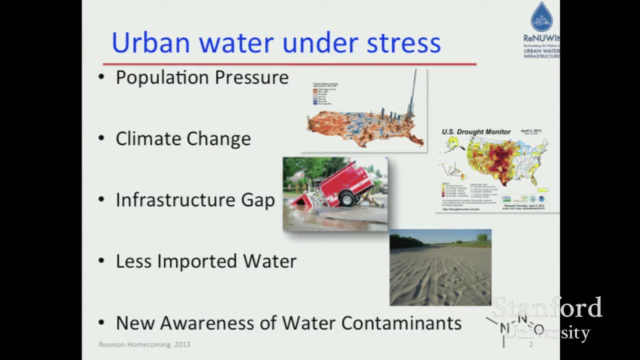 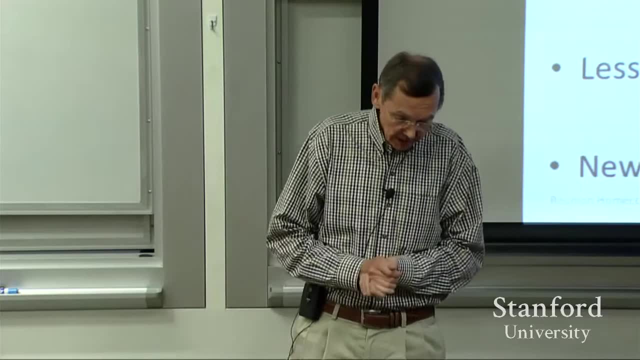 towards the pick this Collectivity 참łutớe 2021 on an increasing climate in the me, And we see that climate change will mean that it will be hotter and drier and our precipitation will come more as rain than snow, And that presents us. 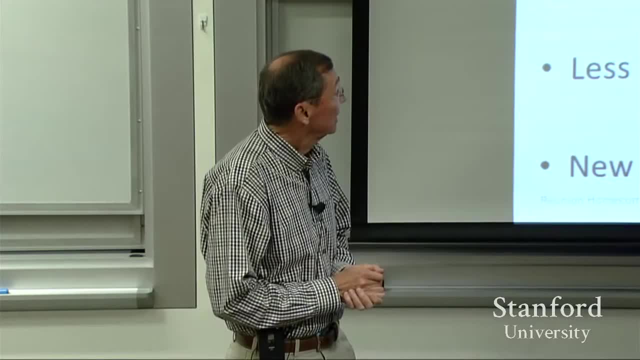 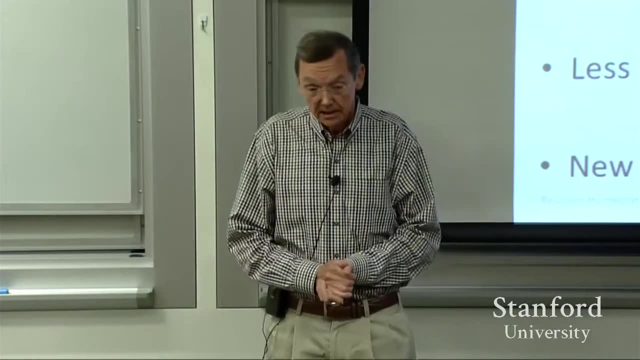 And that will come more as rain, that snow, And that presents challenges for us. Like all of our nation's infrastructure, there's gap in maintaining it And with our West and North reverses. West would now be flashlight condition, but relatively poor. with our water infrastructure, most of it is between 50 and 100 years old. 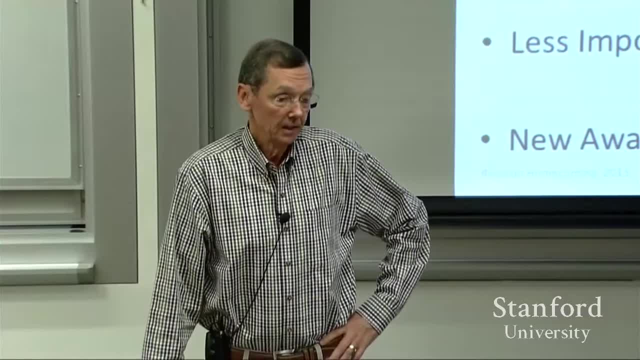 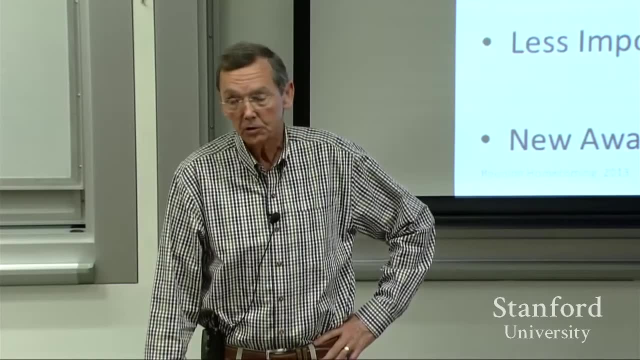 so, one way or another, it's at the end of its service life. so they're going to be lots of investments in urban water infrastructure, and what we can do now is look at the current system as it needs to meet these challenges and think about: are there new ways of doing business? 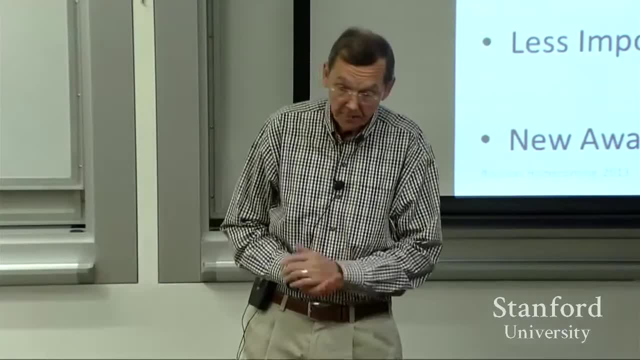 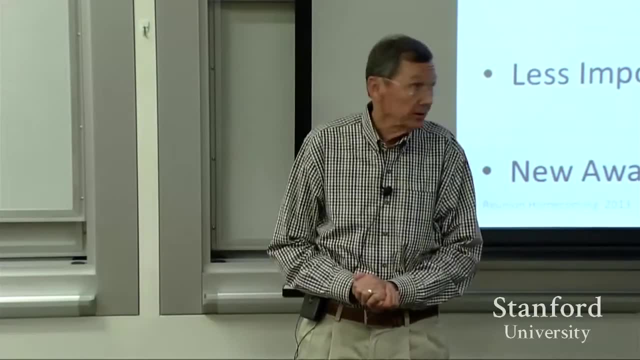 and can we do something different in the future to save money, save water and save energy? and part of the vision for the future is we want to rely on less imported water and also we recognize there's new water contaminants that we have to pay attention to as well. 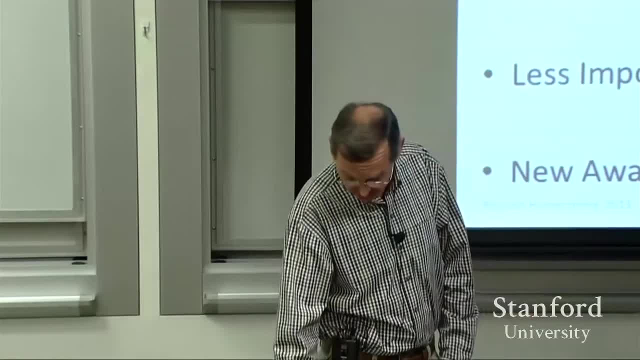 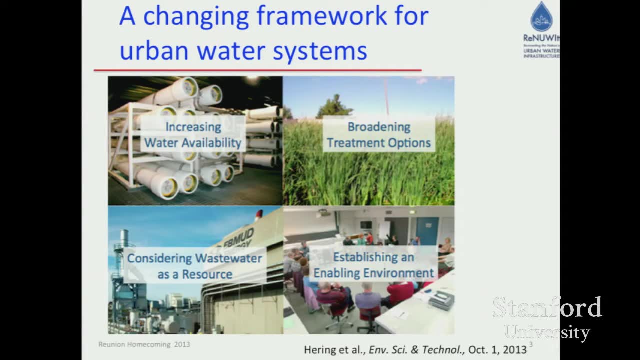 so how is it that we address all of these challenges then? the way we think about it is: maybe we could work in four areas. one is increasing water availability. that would mean like thinking, for example, of more water reuse, or maybe storm water as our source of our drinking water supply. 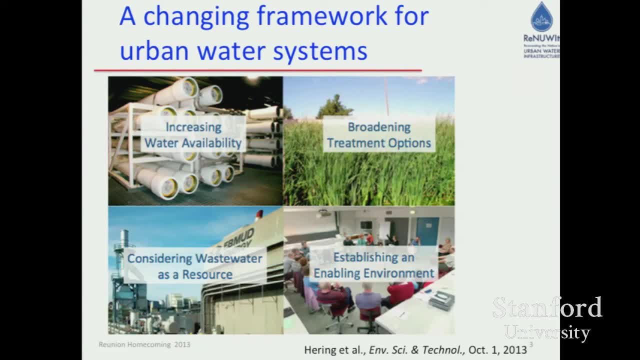 another one is in broadening our treatment options, and i show here a picture of a wetland doing new kinds of treatment and looking at the role that natural systems might play as part of our physical infrastructure. a third is considering wastewater not as a waste, but as a resource for energy and certain nutrients. 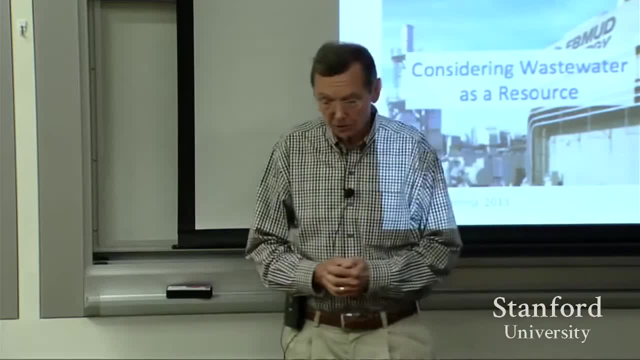 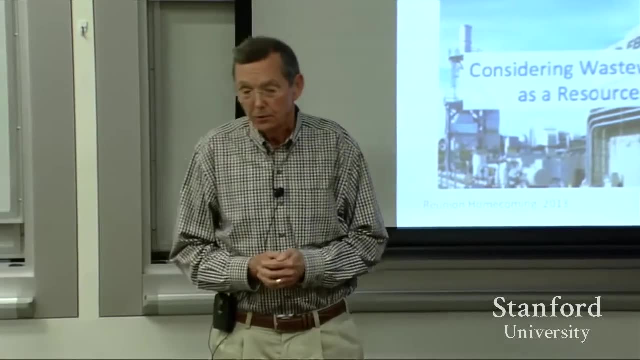 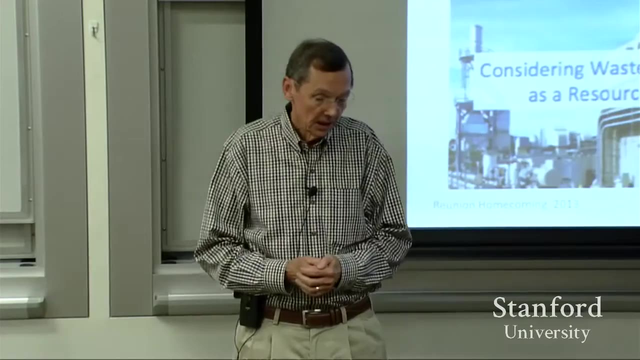 and then this one, which is important, is sort of the systems level thinking and integration. we're dealing with public infrastructure and public systems, so naturally there's a planning, social, political and economic process that takes place in the area in which we work, and we have to be able to address those. 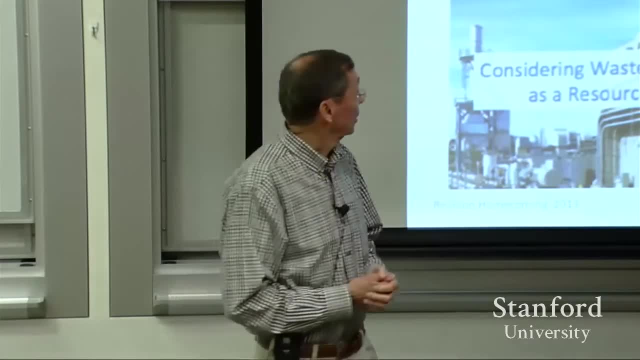 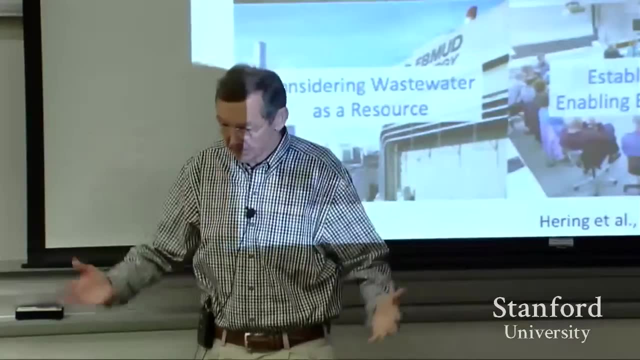 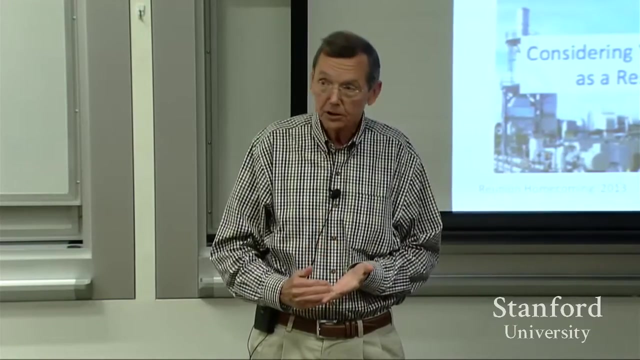 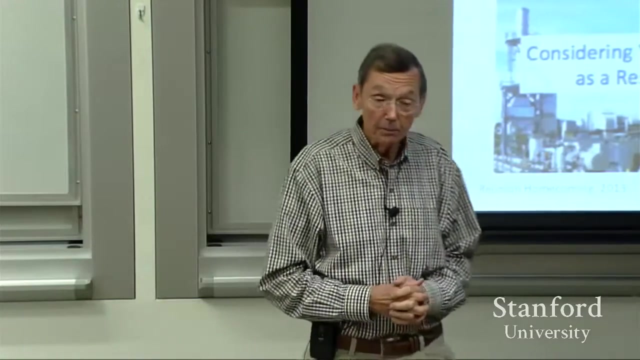 institutional issues, or nothing will change. in other words, we could have students doing the very best work in these three boxes, but if we don't understand how things are integrate at the systems level and how to address those scale-up issues, the regulatory issues, the planning issues and life cycle analysis, then we're just stuck. and what I mean by stuck is we'll. 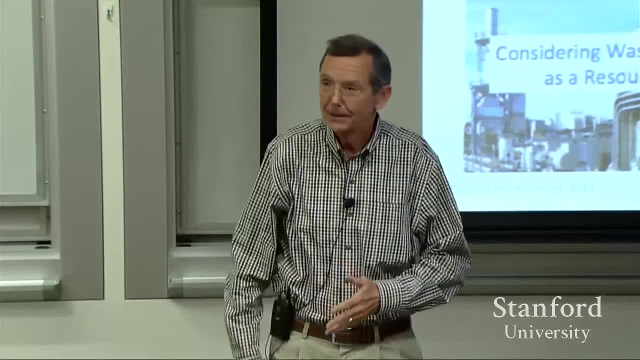 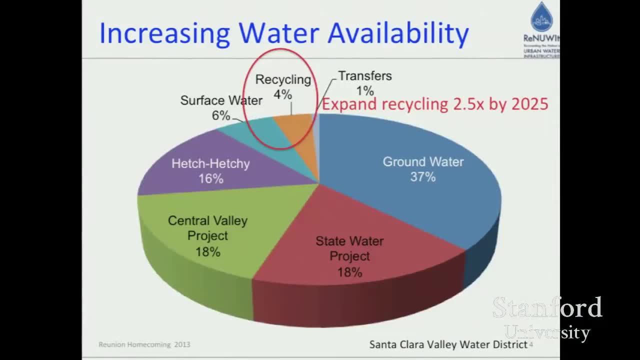 have published papers and students like Hannah will graduate, but we won't have an impact. so let's look at some examples here, and I'm going to just show you examples from a few examples from California and then one from Colorado. so this is a picture of where we get our water from in Santa Clara Valley. it's a 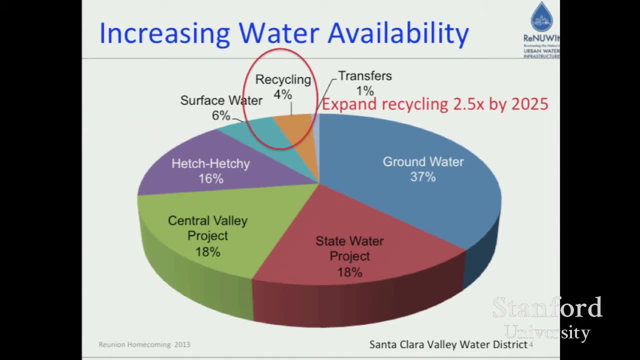 pie chart and obviously- and the pie chart shows where we are today- there's a a lot of imported water here. this Central Valley is imported water. it's pumped in, State Water Project is pumped in and there's a little wedge up there called recycling. now the goal is to more than double the amount of water that we're. 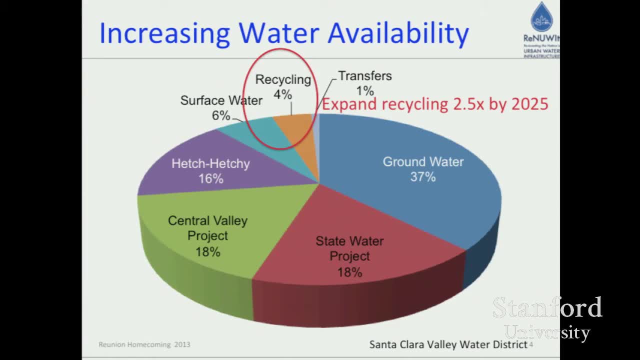 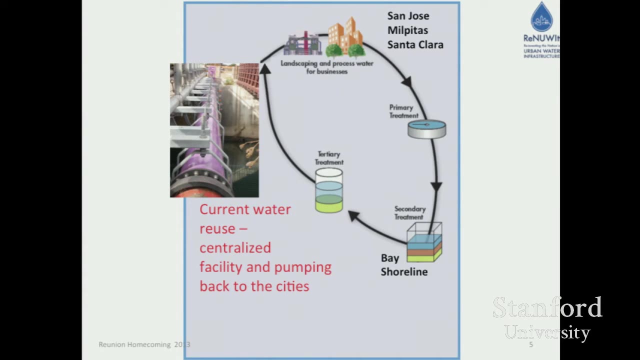 recycling in the next 10 years. in other words, that wedge is going to get bigger. so how well are we doing at that? and there's a picture here that shows the current situation. the wastewater for San Jose, Milpitas, Santa Clara, goes down to one base big. 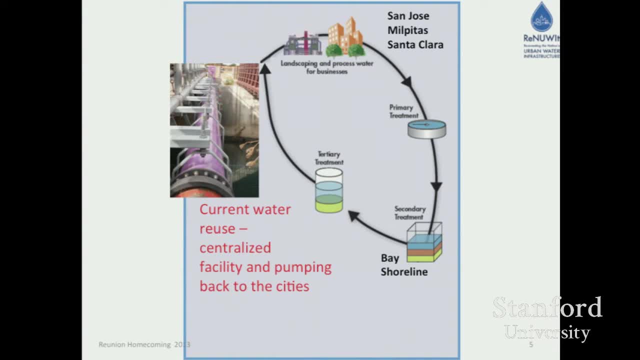 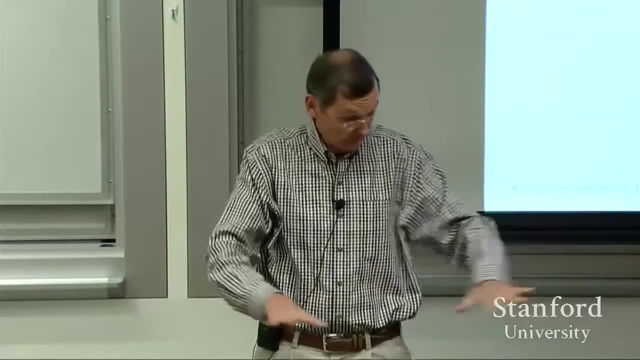 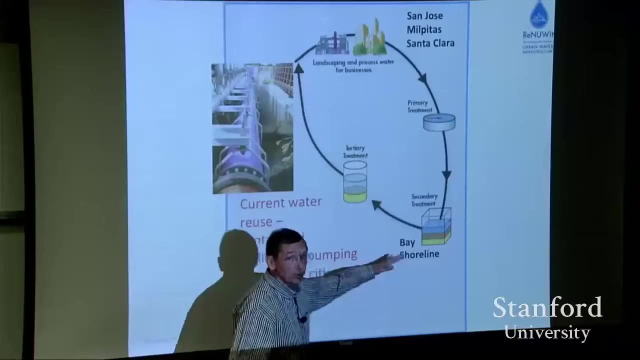 wastewater treatment plant. it's off 237, the south end of the bay, and if you, when you fly into SFO, you kind of turn and if you look out the window you can see this, this big plant. well, it does a very good job of treating wastewater and so water. 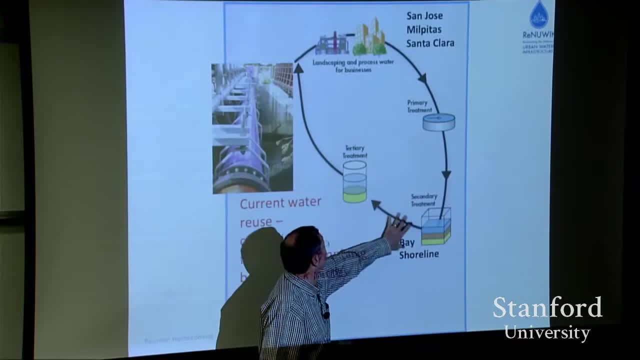 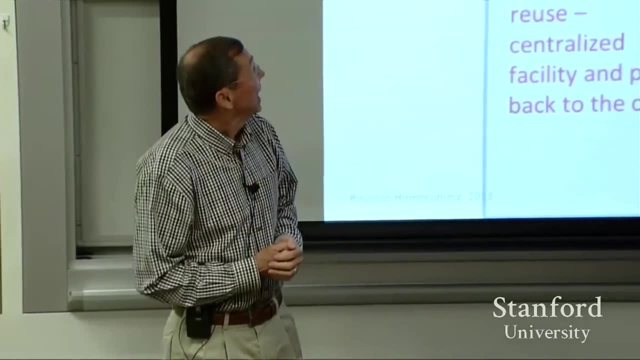 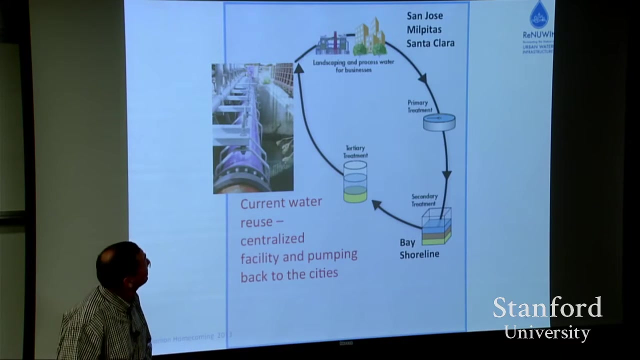 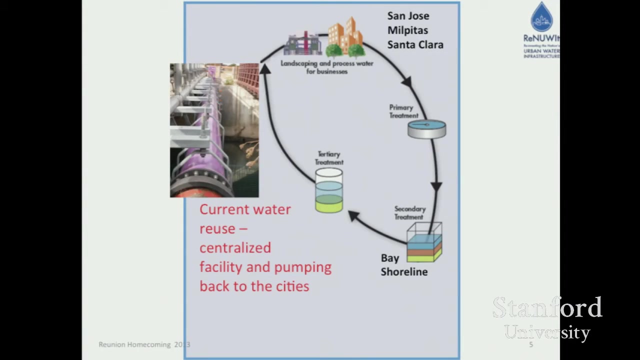 flows downhill to the centralized facility, then it goes through a few additional steps and then it's, it's recycled and it's redistributed through these kinds of systems. here that's a pipe and it's got a characteristic color, purple, and that identifies it as recycled water, and it's a. it's just what's done for code all. 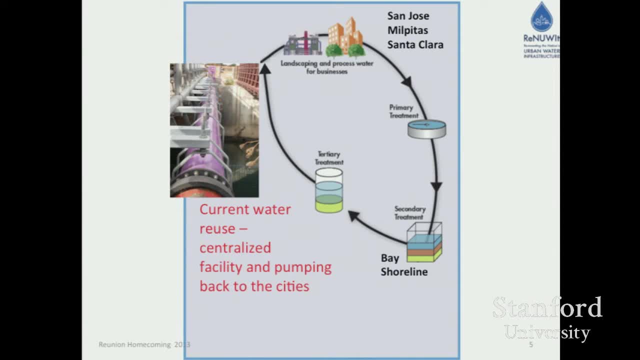 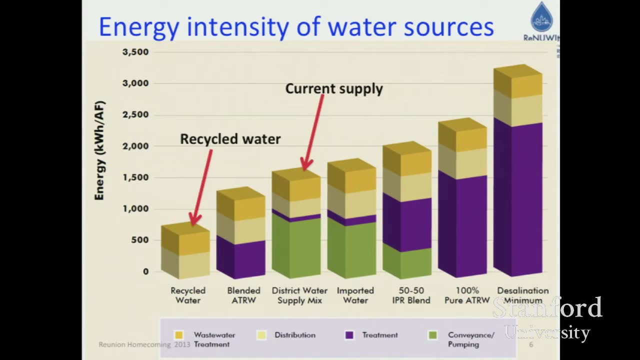 right. so we have the centralized facility and pumping back to the cities and that water can go around in a loop. the thing that's interesting about this is when we look at these energy that's required to deliver this water. there's a lot of benefits that come from. 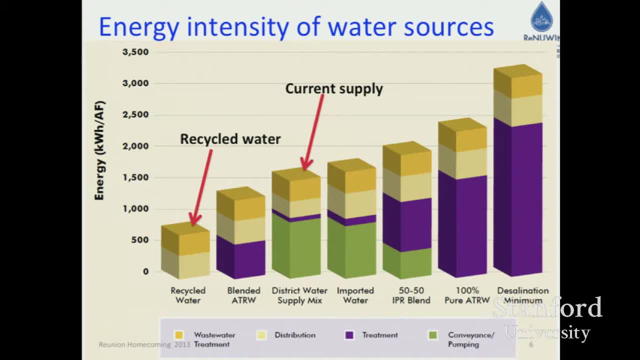 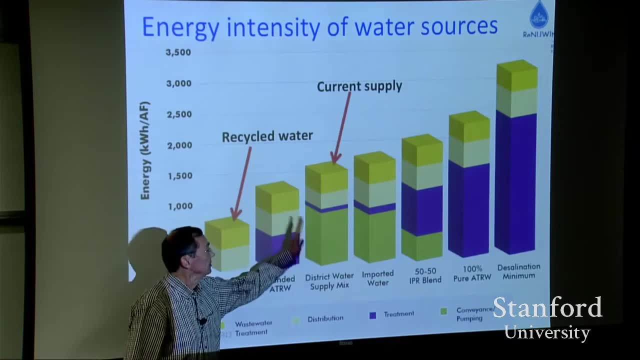 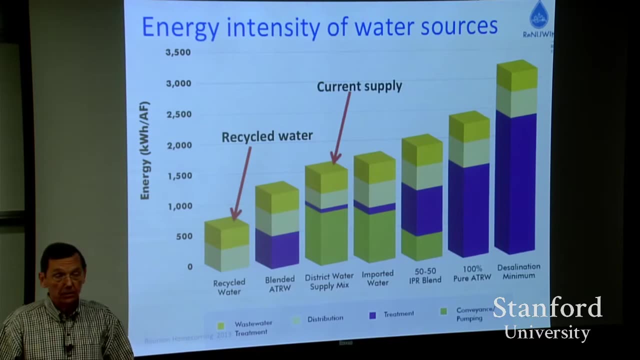 recycling water. so there are a number of little bars here, but the one I want to point to are the ones with these red arrows. this is the energy content, and you can forget about the units here, but just look at the height of that bar. that's the current water supply for Santa Clara Valley. this much of it, this big. 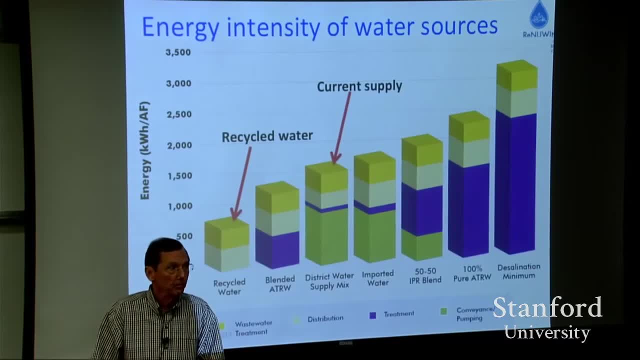 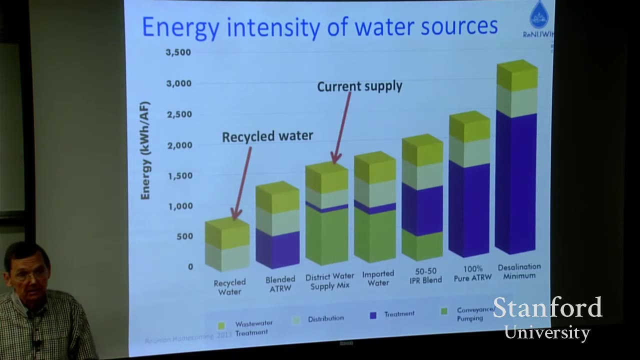 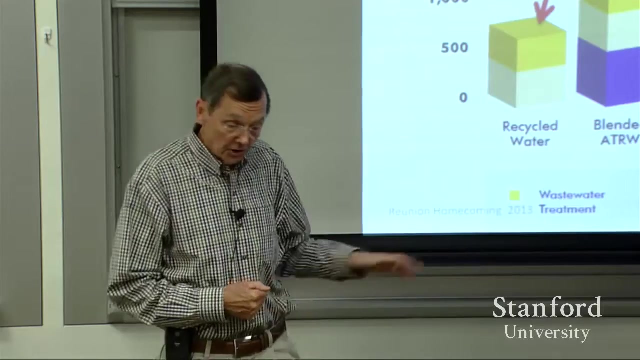 green part, that's the pumping of the water to the system from the state water project and the like. if we go to recycle water, we can. we're not paying for that big import fee, that energy fee, I guess, and we reduce the energy content by about half. so this is a good idea, but- but even here there's a fair amount of 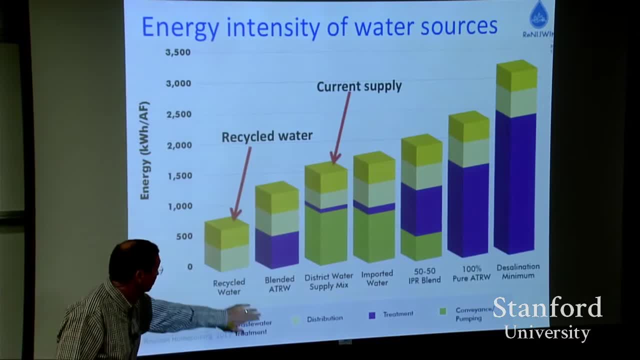 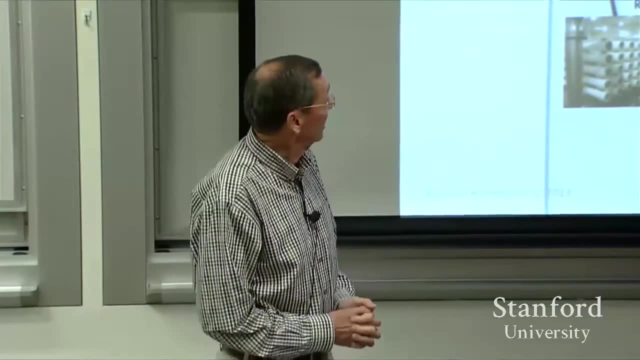 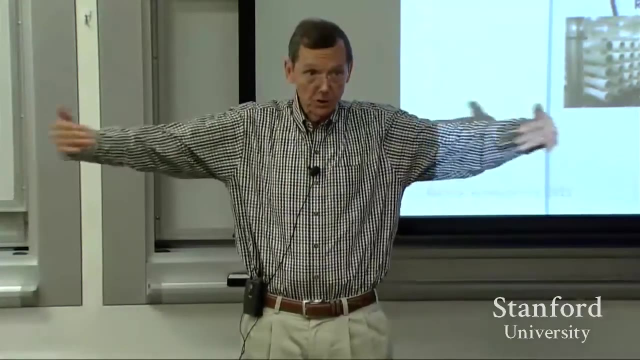 energy that's required to distribute that water in the system. so how is this system looking today? then there's a little bit of a problem when you have the centralized facility at the edge of the bay. you have these big sewer interceptors all coming down to the treatment plant, and we're talking about 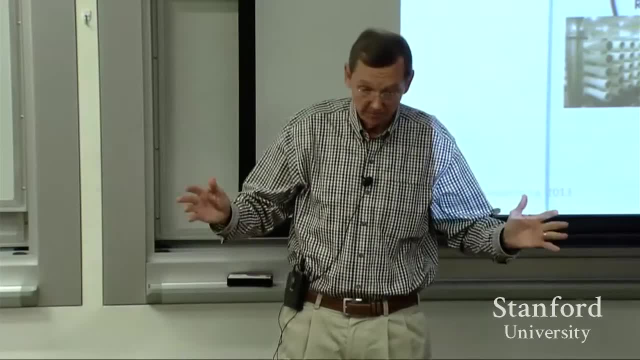 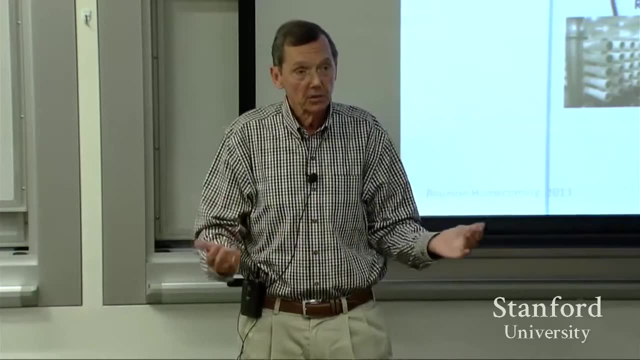 big flows here, like hundred, a million gallons a day or so. you have this big flow coming down to the treatment plant with these sewers, and the sewers will tend to infiltrate a bit. In other words, water tend to leak in, And that water is a little bit brackish. because you're near the edge of the bay. The end result is because of the salt content on the imported water, and the salt that leaks in the water is a little bit too salty to expand the reuse of that water. So what the city has built is a 10-million-gallon-a-day facility. 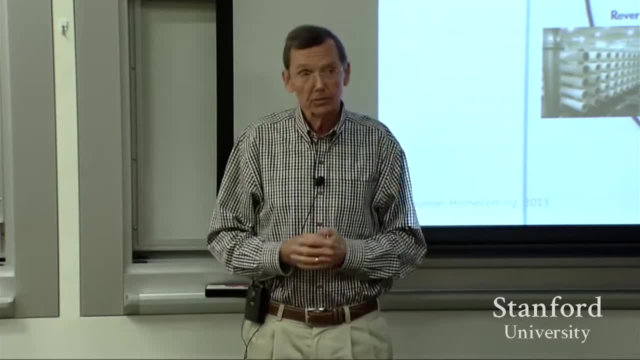 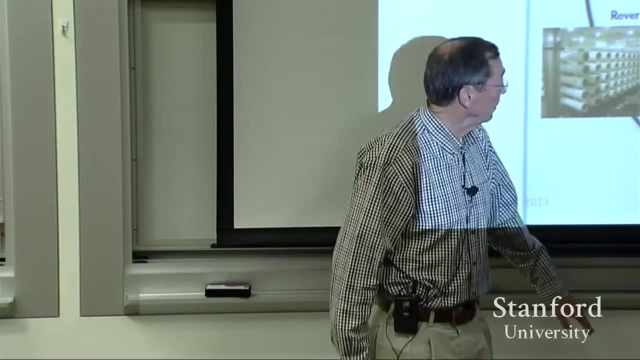 to try out ways to remove those salts Now. just think of sodium chloride. We're not talking big contaminants here, just simple salts. The additional steps are a series of nanofiltration, reverse osmosis and UV disinfection. 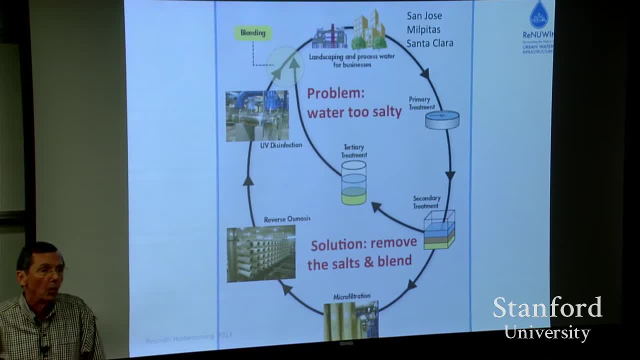 Basically, when we're all done with that, we produce something that's essentially drinking water, And the idea here is that we're going to use what we have here. now is we re-blend that in that recycled water. You have something like distilled water with this salty water. You mix the two together and average it out and you get the salt content that you want. So even with this treatment, this is still less than imported water, even though you have to provide this extra energy here. So that's the situation today. 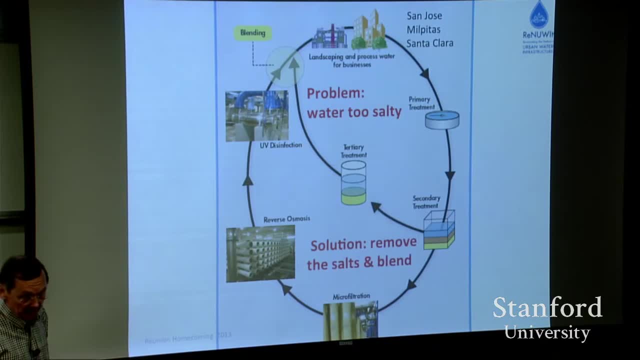 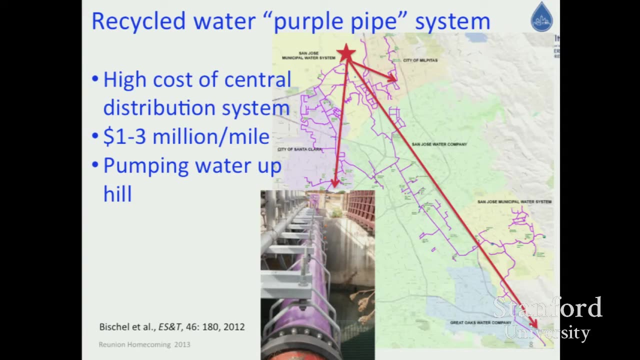 The question is: can we do better than that? And the answer is: well, if we had to redesign the system, we might rethink the idea of these centralized plants. So that star up there is the central plant and these lines here are that 130 miles of that distribution system. 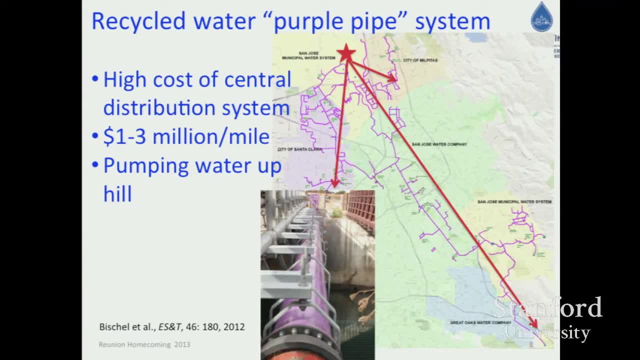 the reverse plumbing system. Now, what's expensive here is putting in those purple pipes. If you have to dig up streets in a city, you're on the order- about $2 million a mile or so- to put those pipes in place. Also, in this case, you're basically taking water. 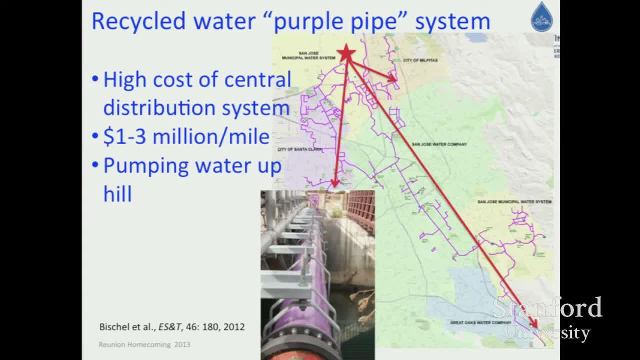 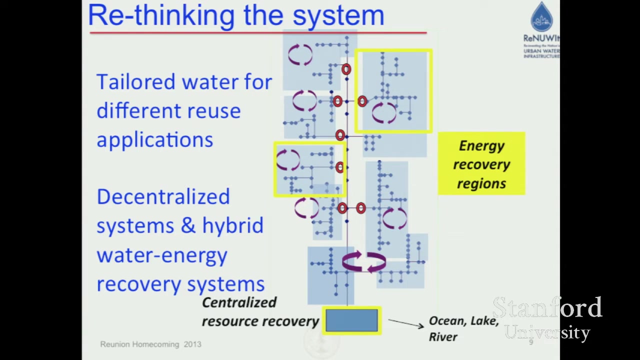 from where it was used and generating it, letting it flow all downhill, treating it to a high degree and then pumping it all back uphill. So one vision of rethinking our systems here was that maybe we should imagine our future water supply and wastewater systems being more distributed than centralized. 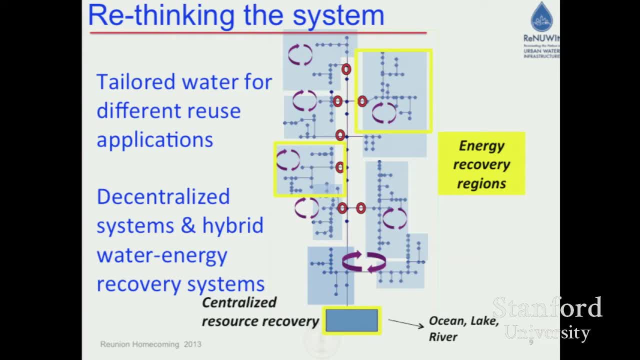 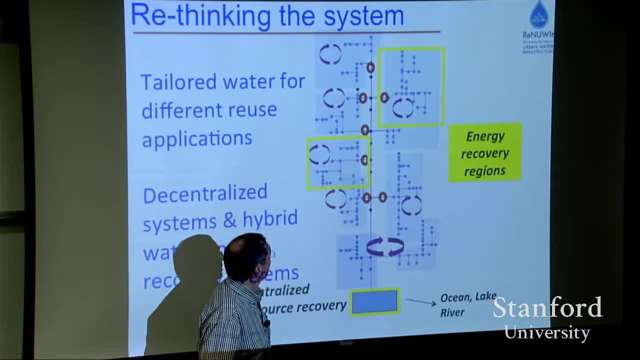 And how might this work? Well, this would be an example of what you might call a sewer shed, kind of like a tree, where different communities are sending water to a centralized facility. And let's imagine this box up there in the right corner. 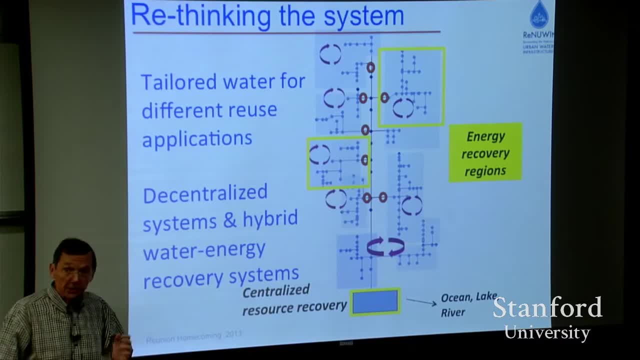 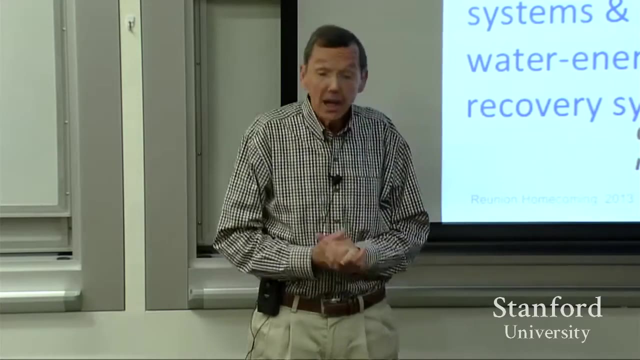 It's Stanford campus. We could imagine building a wastewater reclamation facility right here on the Stanford campus, over by well, behind the credit union. if you know where that is off, Bon Air Siding where all the dump trucks are. Demonstrate how we could reclaim water. 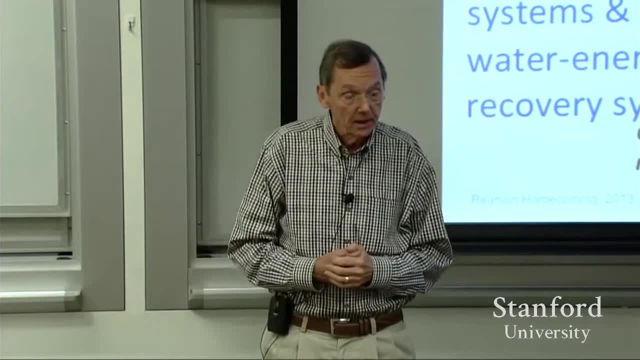 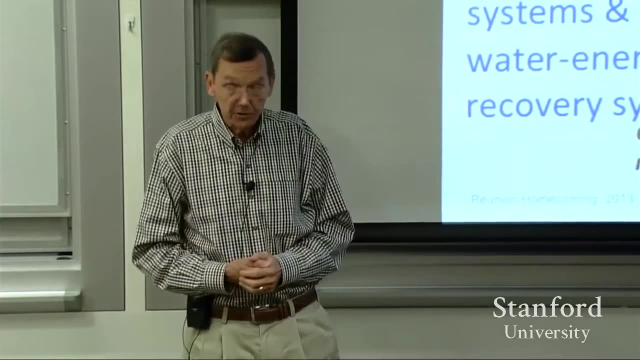 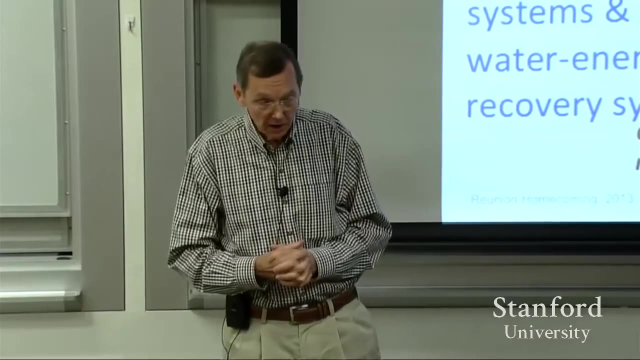 that would be suitable for irrigation on the Stanford campus. Demonstrate how this can be done with energy recovery. So it's energy neutral or maybe energy positive, And from a pilot experiment or something that would be on the scale of maybe 10 or 20 gallons a minute. 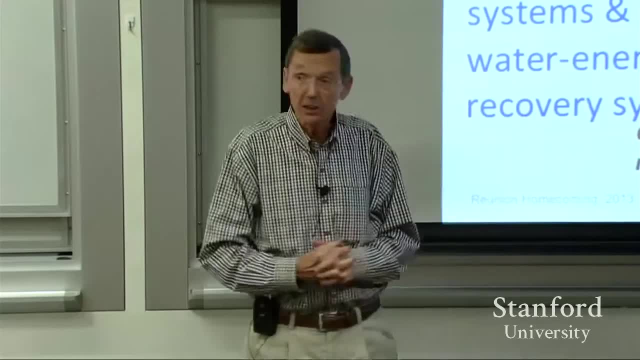 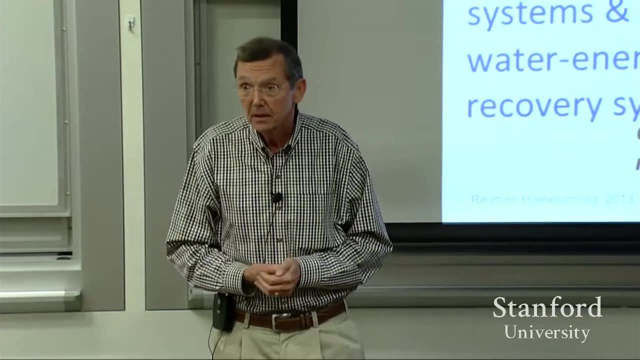 then we could use that as a testbed to say: would this vision really be realized? Could we actually expand this out and treat the million gallons a day of wastewater that comes from the Stanford campus? So the idea here is this kind of a system would provide several benefits. 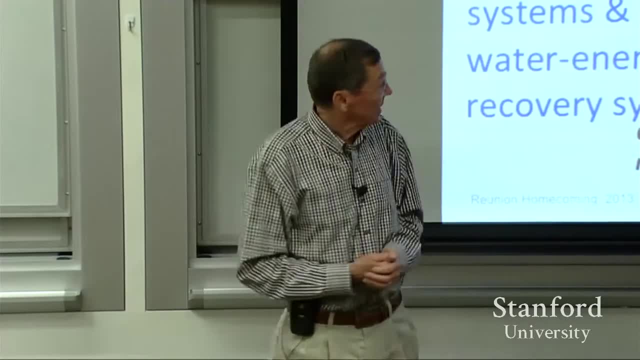 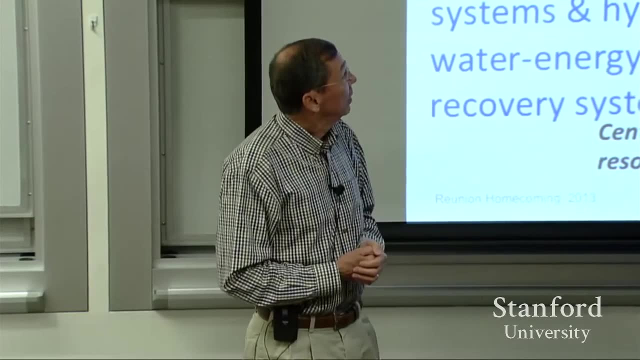 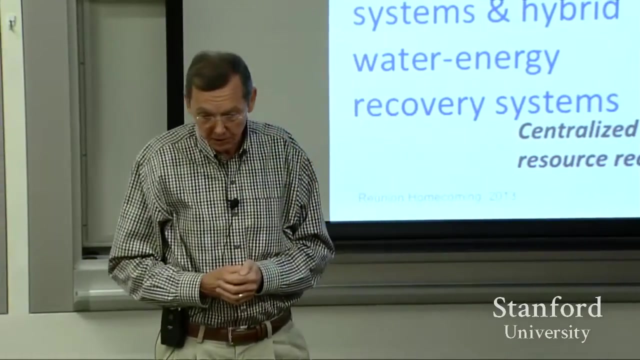 Uh, not only does it allow us to meet our future water supply needs on the Stanford campus, but we would also have a system that we're recovering energy and we're being able to do this water recycle in a much more efficient mode, And this is what we have in planning. 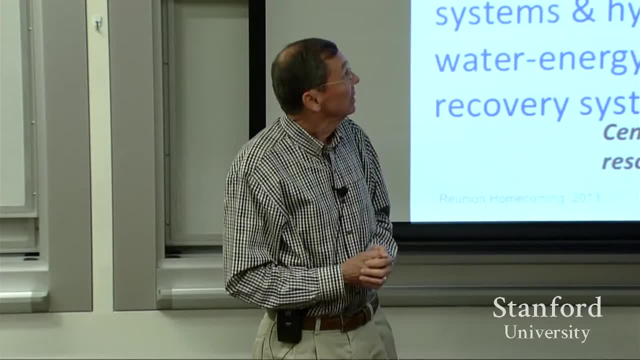 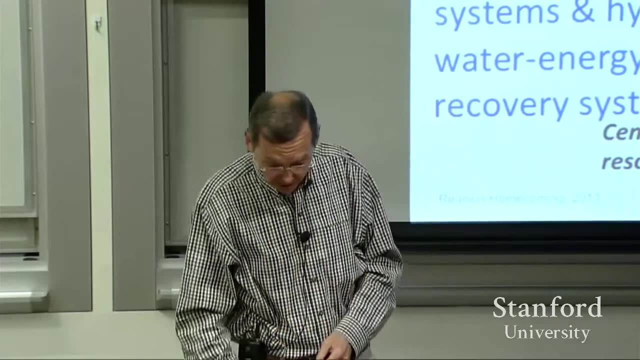 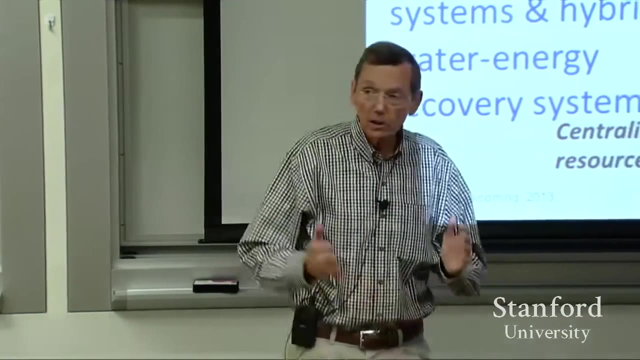 to actually demonstrate on the Stanford campus over there at a pilot facility- Uh, that's, that's in design right Now to test out technologies that would allow us to achieve this vision. When we look at Stanford, it's sort of obvious in a way that maybe we would make a good sub area for. 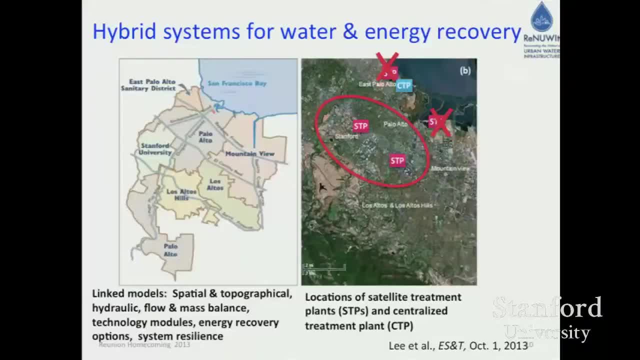 study or for trial, because we're- you know, we're kind of self-contained And all the sewers on campus go to one place, and that would be the place you'd want to tap in. But when we look at the problem here, this is just. 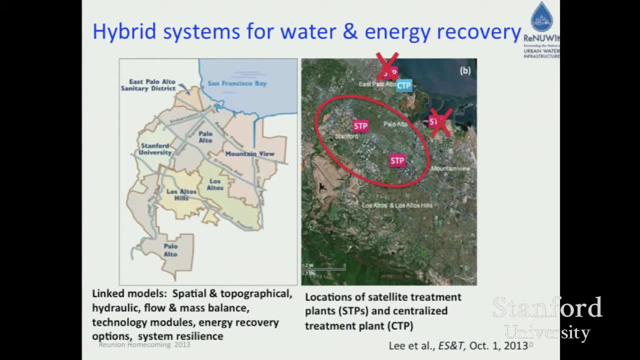 this is the sewer shed for the Palo Alto, This is the water quality control plant, And when you begin to think, well, how's this really going to work in practice? You end up with lots of issues to discuss here that are like: 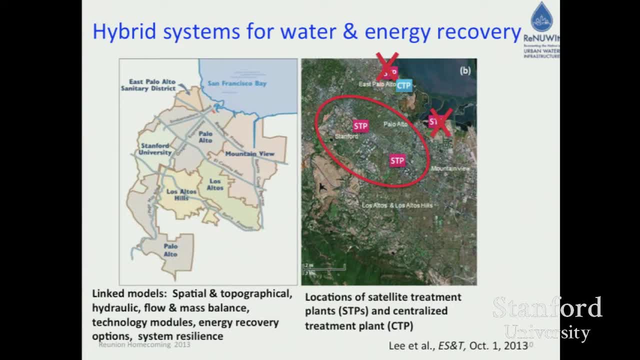 well, what's the spatial configuration? What's the topography? Oh, what's the hydraulic models? What's the flow and mass balance? What kind of systems would you put in a satellite treatment plant? You have all kinds of technologies to choose from. 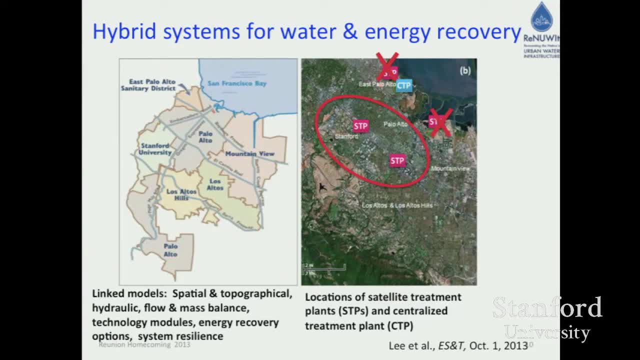 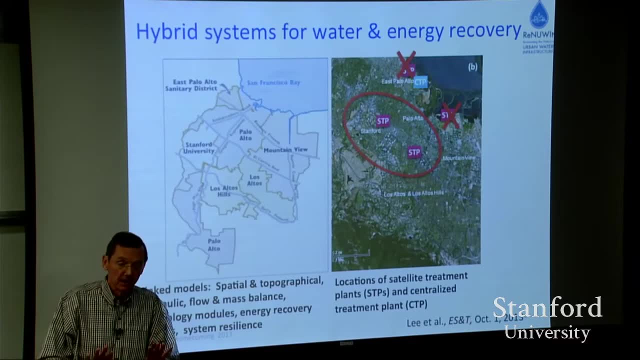 Would you do energy recovery or not? What's the resilience of the system? Well, you could ask. you could put more issues here, But you can see right away how you'll get so many combinations and permutations that, if you really want to think this out, 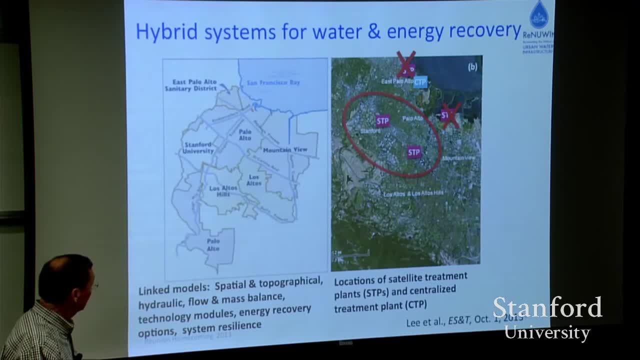 it becomes a complicated problem And we've been using decision analytic tools coupled to technology modules to address the issue of: well, what would be the right vision for this system? And the vision would be: control, would be a couple of satellite plants and still the centralized facility. 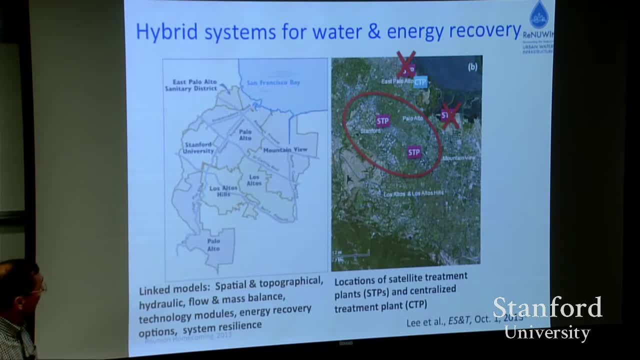 though doing something a little bit different in the future. So, thinking through this then, how does that vision of that satellite treatment plant work? It's kind of tricky to say where exactly and how, And so this was our first test case at that. 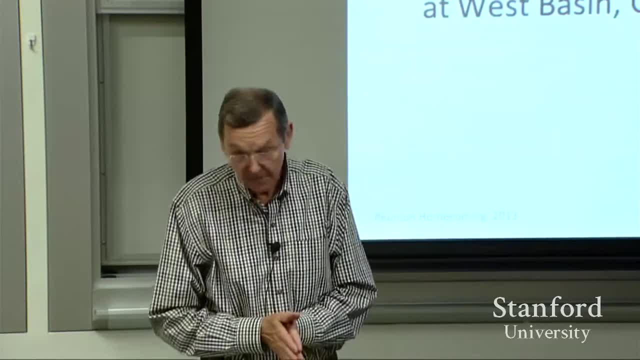 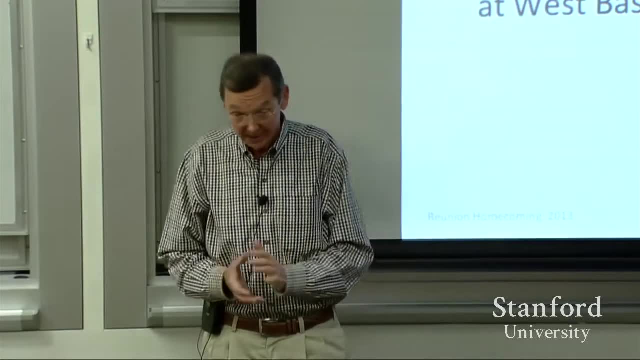 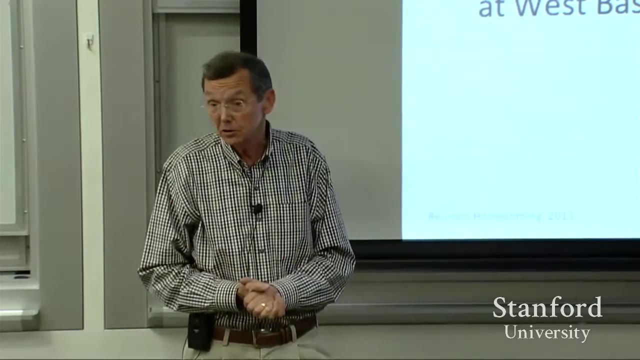 The other thing is when we look at these purple pipe systems, we're producing here typically one water quality all the time, And we can do better than that. You'd think maybe I should be able to produce waters of different quality depending on what its intended use is. 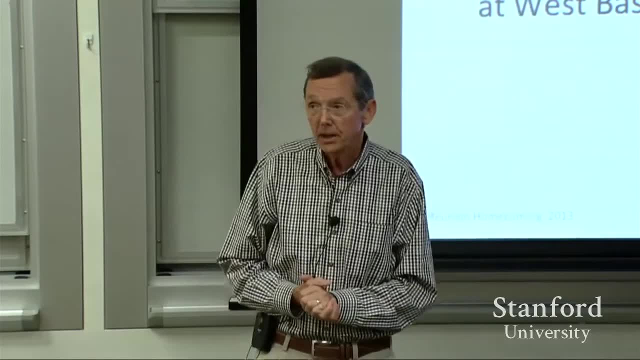 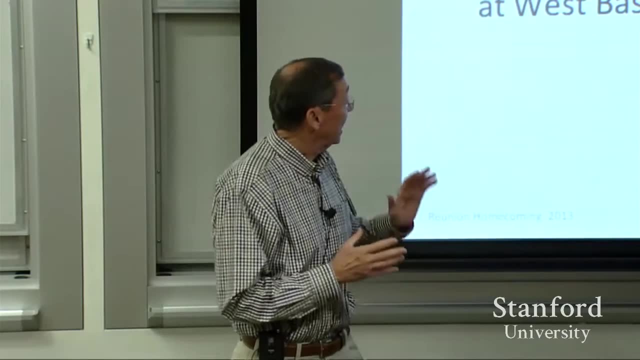 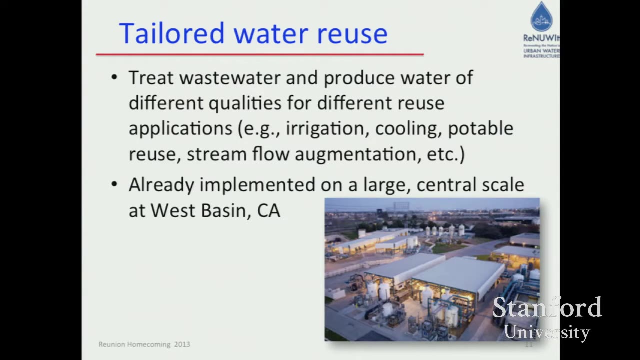 And for inspiration on this we can look down at a treatment facility that's south of the Los Angeles International Airport And at West Basin, if you go south of the LA airport, there's a big industrial area kind of along the coast there. 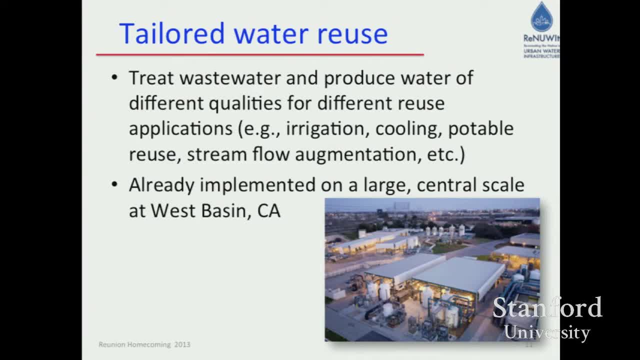 It's petroleum refineries and whatnot. But what they do there at that treatment plant is they produce waters of five different qualities, depending on if it's using for cooling, potable reuse, irrigation and whatnot. So it's possible to do this, but it's not. 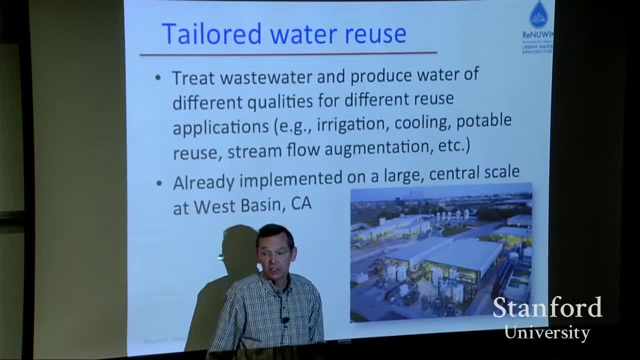 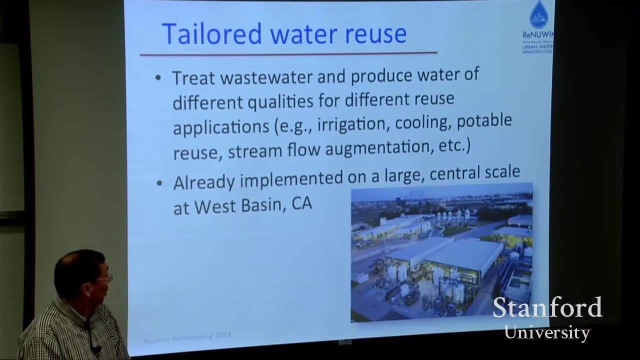 possible to extend this vision very far from what it is now today, because they've already exploited their customer base right there in that small district, in that sort of industrial area of LA, So we were thinking in the center here then. well, how do we produce waters of different quality? 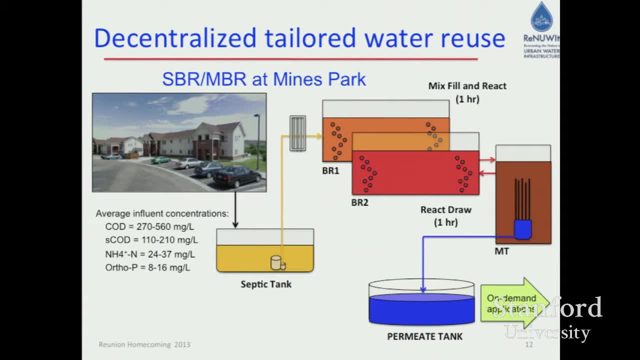 And what quality might we like? And this is a system that's being tested at Colorado School of Mines. It's basically a combination of membrane reactors and biological treatment systems that can produce water of different quality, And this water is largely of two quality. 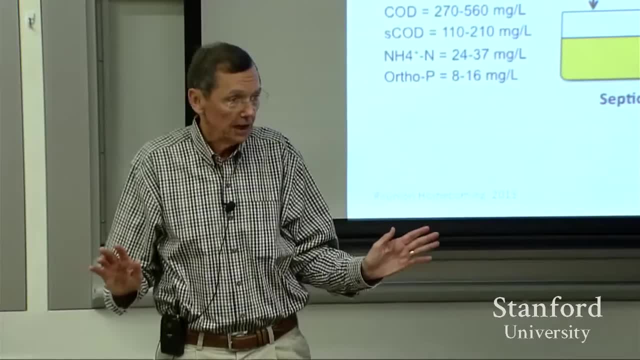 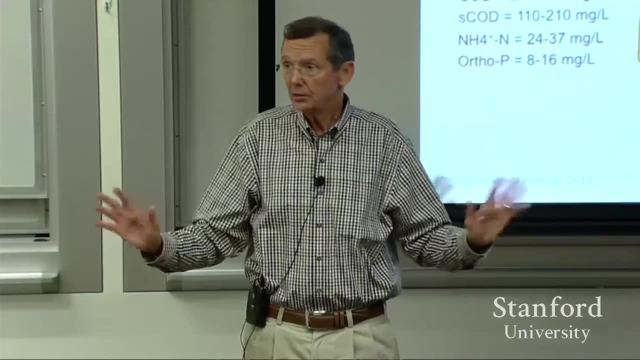 That's safe to come in contact with. but if you operate the system one way, you'll leave nitrogen and phosphorus in the water. If you operate another way, you take it out. Now what's about nitrogen and phosphorus? Well, these are nutrients. 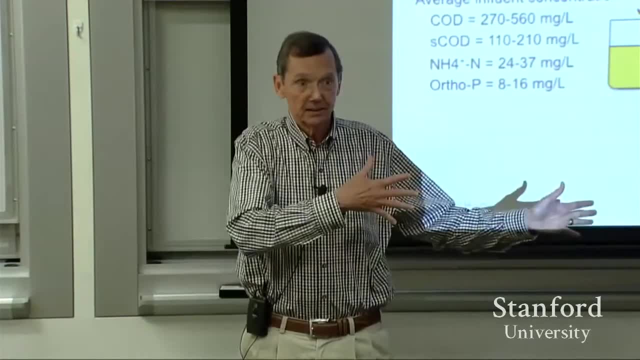 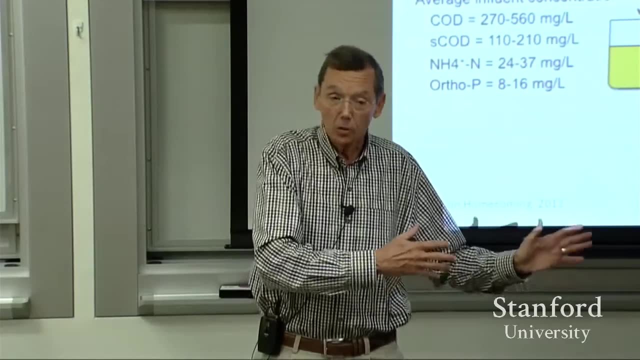 So if you're using water for irrigation, as you would in the summer, you might want to operate this plant to lead the nutrients in, because it'll supply a little bit of the nitrogen to the water, But in the wintertime, when the ground's frozen, 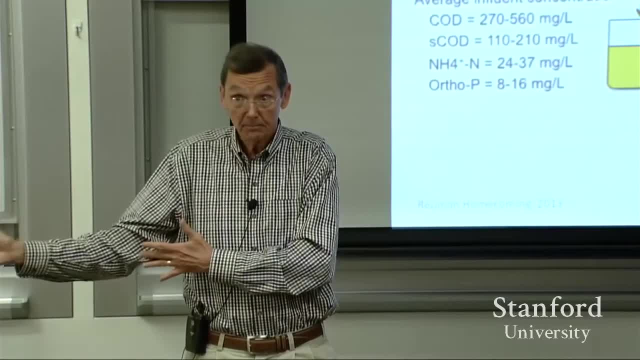 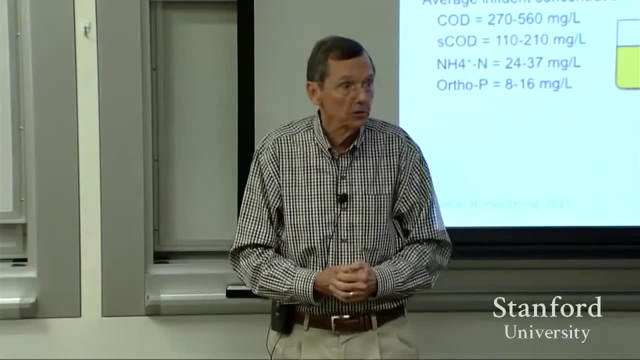 this water would go to a stream and you don't want to over-fertilize streams and rivers, So you take the nutrients out. Well, this idea of being able to switch back and forth between waters of two qualities: nutrient rich or nutrient poor- 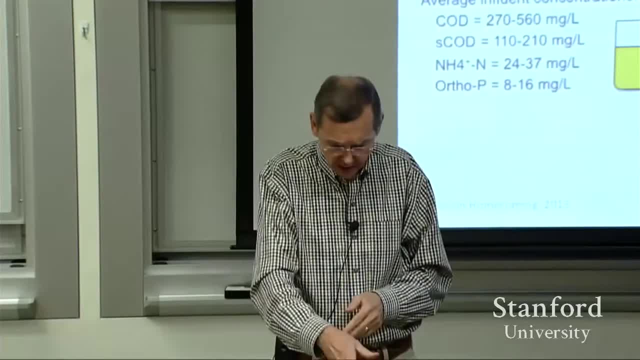 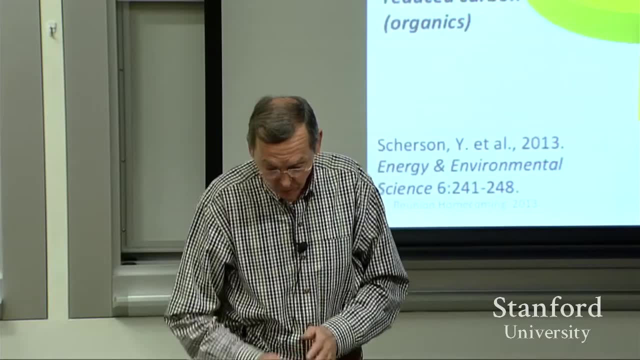 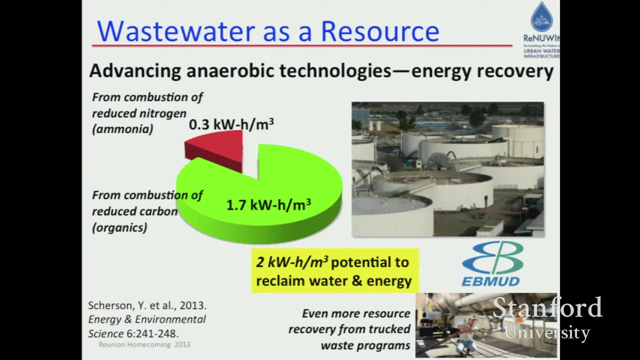 is an example of tailored water And that switch right. there is one that has a lot of implications to expand water reuse. The other one is I mentioned I mentioned nitrogen. I mentioned in that box of sort of four themes was the one of wastewater as a resource. 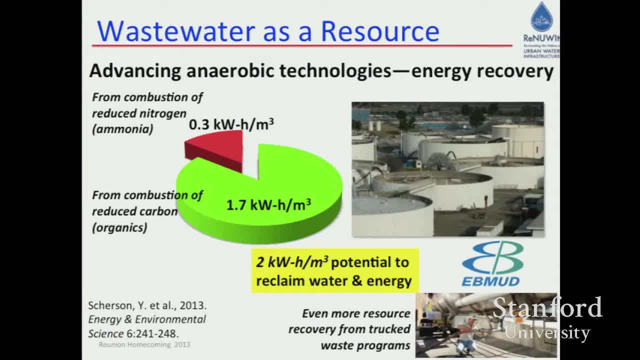 Wastewater contains organic matter. It contains nitrogen as well ammonia, And what we do today is we expend energy to treat that wastewater. But the wastewater itself, if you look at the chemical energy that's in there in terms of reduced carbon and reduced nitrogen. 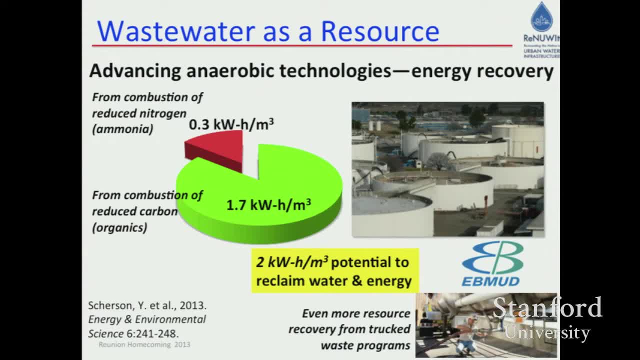 it has more than enough chemical potential energy to treat itself. But how do we do that? Well, we have to go to new kinds of systems. We need to go to anaerobic technologies. There's technologies that don't involve aeration. 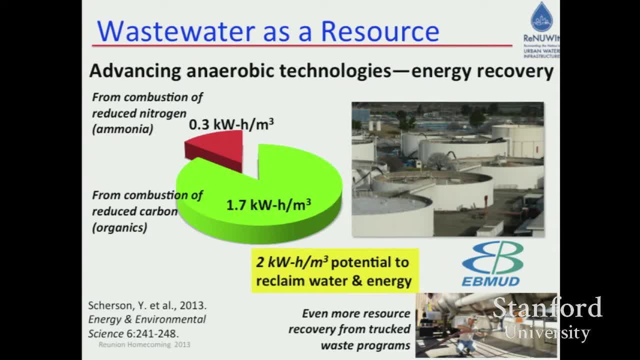 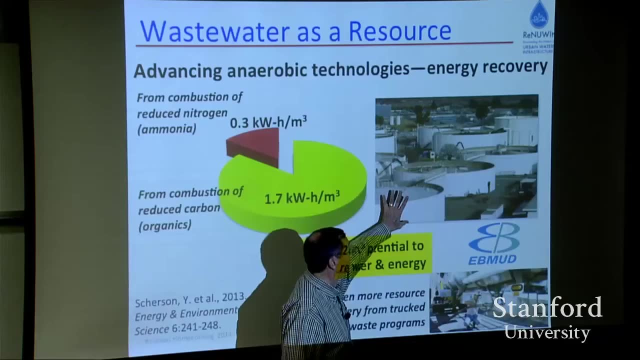 And capture all of this carbon as methane And then we can combust the methane, produce electricity and these plants can become energy positive. And that's a different mode of operation. But to take a big plant like East Bay Municipal Utility District and say, all right, let's get rid. 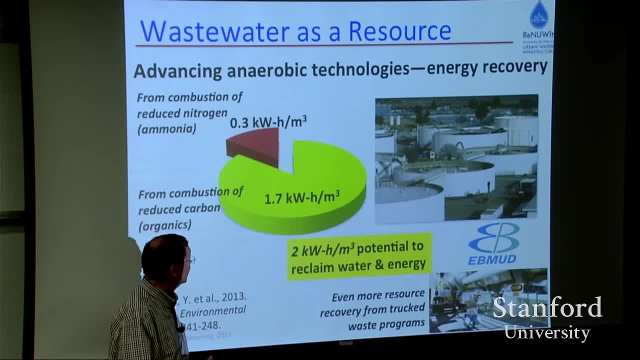 of all your aeration basins. We're going to go to this new idea. Well, we have to test these out at scale at some scale. And again, this is something we could test out at the Stanford modules that we would place over on the other corner of campus. 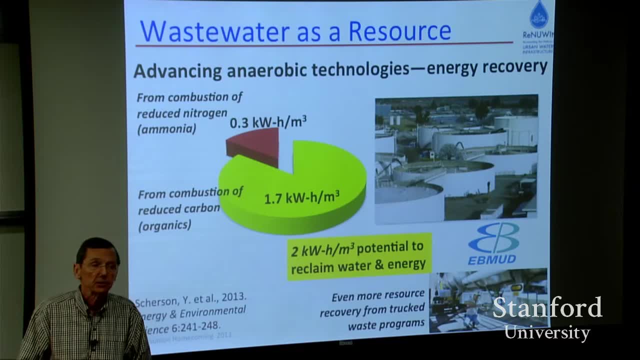 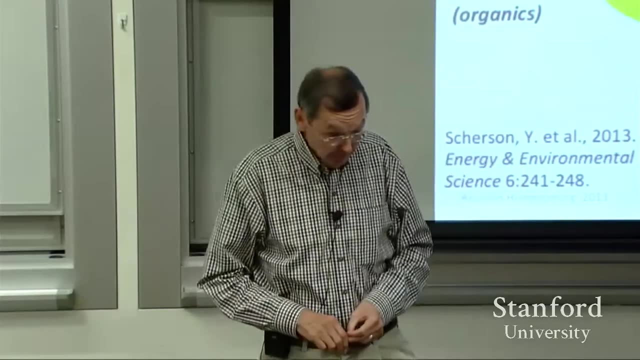 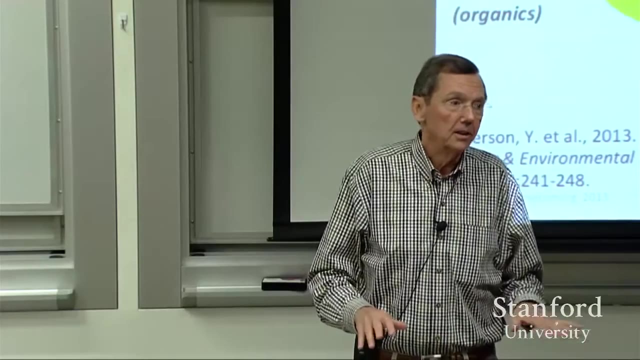 Another thing that's interesting here is to think about wastewater treatment plants of the future as resource recovery facilities. My folks moved to Palo Alto in December of 56. And at that time in the summer, in August, the bay lands would stink like you can't imagine the stink. 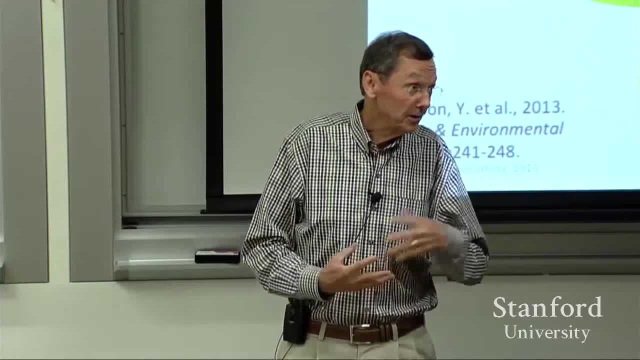 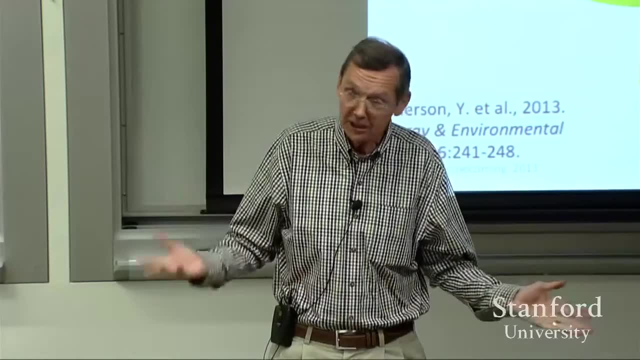 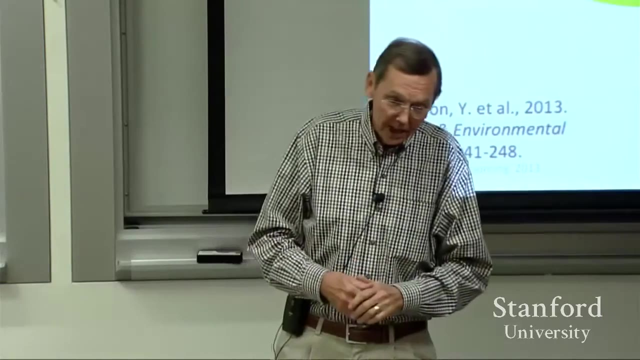 And where was it coming from? It was coming from San Jose and from all the canning operations that were done Down in San Jose. Now there are no canneries left there anymore. So with the canning facilities moving away and the upgrading, 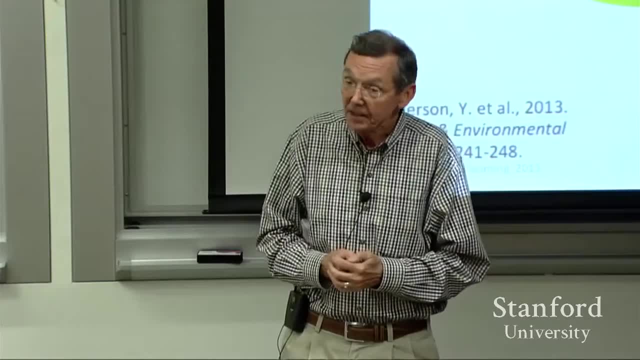 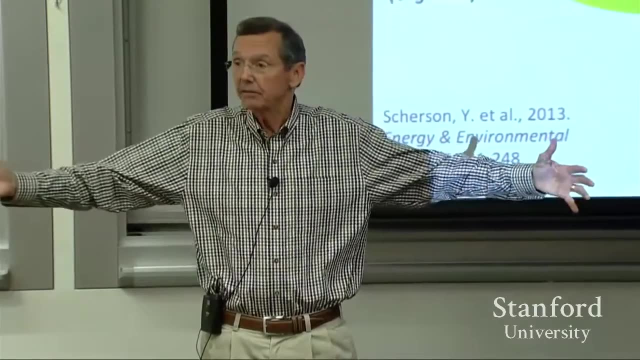 the treatment plants, we weren't discharging this waste to the bay. There used to be canneries in Oakland too, But they're not there anymore, But the plant was designed when they were expecting a lot of food processing waste to come to the plants. 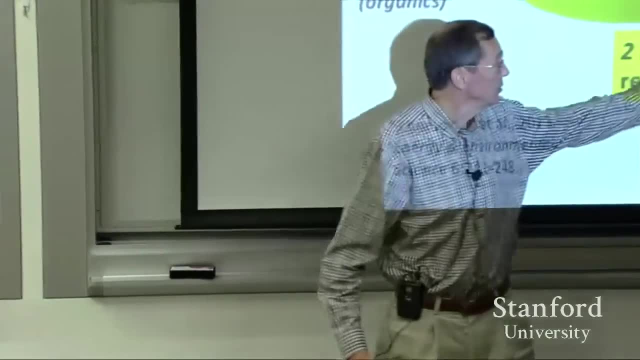 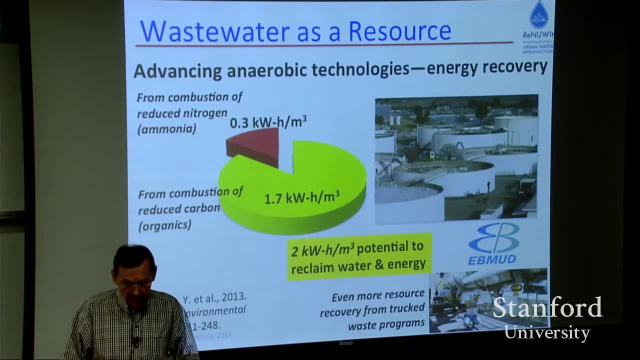 So in Oakland they happen to have excess capacity in these systems here That are called digesters. So what they've done at East Bay Municipal Utility District is to rethink one part of their operations, And that's this part that deals with all the waste sludges. 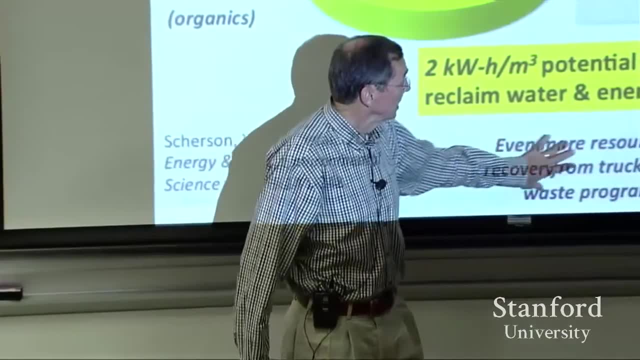 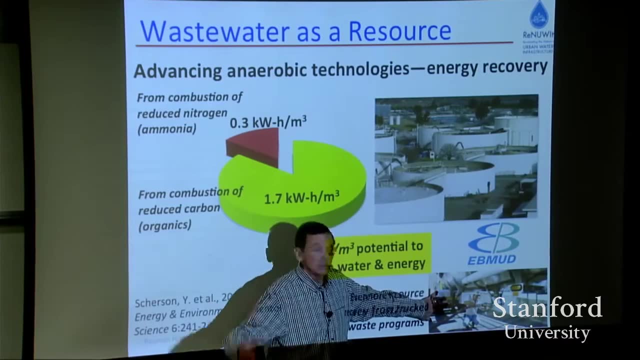 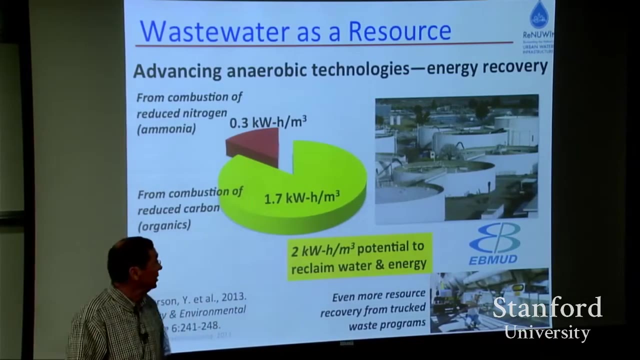 And have instituted a program to bring in trucked food waste from Napa and the Central Valley, like chicken blood or whatever, And then process through these digesters And convert that carbonaceous material of methane And then combust that And that's a successful program. 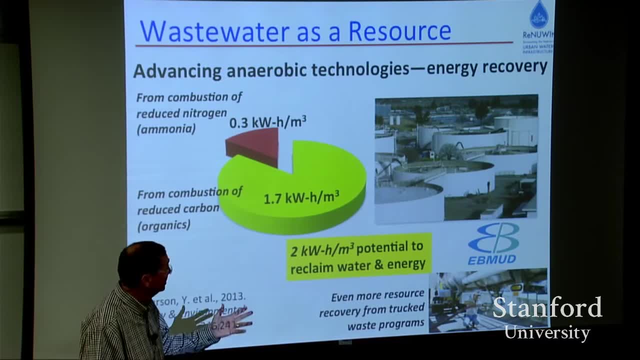 And now East Bay Municipal Utility District's plant is really the first energy positive plant wastewater treatment plant in the country, And they're able to do this because of the trucked waste program. So for us in our center here, what we're studying- 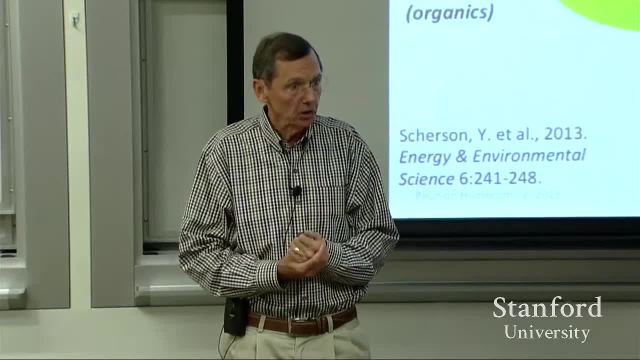 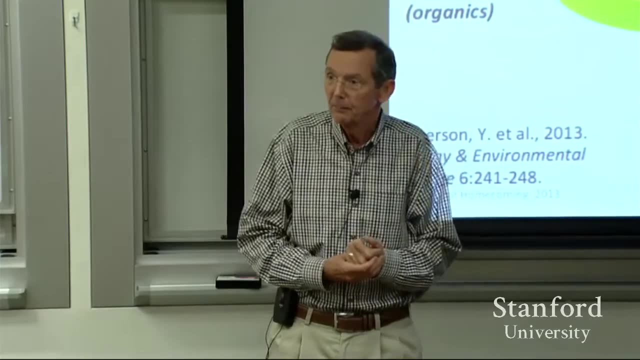 Are these anaerobic technologies how they'll really work? And then also the business model of the trucked waste. I mean, what if Napa decides? you know this looks like a good deal. Why don't we, instead of having the trucks run down to Oakland? 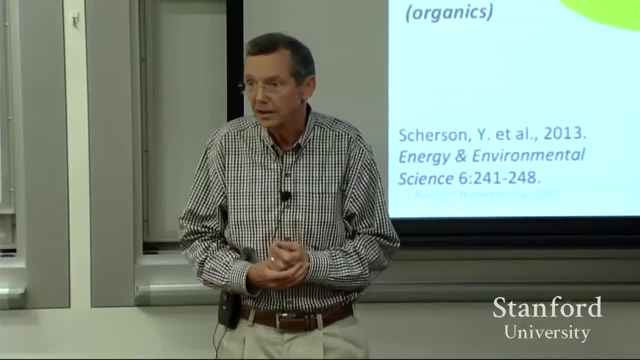 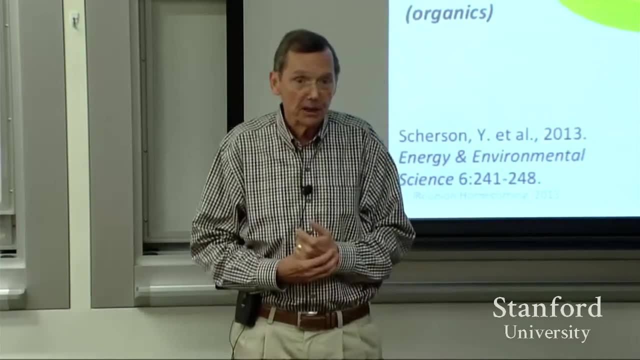 Why don't we? why don't we do this ourself? Or what if Modesto decides? you know, this is a great idea. We can just do that too. How many of these facilities could you support around the bay? Well, those are the kinds of sort of systems level questions that 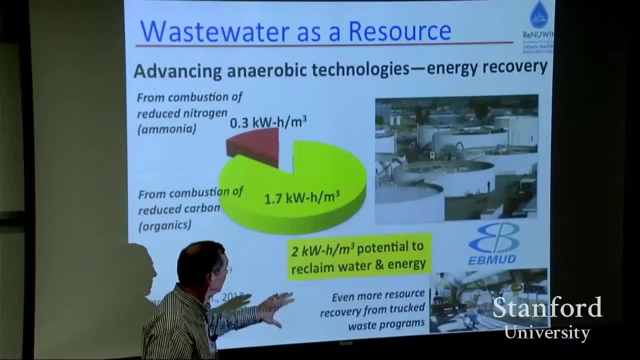 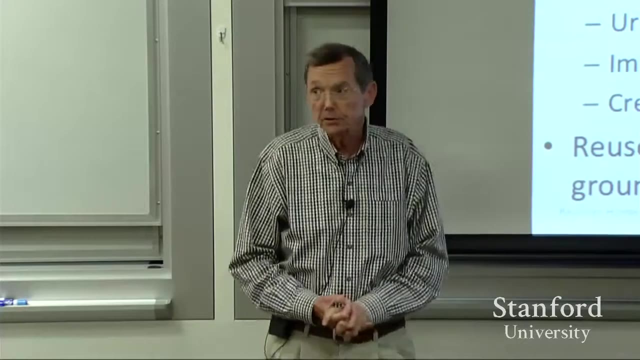 that come to mind About expanding this, And so there's sort of a business finance issues here And there are these technological issues about how you really make these plants work reliably. The other box that I mentioned at the start of the talk was broadening the treatment options. 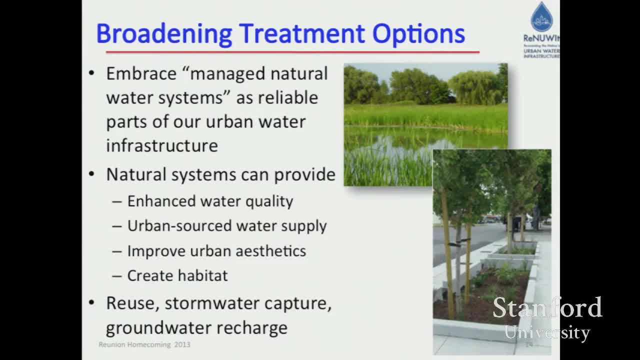 And here we might think of how can we use natural systems to treat our water, And natural systems you can think of as wetlands or maybe these bio infiltration basins like this And you've all seen these Along curbsides and the like. 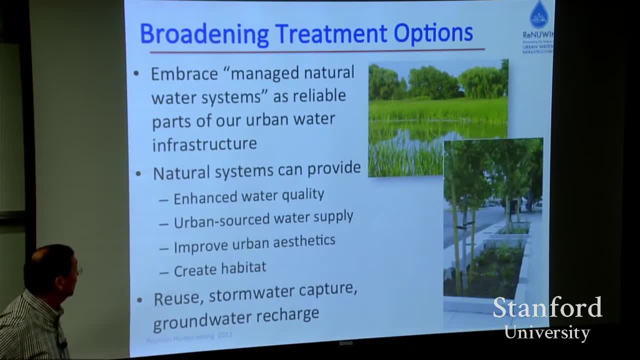 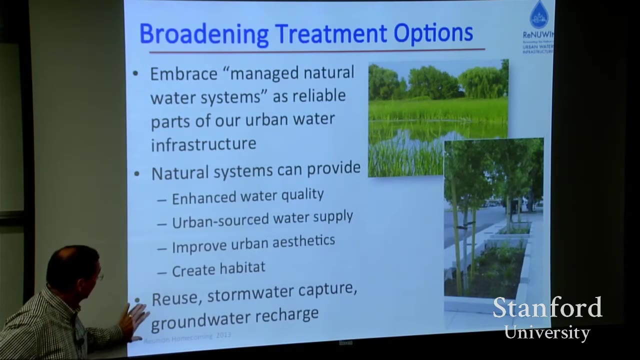 Well, we, we believe natural systems can improve our water quality. They can be a source of local water for us. Obviously, they improve the urban aesthetics and they create habitat. So when we think about reuse and storm water capture and recharge of ground water, there's a big role here for natural systems to play a role. 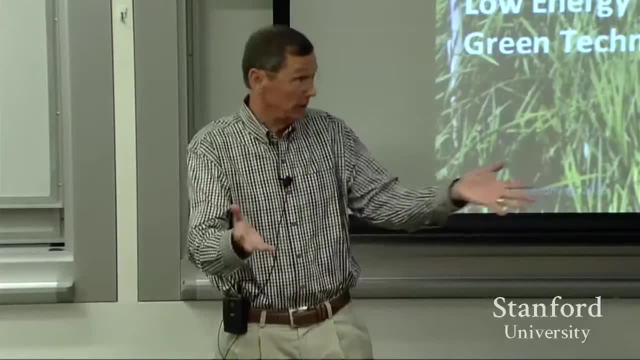 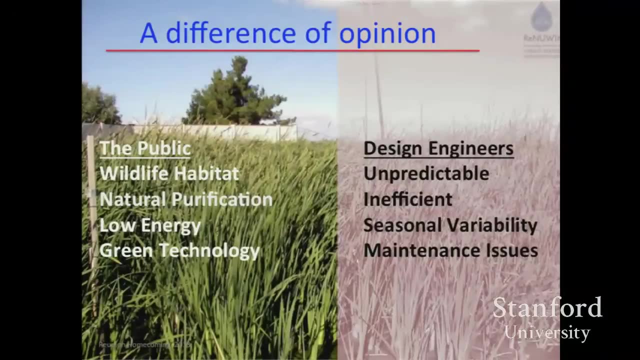 These natural systems. I would think you all have seen wetlands and marshes and grassy areas And you think, gee, that's, there's a peel. Do you like the wildlife habitat, The purification, the low energy, the green? 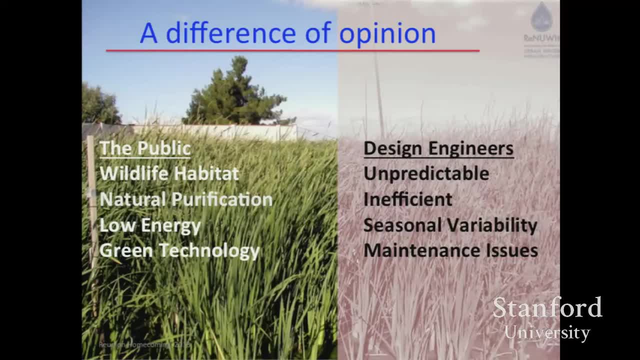 But you know, engineers look at this and maybe plant operators look at these and say: you know, these natural systems are unpredictable. They may be inefficient if it gets cold. There's some seasonal variability. I really don't know how to manage, to optimize or change performance. 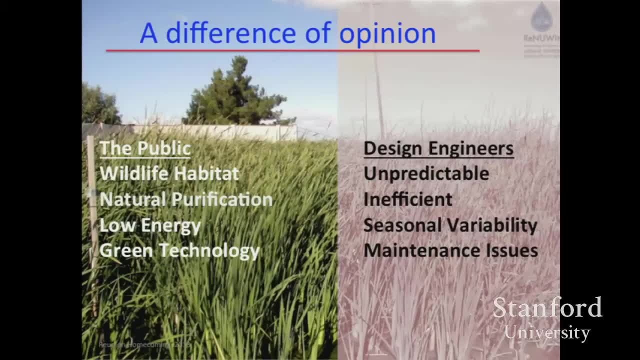 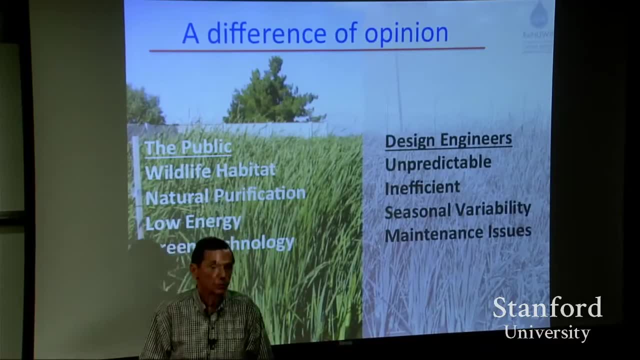 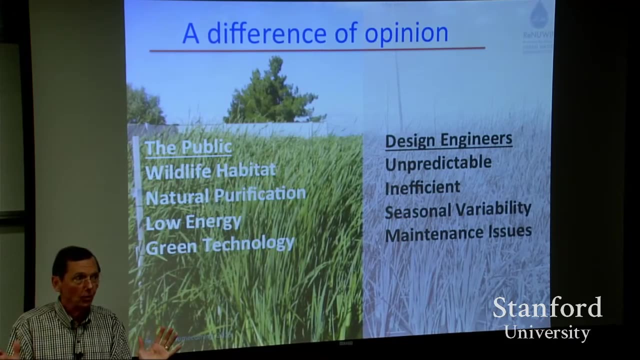 These are issues that we're addressing in our center- is: how can we better invoke natural systems as part of our urban water infrastructure? Now, where might this go? Well, let's look at the issue of storm water capture. You all know storm water. 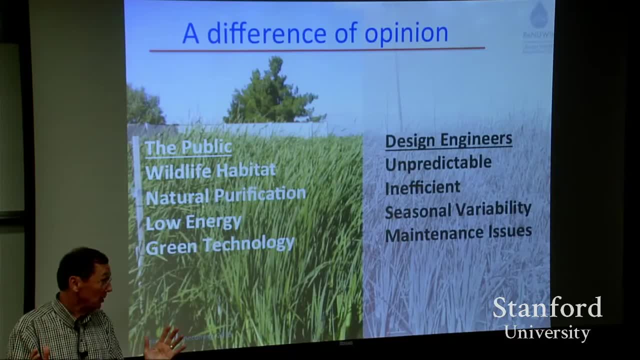 You know what happens around here with all our storm water. We just collect it up and push it to the bay as fast as we can And you, you know all the curbs that say, you know, don't throw the water over it. 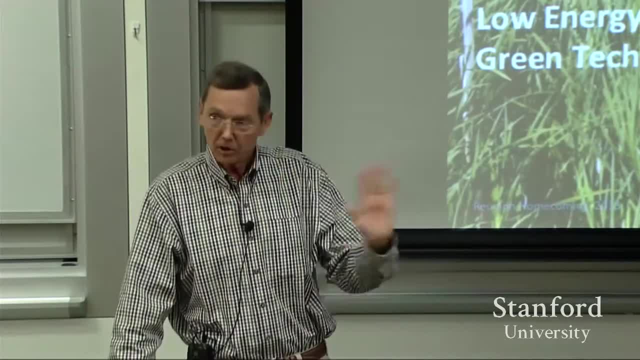 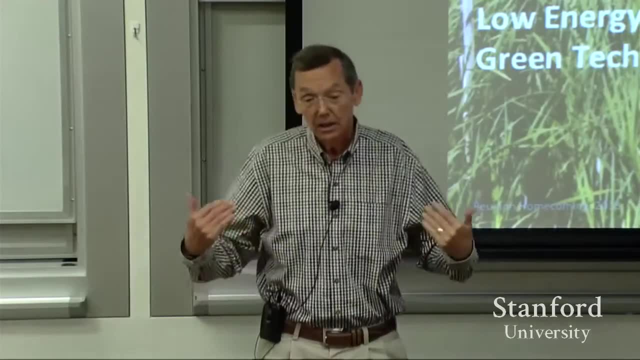 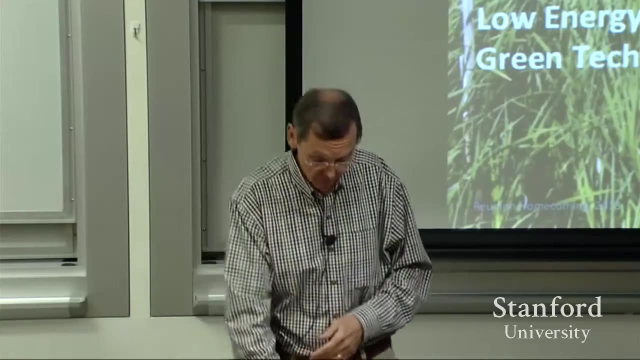 of the waste here flows to bay. So all the big cities kind of like from the California coast. here the mentality was quickly collect that storm water and shove it to the ocean or a bay and get rid of it. Now we see it as a resource for the future. 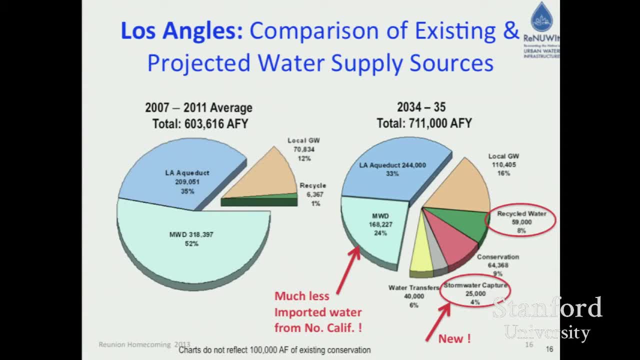 So this is another pie chart. The last pie chart I'll show is where the city of LA sees them getting their water for the future. This is where they are today and that's where they want to go tomorrow, And so there are two pie charts. 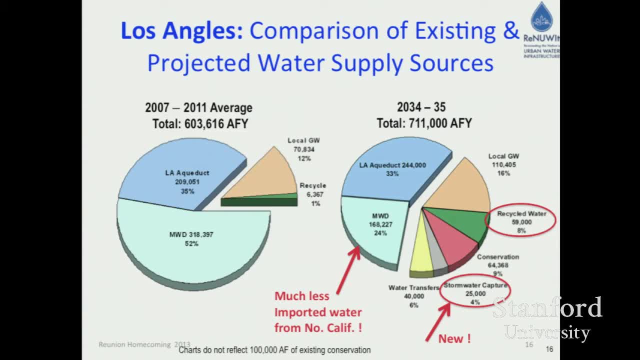 But this doesn't look like much of a pie chart because there's one big, huge piece here, And this is the piece, that's water imported from Northern California in the Colorado River And the plan for the future 20 years out. 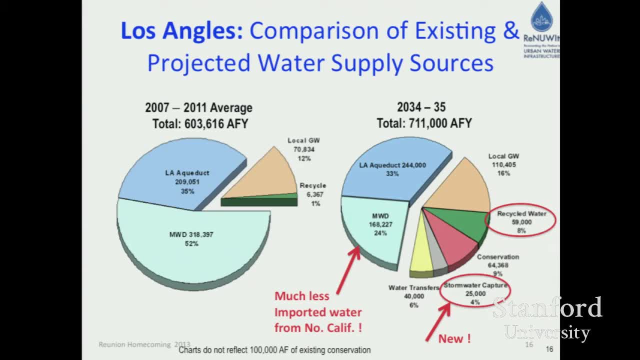 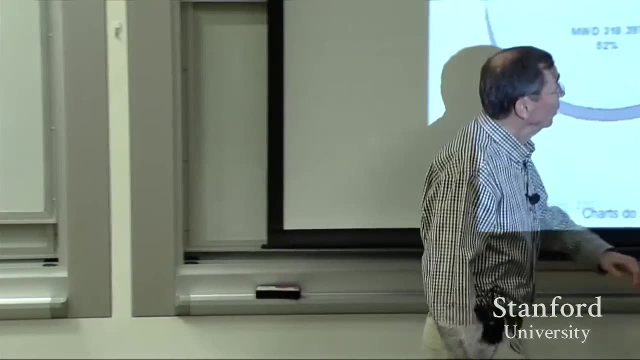 is, even with increase in population, the absolute amount of water that they're going to import is going to be less, And this is a trend for the future: Less reliance on imported water. And so how do you make up this difference? Well, recycled water plays a big role. 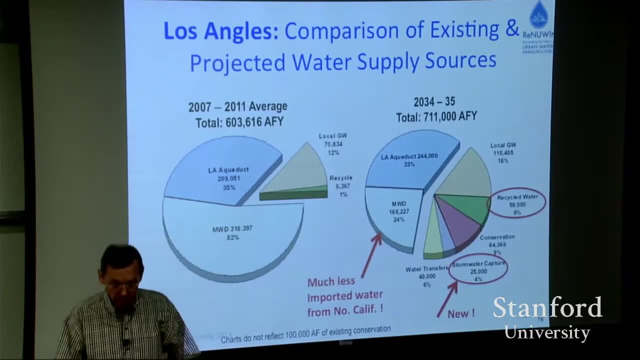 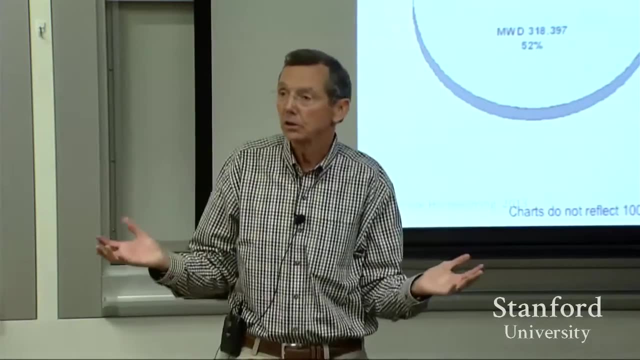 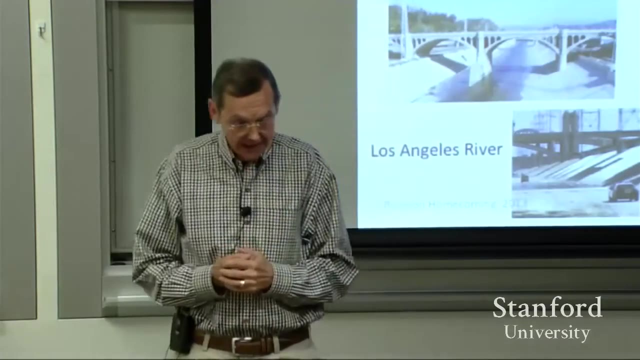 And storm water capture now plays a big role. I mean, storm water wasn't even on this side of the picture, So how does storm water capture really work? How would it work in LA? Well, we live in a Mediterranean climate, And what does that mean? 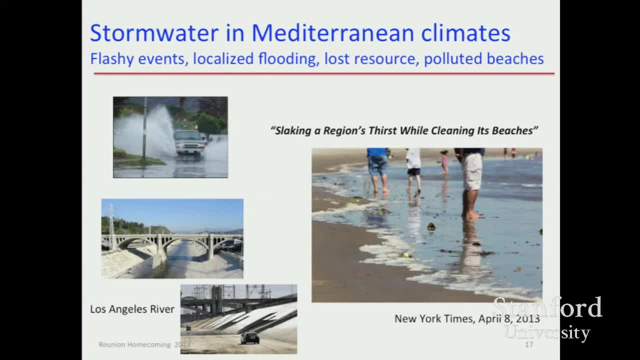 That means we get these heavy rainstorms in the winter and then it doesn't rain for six months or something like that or whatever. You know, we're still in our dry season. So we have a challenge here of sort of balancing out the time when we have water and the time when we need it. 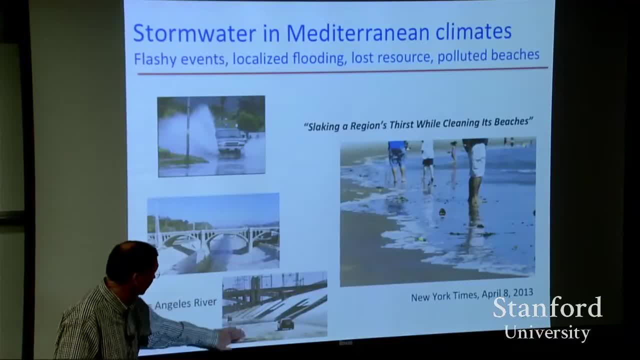 Our approach to these flashy storms was to build these things that you see in Hollywood movies. You know the chase scenes in Terminator or something. And then another problem here is that you get these big surges, that kind of flush the city and you end up with contaminated beaches. 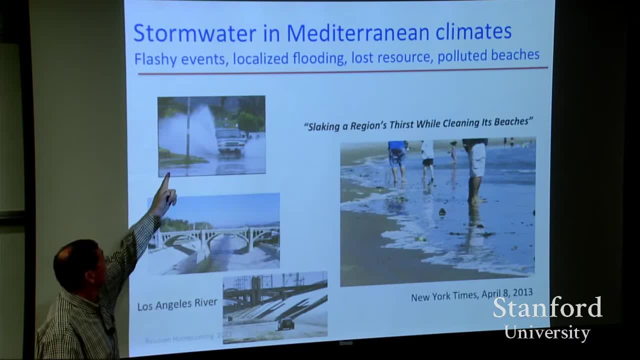 And there's some parts of the city north of the Burbank airport that don't even have storm sewers. So that's where we are here. So we say, well, how can we think of a new way of sort of managing these flashy systems? 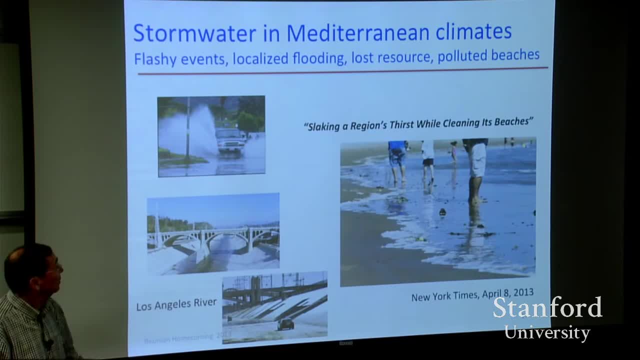 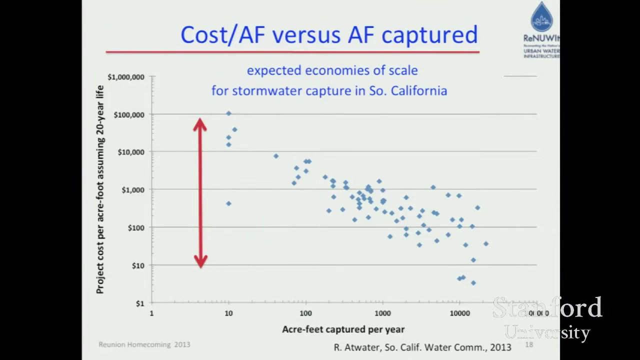 manage the localized flooding, save this water before it goes to the ocean and, at the same time, prevent the pollution of beaches. Now, that's the idea. Well, how big would these systems have to be to make a difference? Well, this shows the cost per acre foot of water captured. 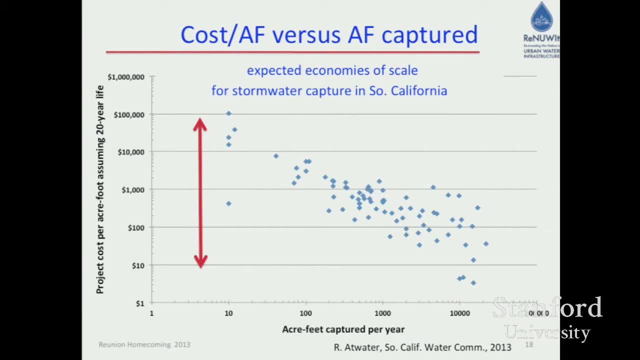 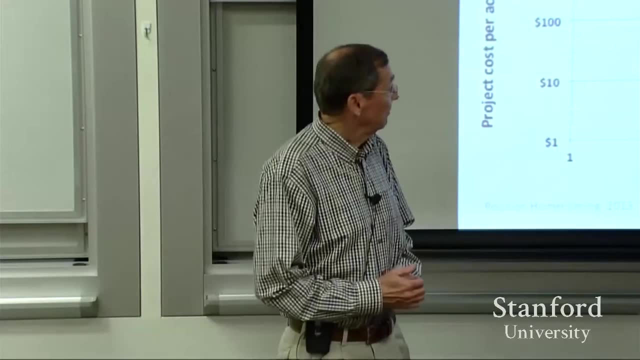 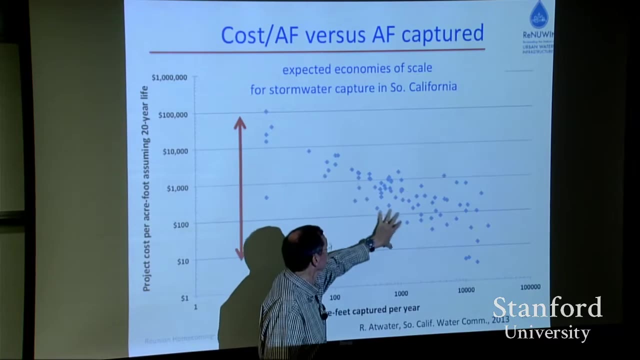 versus the acre feet captured. In other words, you say Cost per gallon versus number of gallons, And an acre foot is about a third of a million gallons. The point here is you can see how these are both log scales. So to be efficient here we need a big system. 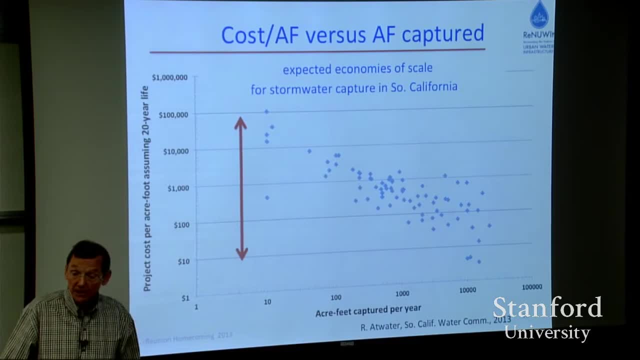 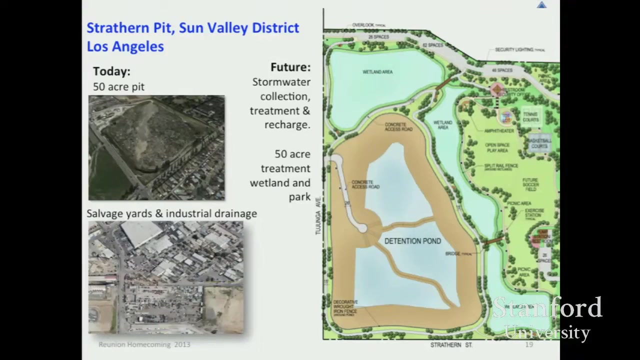 We need something that will capture about 1,000 acre feet a year And that becomes an efficient size. Well, where might we try to go? We try this out And we're working with the city of Los Angeles. well, the LA Department of Water and Power. 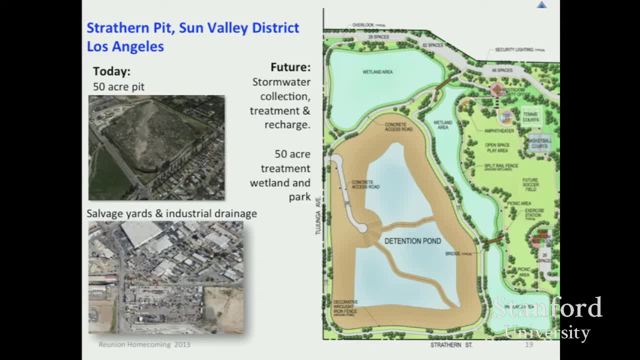 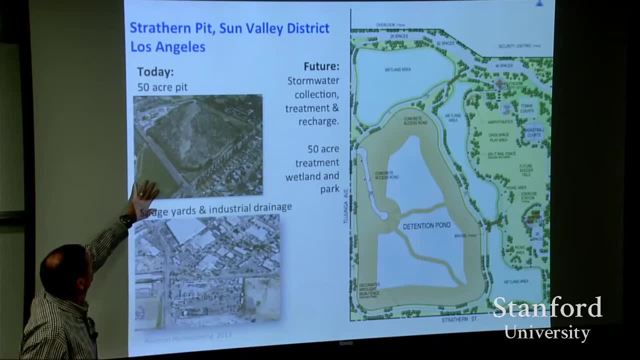 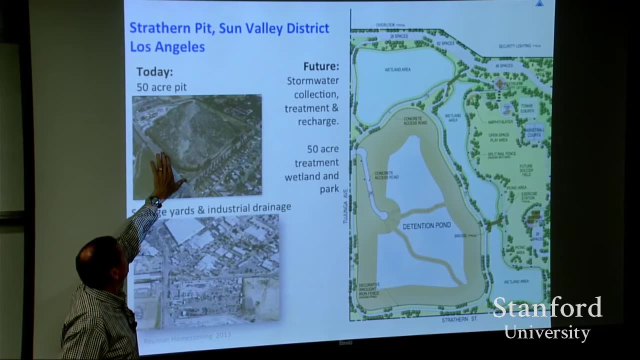 and the Bureau of Sanitation and Public Works to look at a field site north of the Burbank Airport which is a current old gravel pit and a little bit of a dump for construction debris, and converting that And then we can use that to a system that would collect storm. 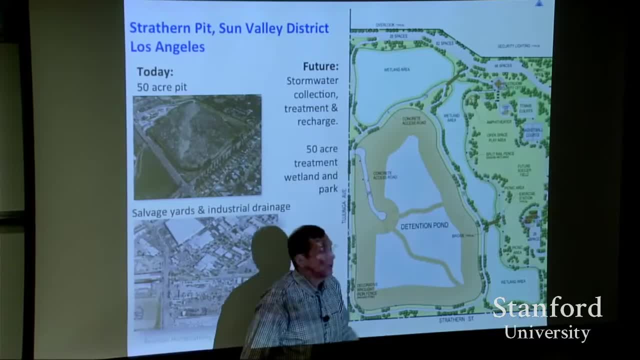 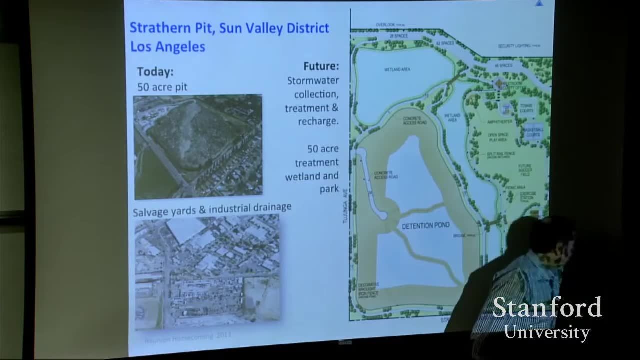 water, hold it for a while, then process it through this wetland and thereby purify the water. We might have to put a few more steps here And then pump it about that far into the ground and it becomes part of the water supply. 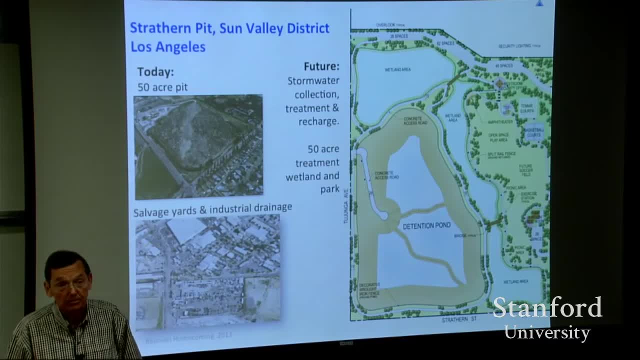 for the city of Los Angeles. Now, that's the picture. This is the artist's picture. I have other ones that make this look like it's just this little isolated thing out in the green space. But there's a lot of other things that we can do. 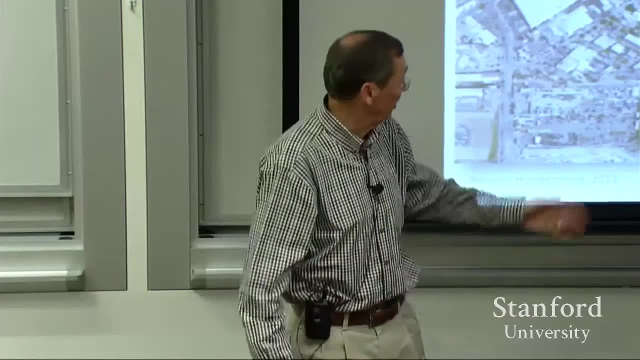 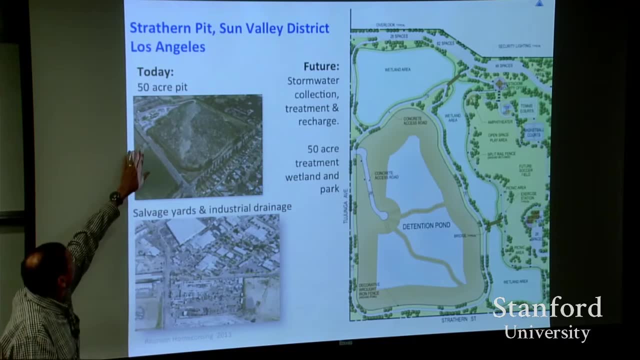 We can take this out into the green space. The reality is, though, this is the area in which it sits- A lot of automobile recycling and industrial activity just off the edge of the picture here, So when we think about storm water capture, we need a big spot. 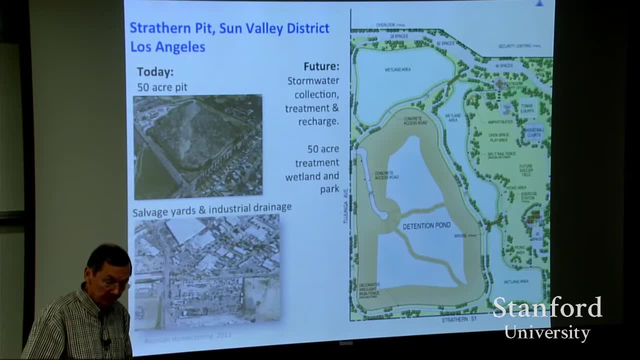 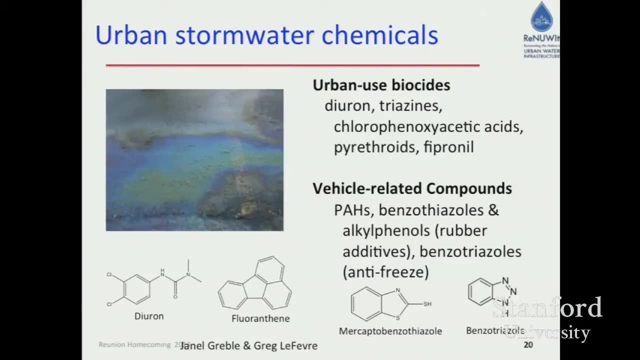 And you can repurpose some of these sorts of places, But you also need to be aware that storm water is not clean. obviously It contains biocides, You know, that are used for weed control, and that kind of things. It has vehicle-related contaminants, oils and stuff like that. 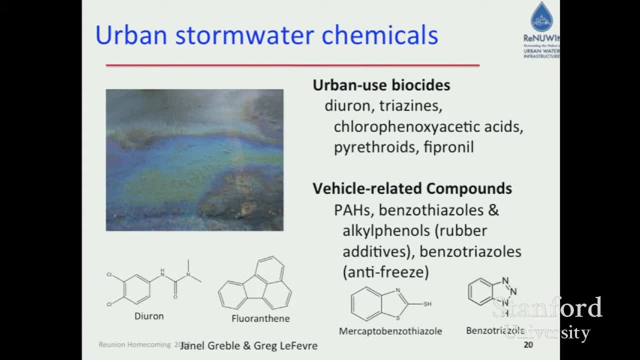 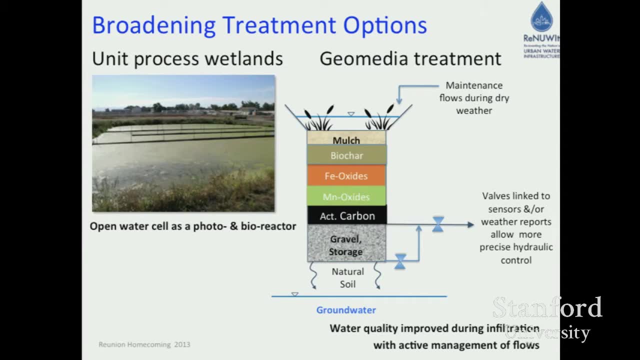 additives to tires, ingredients in antifreeze- All of this is in our storm water. So the challenge for us, then, is to think about: how do these, How might that wetland system really work in removing those kinds of contaminants? So the challenge for us, then, is to think about how do these? How might that wetland system really work in removing those kinds of contaminants? 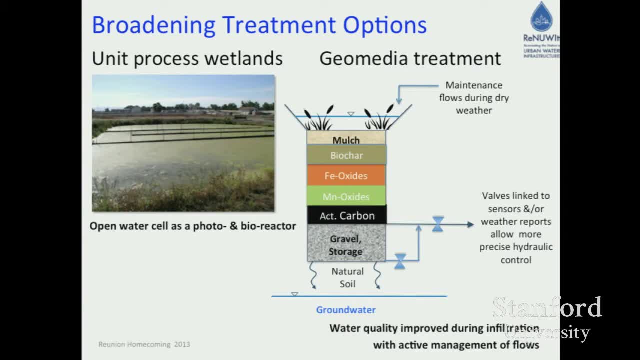 And these are not Those ones I just had on the previous slide, are not the normal thing you find in wastewater. This is storm water, And so what we're looking at here is a combination of both natural systems, like a cell here that would be open. 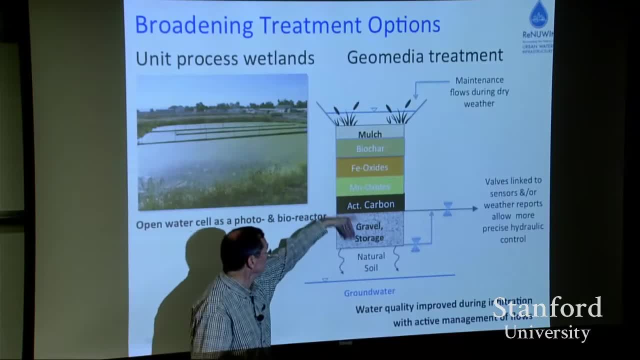 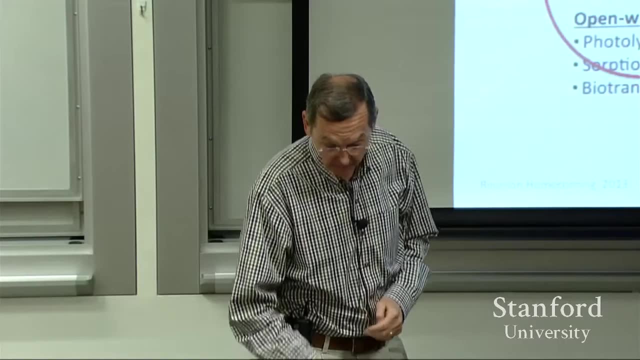 and a system like this that might have an infiltration system with different media to remove the last little bit of contaminants. So the idea is that we are imagining. So the idea is that we are imagining. So the idea is that we are imagining that we can do a better job. 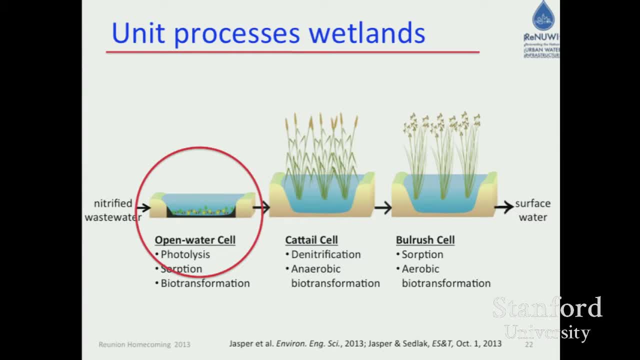 of designing and operating these wetland systems, And here I show a picture of a wetland system that really doesn't have any plants in it, at least emergent plants. It's a very shallow system, about a foot and a half deep. 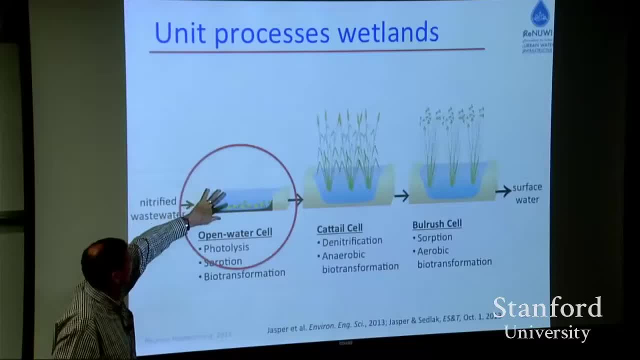 And the idea here is to promote reaction with sunlight- That's called photolysis- And then in this system you'd be growing a little bit of algae and there'd be some bacteria there. So there's a combination of physiochemical transformation here. 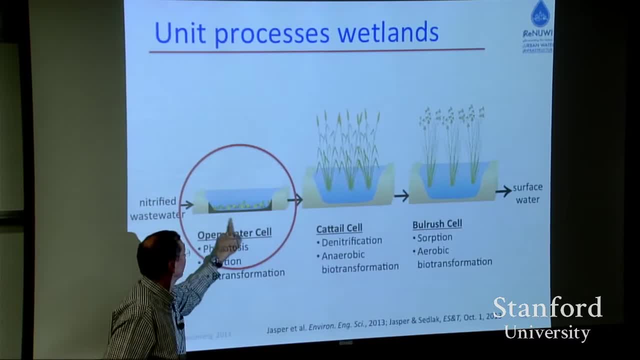 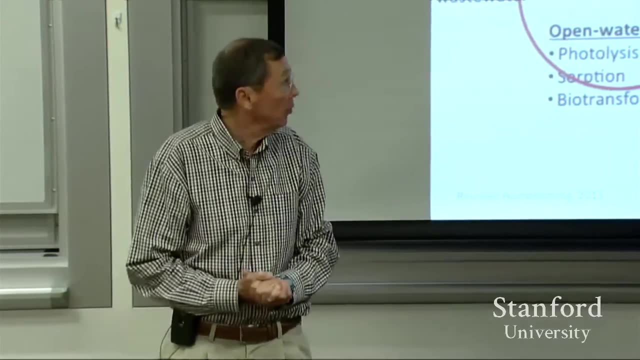 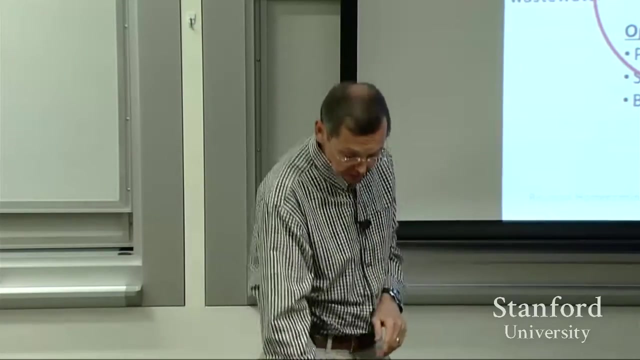 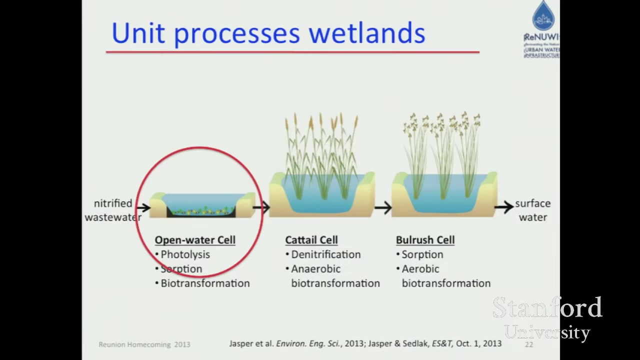 by reaction with sunlight and then bacterial reactions here in this bottom little layer that would form in that cell. And we've tested these ideas out at that picture I just showed earlier at this small plant up here in Discovery Bay. But they're all questions about how does this really scale up? 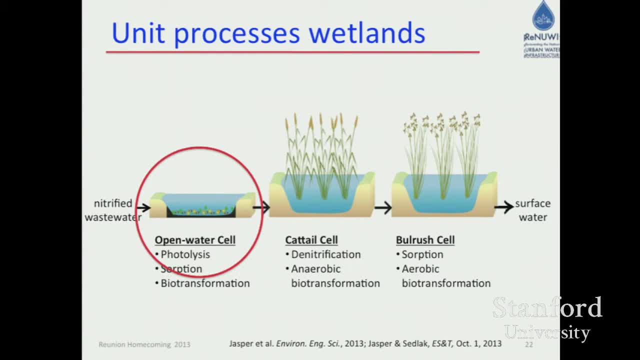 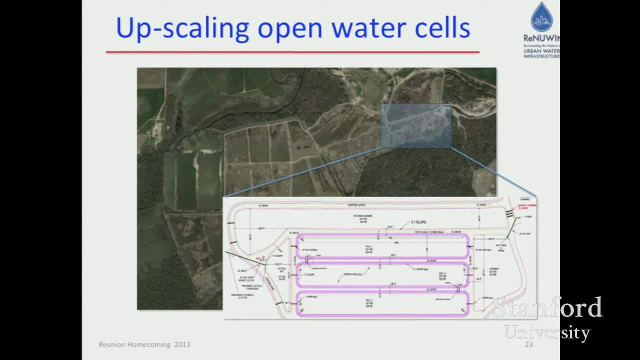 and will it be reliable at big scale? And for that we are working with Orange County Water District, and they have just built for our testing a set of three parallel cells that are 100 feet wide each and 800 feet long. And so this is, I guess you'd almost. 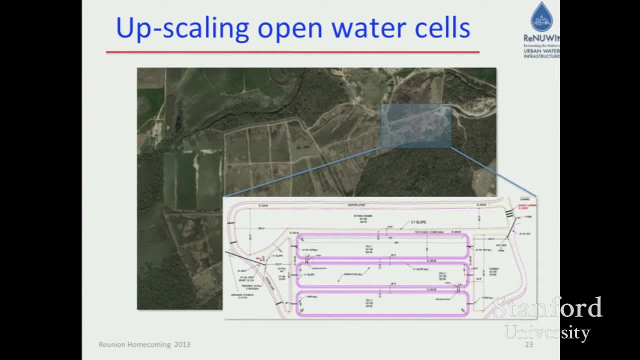 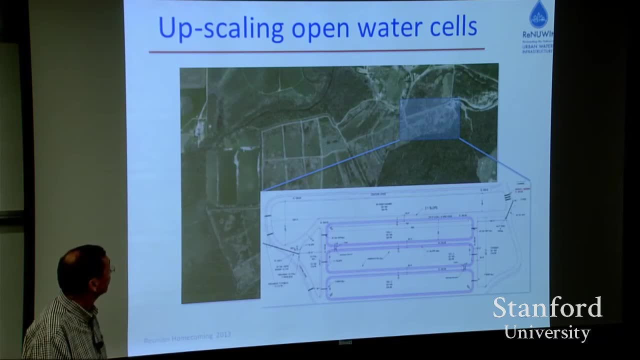 I'd call this a full-scale system, But we have these three parallel trains here, or we could make it be serpentine back and forth. That system is built and our experimentation will begin later this year on addressing questions of both sort of a biogeochemical nature. 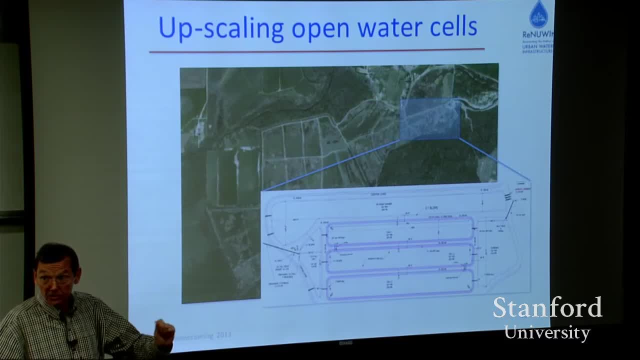 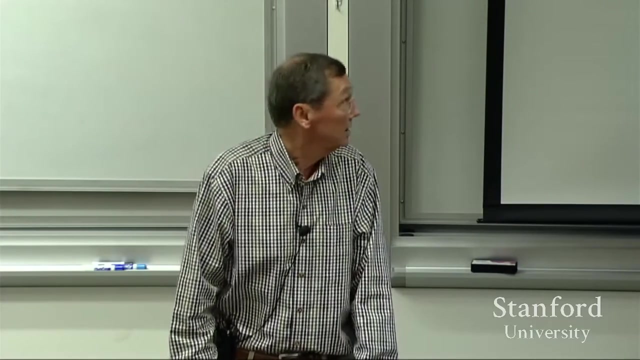 and a control. How do we actually sense and control these facilities? So I guess I go a little bit off script here a little bit. You know this shows the value that this water district has placed in our ideas here. When you look at 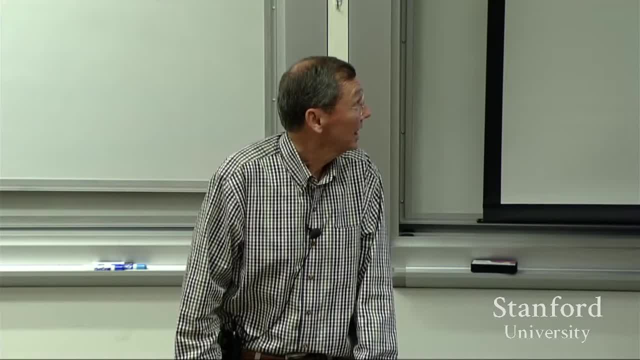 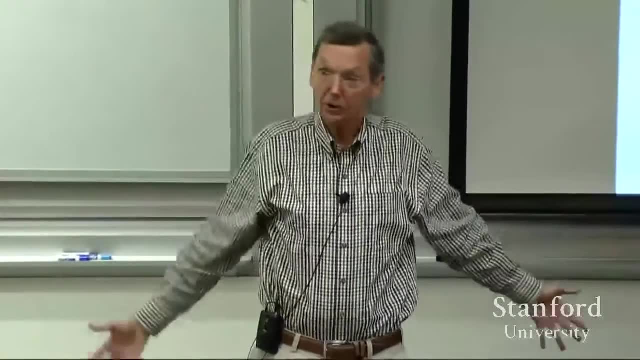 I have another picture that Maybe I should use that on Friday. It shows a truck out there and you can't see the truck. I mean, you can tell this is a dump truck and this thing is huge. So anyway, this is right by the Santa Ana River. 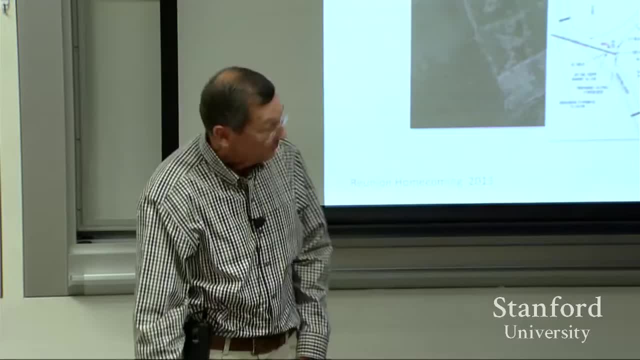 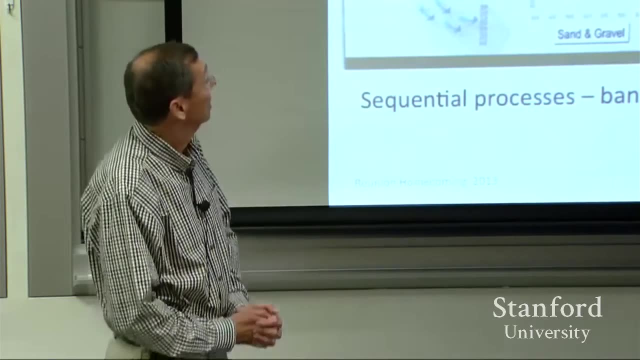 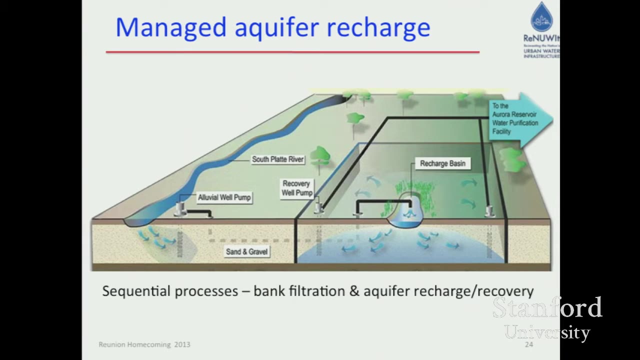 and this will be our experimental facility to look at how to upscale these new ideas in wetland treatment systems. Another area in which we're working is out near Denver, sort of northwest of the Denver Airport. This is the South Platte River that flows out of Denver. 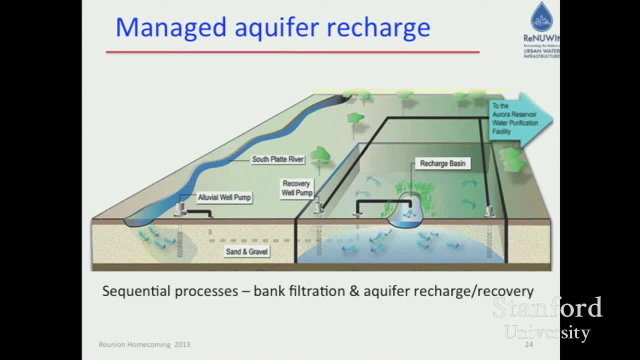 and the South Platte River in the summertime. much of the year is basically wastewater from Denver. I mean it's been treated, but it's what's referred to as an effluent-dominated river. With some water transactions, there was an opportunity. 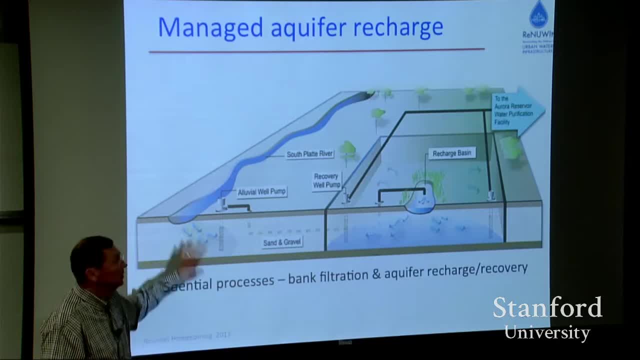 There was an opportunity for the city of Aurora to take some of this water and pump it to meet their water needs, And what they've set up here and what we've studied and investigated over the last several years, is how this system works in terms of this pumping of the water from the river. 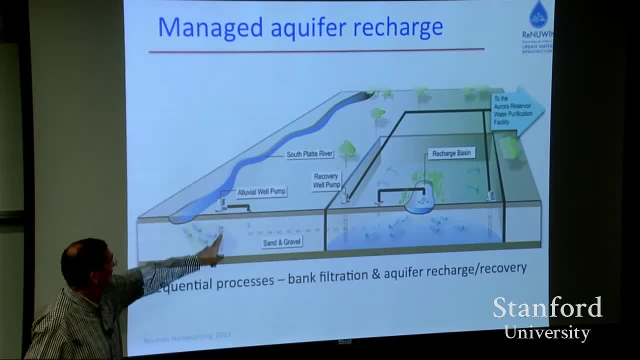 Now, you don't pump it from the river directly. You pump it from this well that's adjacent to the river, So you get a little bit. It's called bank filtration. You get a little bit of filtration, but you don't pump it to the earth here. 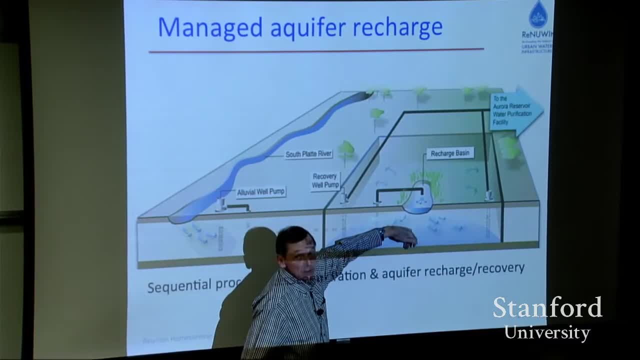 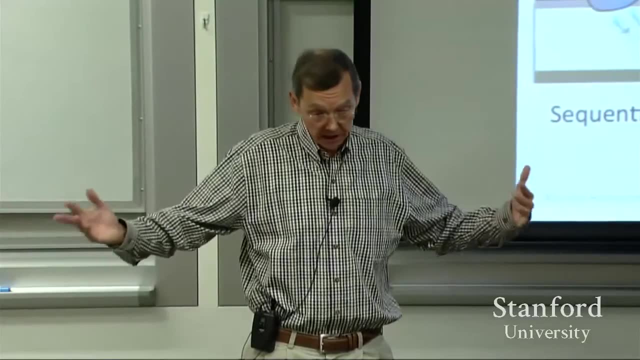 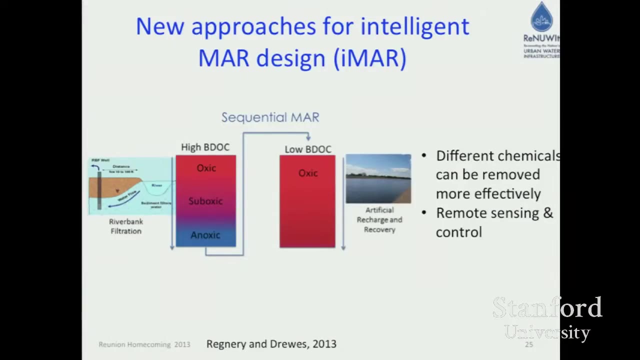 That water then goes into this recharge basin, stays in there for a while and is pumped out and then goes to the city. So it's a combination of a bank filtration and this recharge basin, And this leads to a new idea that we've been able to show. 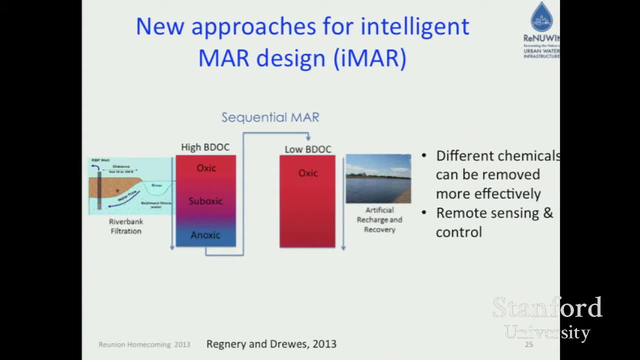 about how different reactions are occurring in each parts of the system to remove contaminants. When you pump the water through the ground or into the ground and then you're going to pump it out again, it comes with a little bit of contaminants. They're more degradable. 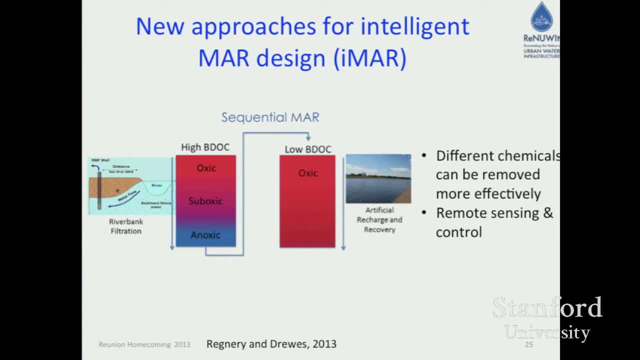 They deplete the oxygen in the water. So in this first step here you get a consortium of microbes that can live on, sort of the easily degraded substances that are in that water, and then they begin to deplete the oxygen. You pump that over into this. 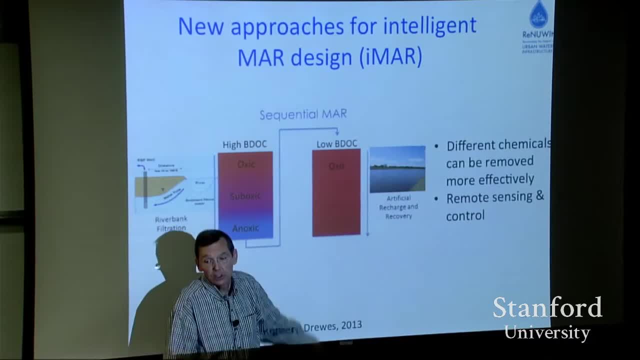 There's a picture of the Aurora recharge basin. You pump it over here and you get a different flora of microbes. And what happens there now is the easily degraded carbon is gone. It's an oxy system and you get a whole different flora of microbes. 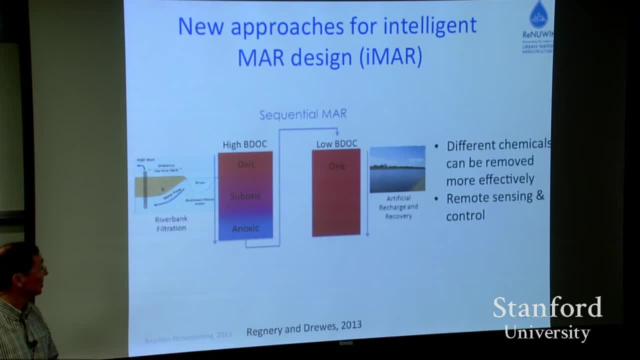 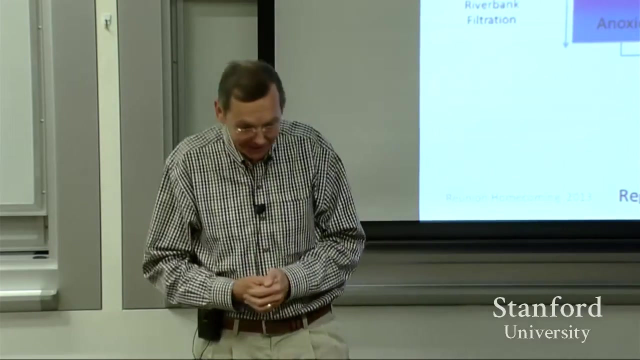 The two together really remove the trace contaminants with a high degree of efficiency. So we call this managed aquifer recharge, or because we're at Stanford, I guess we like to put an I before everything. I might call it I M-A-R. 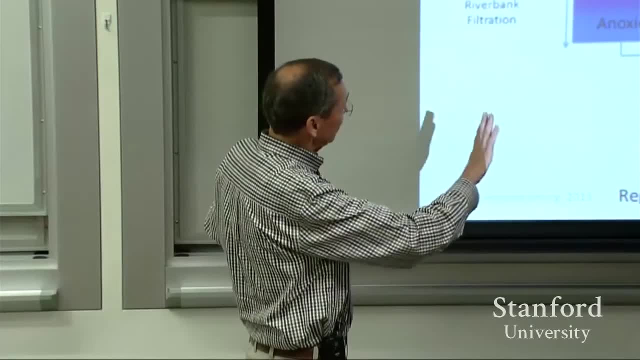 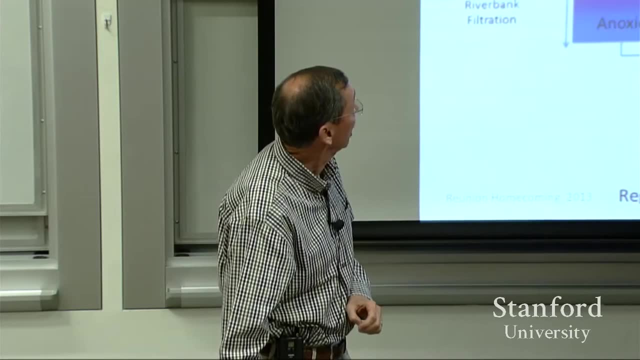 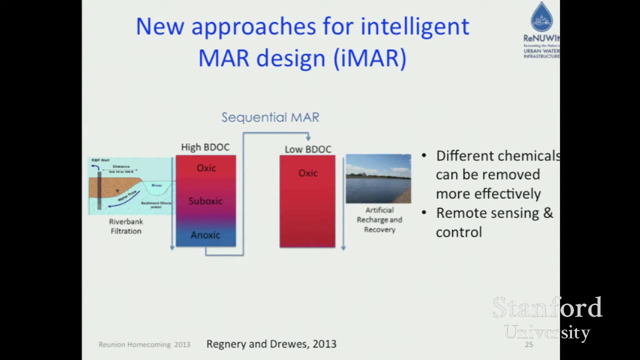 But that's a This understanding, these Working together these two systems has led to better understanding of how we can recharge groundwater in ways in which it can become part of our urban water supply, but do it in ways that are safely Or that are safe. 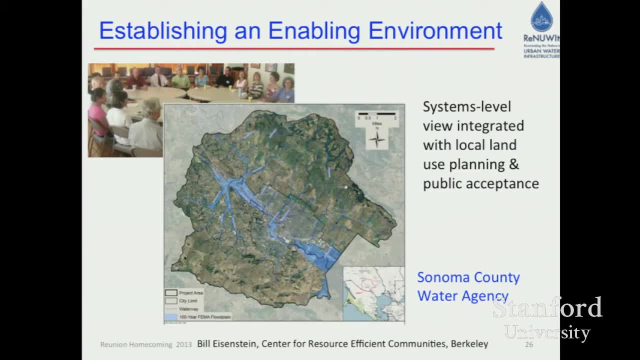 And then, lastly, the last box I talked about was the one of establishing the enabling environment. I mean, how do you do systems-level thinking? You know what's the Why should I do stormwater versus water recycle, Or why do I need to do either of those? 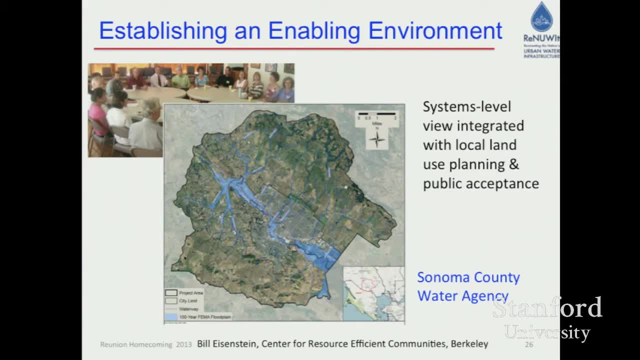 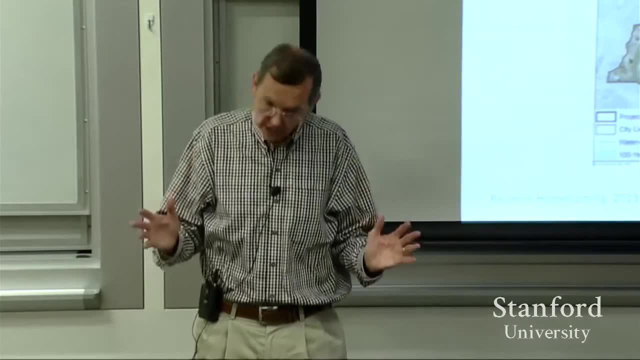 Can't I just buy someone else's water, You know, say, when you think about your urban water supply. Well, for this there's no straight answer. There's no one answer for every place. There are clearly regional and political realities. 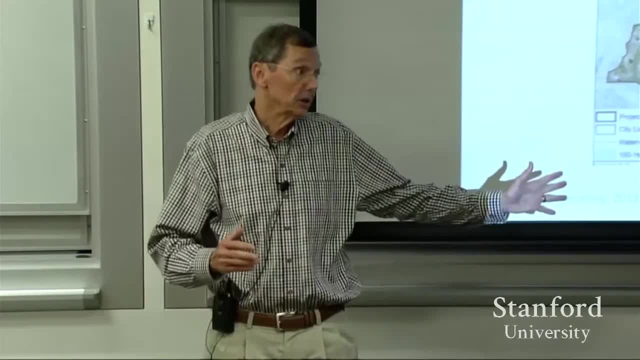 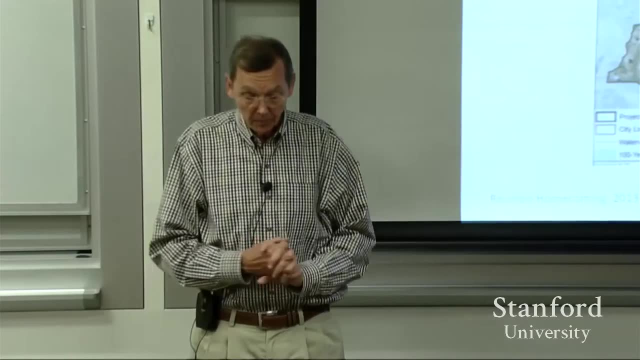 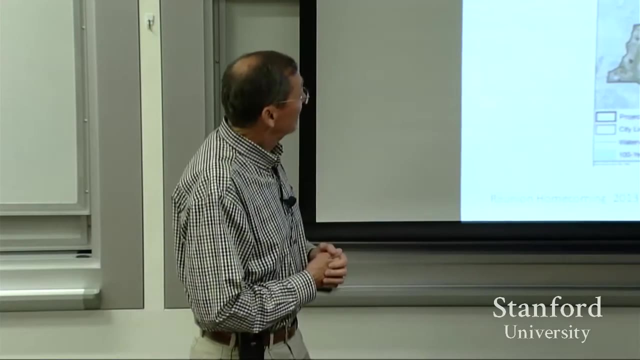 and the solutions that come up in one place are not the same for another place, But within one region, I think we can understand that working together collectively can provide local benefits. With that thought, this is a picture of Sonoma County and we're working with Sonoma County Water Agency. 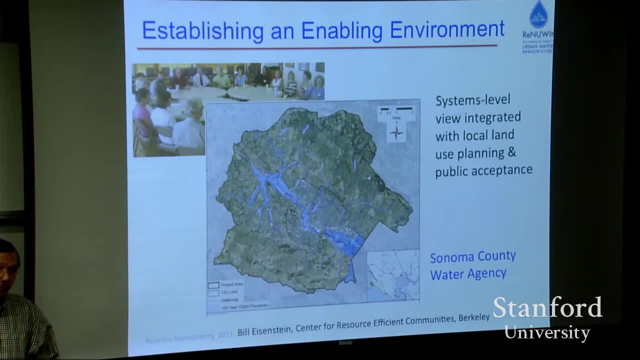 to look at the idea of stormwater capture for them. Now they've gone through a whole lot of review with their citizens in Sonoma and have said, and through a bunch of public meetings and presentations I guess like this: 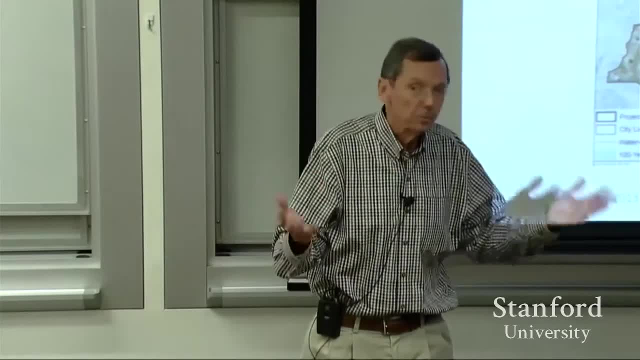 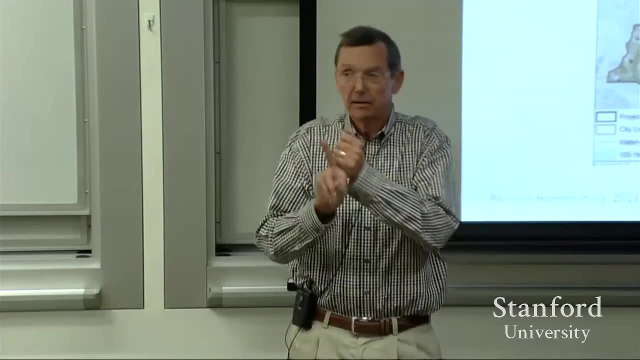 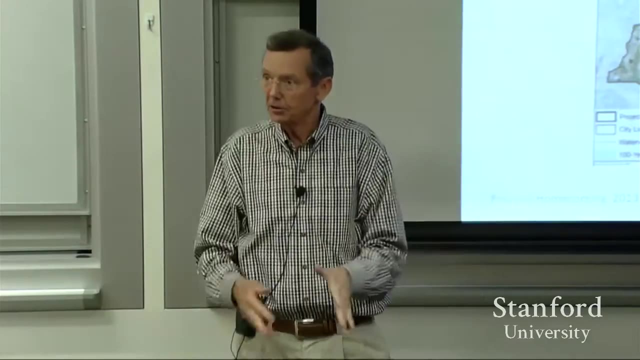 they get informed about the future of their water supply. What do you people want? What do the public want? And there were two things: Flood prevention and stormwater capture for reuse. Now this comes from a you know sort of large decision analysis. 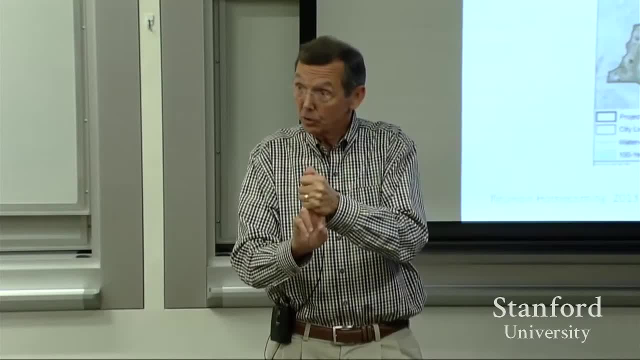 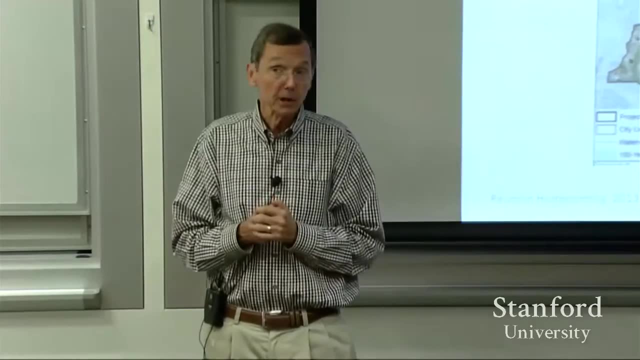 but down to those two things: Flood prevention and stormwater reuse. So what's our contribution here? Well, we're going to be looking again at some contaminant removal in those systems. but another big-picture idea is: where exactly would you put these capture systems? 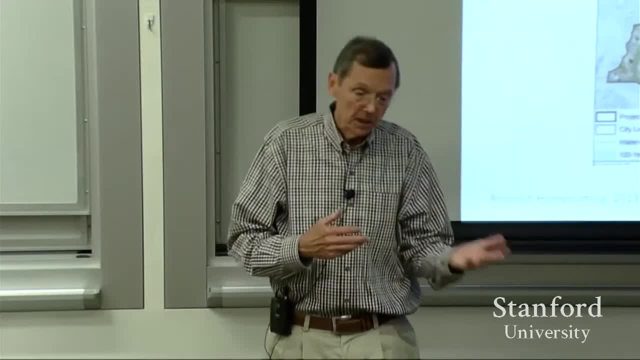 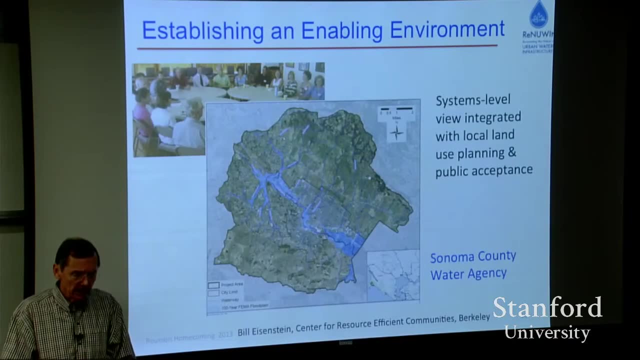 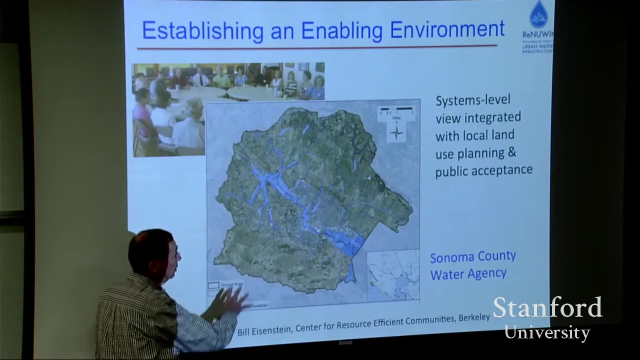 Where do they fit in terms of an urban planning context? What does it mean to repurpose some land? Would the community accept that? How many times could you replicate it? How many sites could there be that you would work at? So for this, this takes us into the realm. 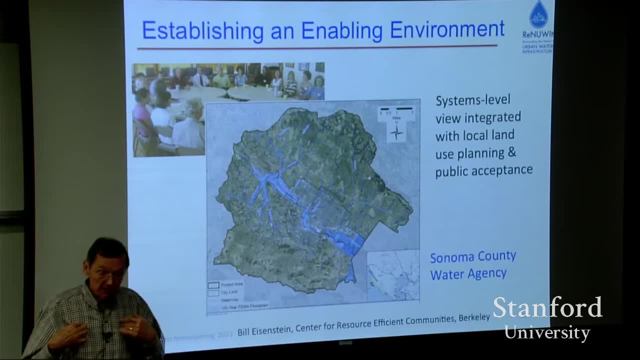 of urban planning and design, We- meaning folks like me and my colleagues- can come up with these systems that remove contaminants and collect the water. Now you say, well, where do I place them out here? Well, you can imagine that's a whole different set of questions. 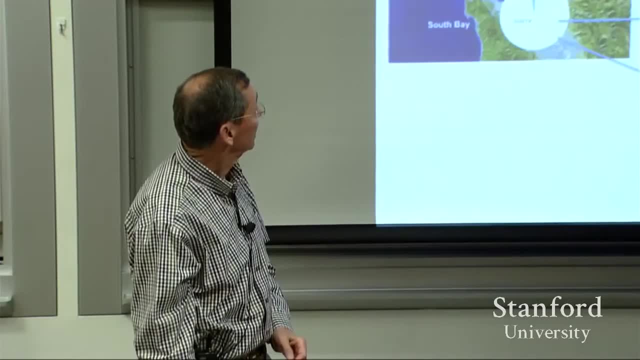 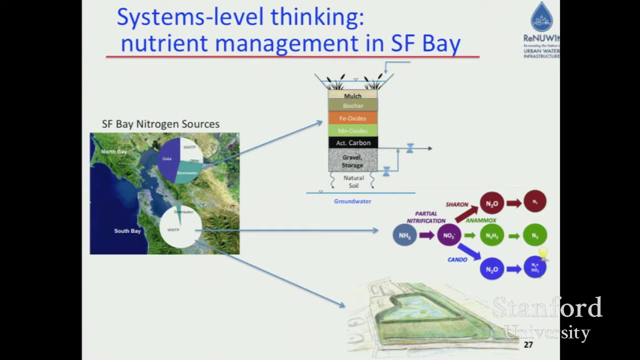 Another issue in the Bay Area that we're facing- and this is the last example- is the role of nitrogen In San Francisco Bay. nitrogen's in wastewater. It's a, and the nitrogen in wastewater is really no different than the nitrogen in fertilizer. 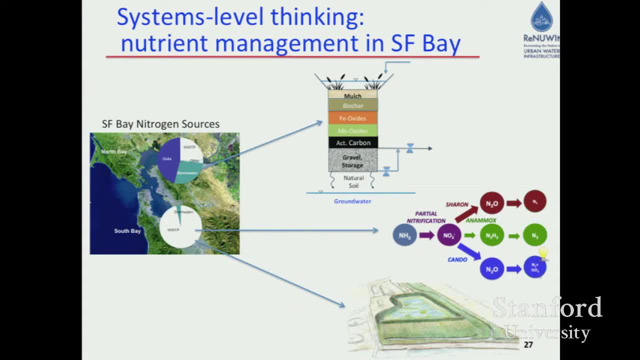 You put fertilizer on the ground and the grass grows. You put fertilizer in the bay and then what happens? Who said that You did Algae Today? yes, Some years ago, no, because the bay was more turbid. 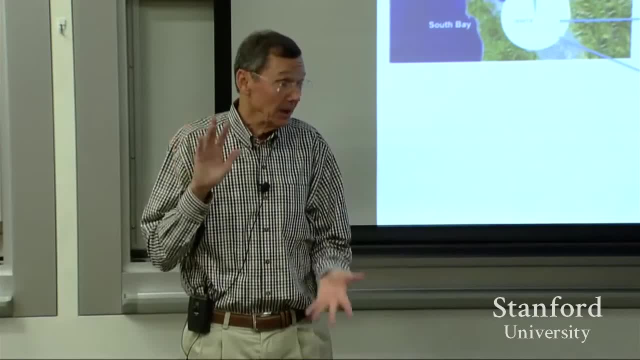 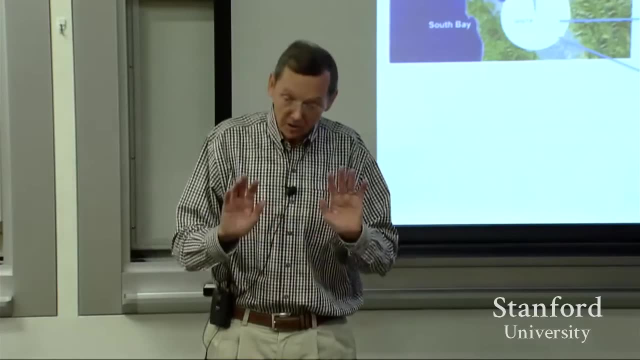 So you remember, algae needs nutrients and needs sunlight. When the bay was more turbid, this nitrogen discharge was not- there were controls on nitrogen- but it wasn't such a big issue Now, with the bay becoming clearer because of less silt input. 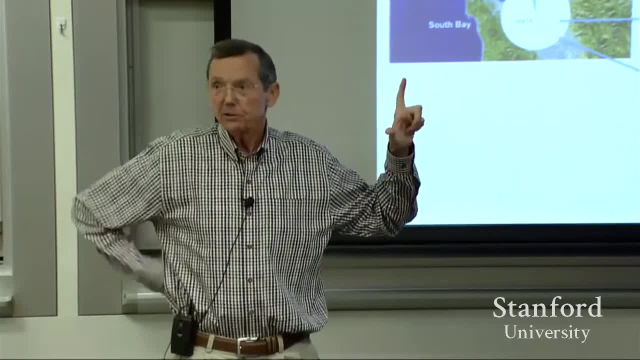 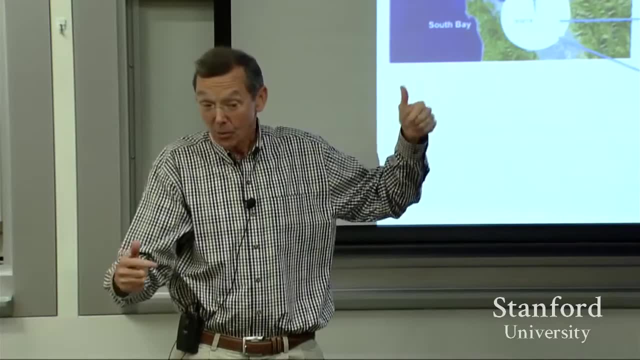 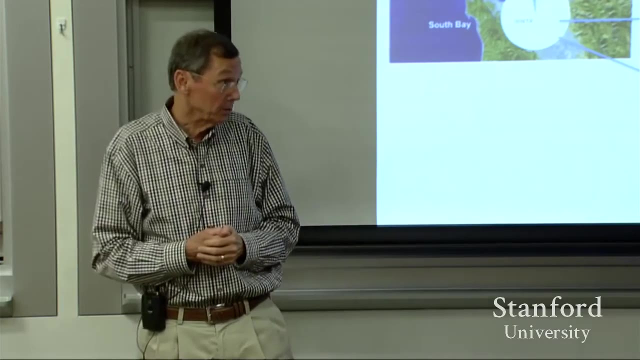 from the old mining activities a long time ago and invasive clams that sit at the bottom of the bay and act as filter feeders. the water's getting clearer, So we now are facing an issue about nitrogen removal from all these wastewaters. 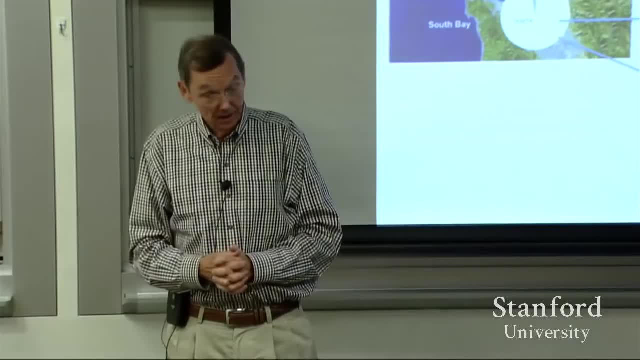 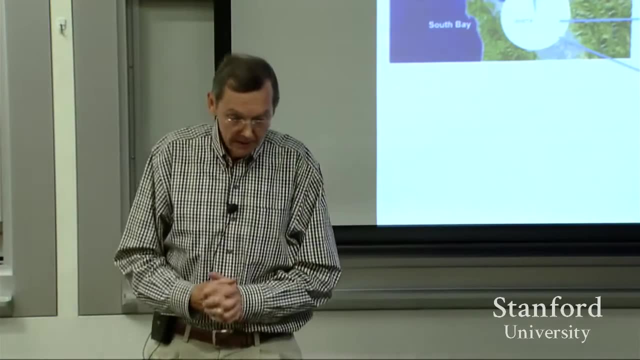 And then, how might you do this? Well man, this is a billion dollar. all the problems here are billion dollar problems. You have a bunch of wastewater dischargers that now think, oh gosh, I gotta do nitrogen removal. 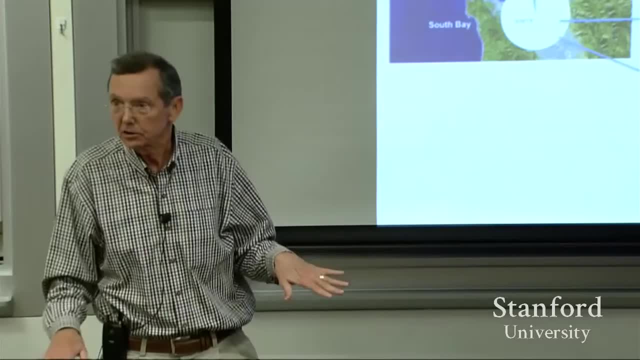 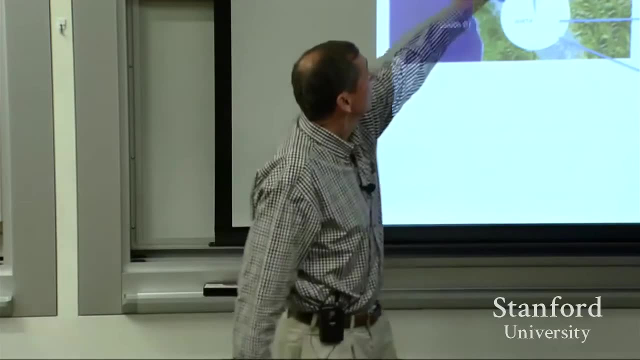 Before it was. don't discharge ammonia, because that's toxic to fish. But you can convert the ammonia to something else. Well, how might you do this? Would you go up here in the north end of the bay? stormwater's a big deal. 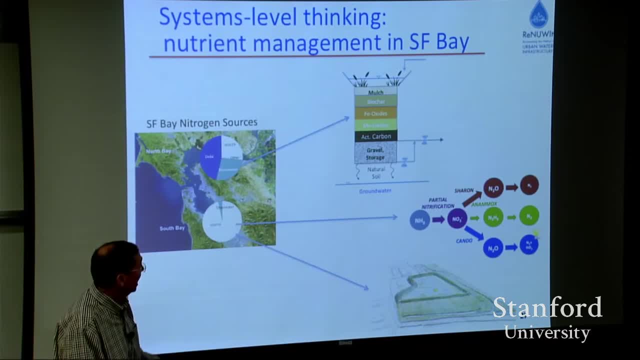 In the south end of the bay. it's wastewater treatment plants. What system might you look at to say how am I going to deal with this? And one area that we're looking at is to go back and revisit this wetland treatment system again. 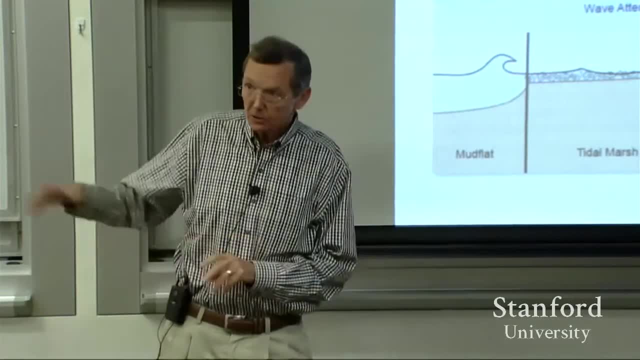 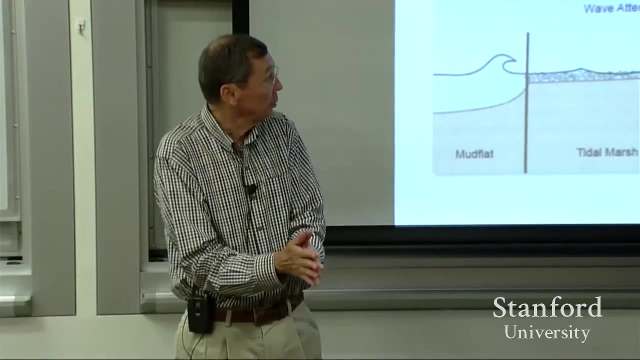 And we're working with Oraloma, which is over by, you know, just north of Union City, and are talking about, you know, a way in which we could take their wastewater, put it in a dike system and that wastewater 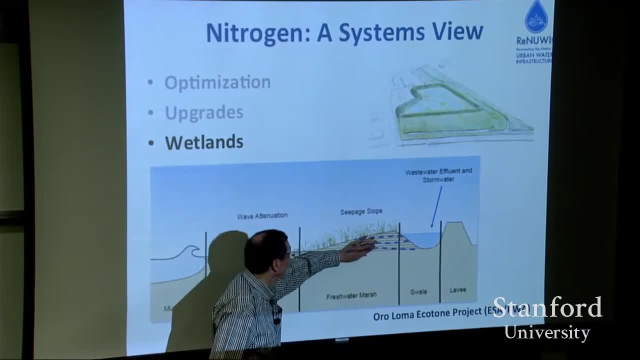 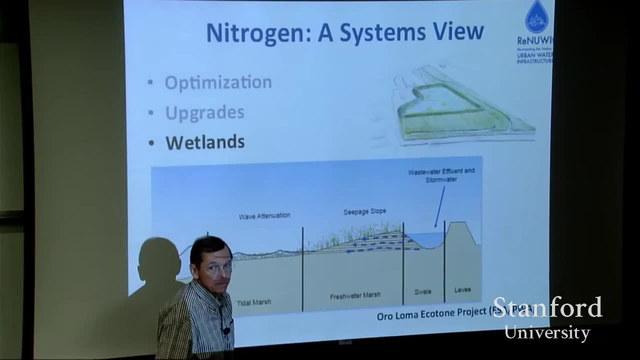 you know, which is basically clean but has nitrate in. it would flow through the subsurface And in this process here the nitrate's taken out and the water seeps to the bay. Now what's special here? 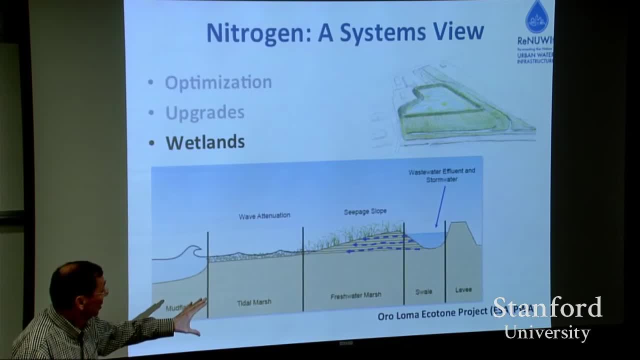 Well, this is a low energy system. You're building up a dike, a dike here that gives you some flood protection. This might work 50, 60 years, something like that. It creates a habitat where there isn't now. 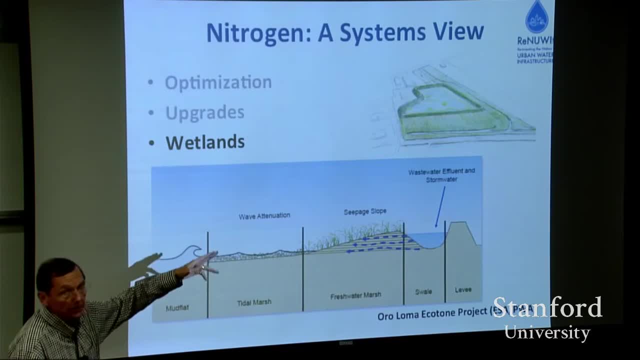 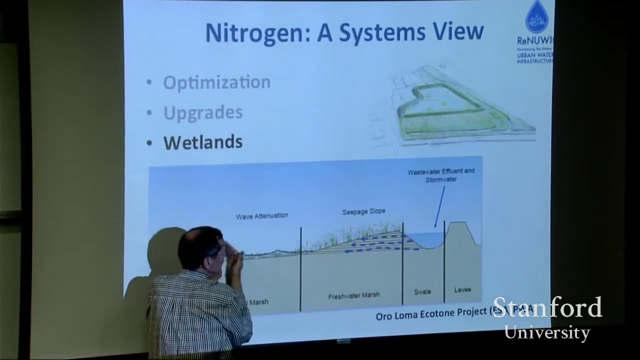 And there's also recreational benefits that can occur, you know, with bicycle paths around this kind of facility And you could imagine this expanding perhaps around the south end of the bay, This piece here, this freshwater, this brackish water ecosystem. 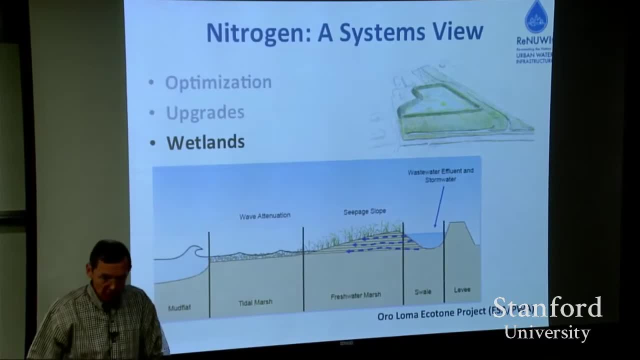 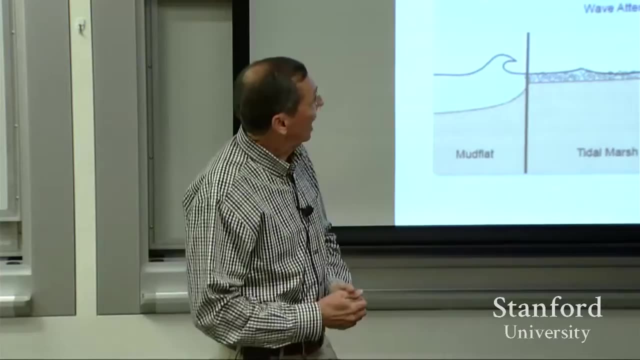 this reach is largely gone, on the fringe of the bay because of fill All right. Last slide now is say: well, how do you put all this together? Do you like this or not? How are you going to manage nitrogen? And this is where you all come in. 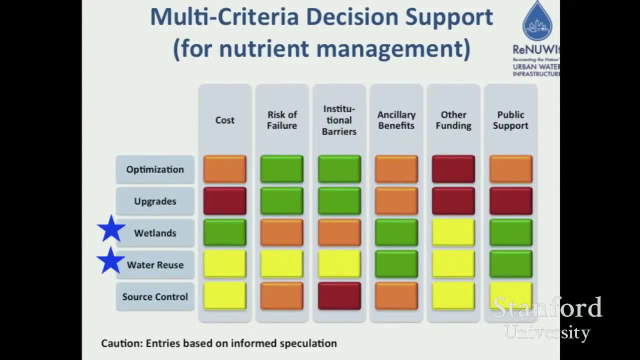 You know, you say, let's look at a decision tree here. A decision tree I mean, you know a little decision matrix. We can do various things as engineers. I could go optimize my plant. I'd get down there and tweak the daylights out of it. 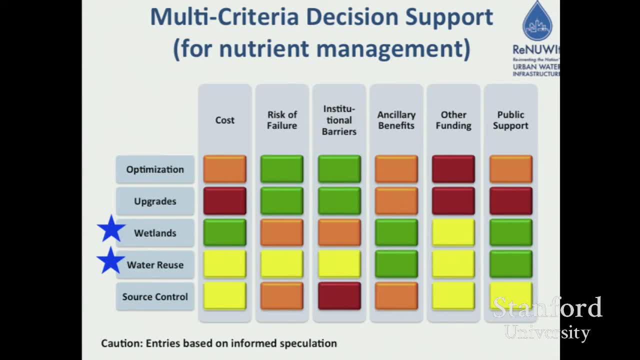 So that it works the very best it can. I can also upgrade a plant, Put more technology inside the plant fence, Or I might try this thing at Oraloma that's being designed and built- Use wetland systems, Or I might think of water reuse. 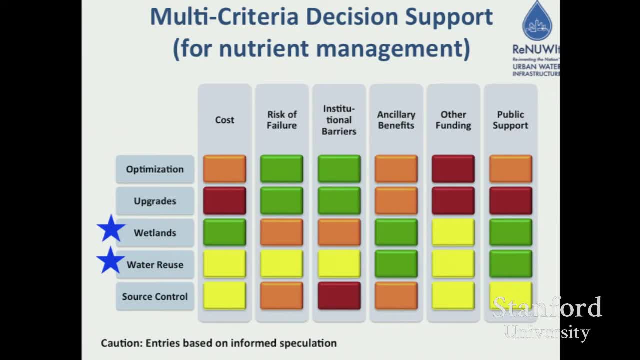 If I reuse water, I'm not putting nitrogen and nutrients back in the bay. Or I might think about source control in various ways. And then you can look at this diagram and think, okay, what's the cost, What's the risk of failure? 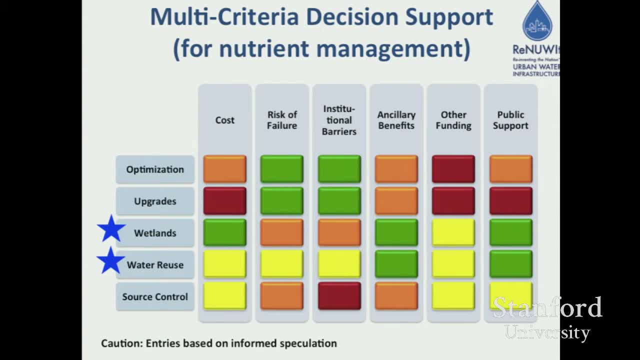 And that's a huge thing. in our field, You don't want to fail. What are the institutional barriers? What kind of co-benefits are there? Are there opportunities for additional funding beyond a wastewater treatment group, And would it be public support for those ideas? 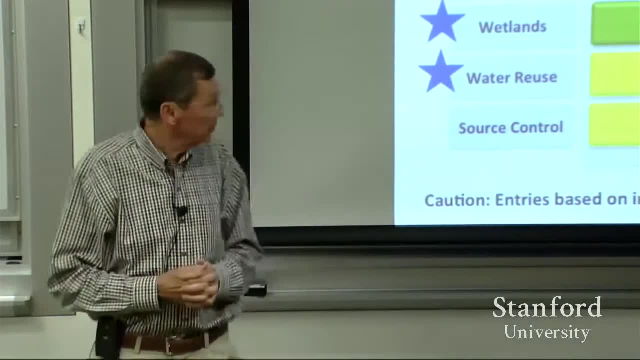 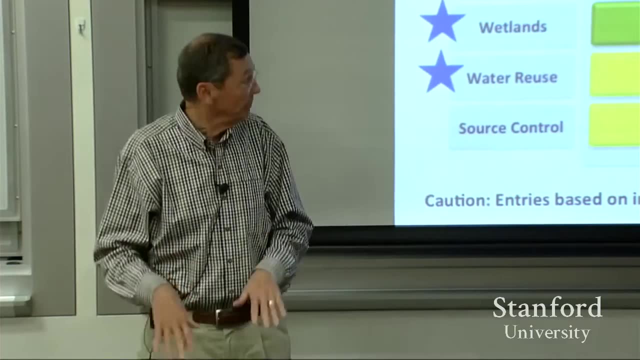 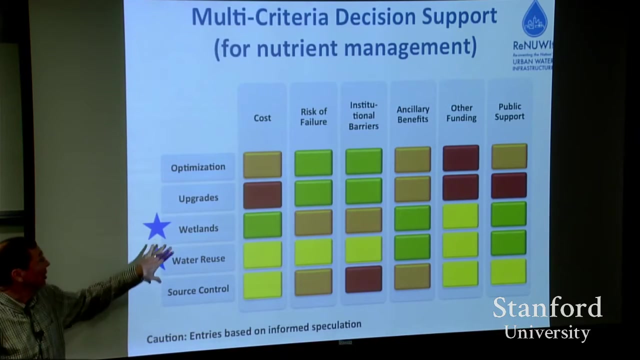 Well, what we're looking at in our center here is this idea that maybe we could help solve the problem by paying more attention to the role of wetlands and water reuse. At the end of the day, all of these will be done. 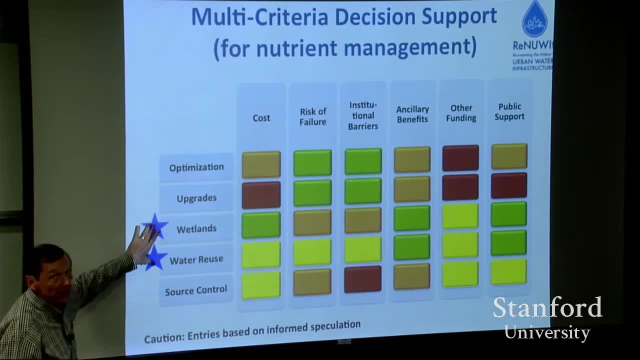 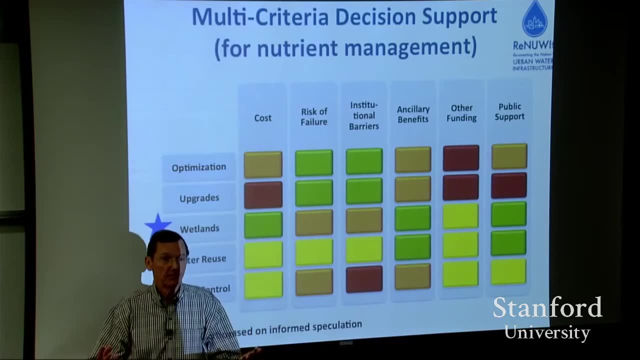 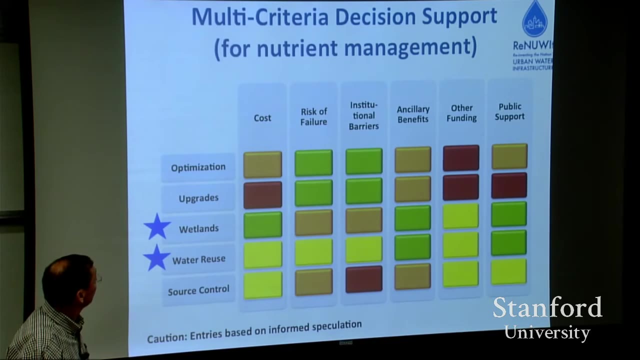 But for us, in our research, we think we can contribute here, And what I'd like to do is take some of these boxes that are orange or yellow and turn them green, And that's the role of our research. The example would be, say, risk of failure. 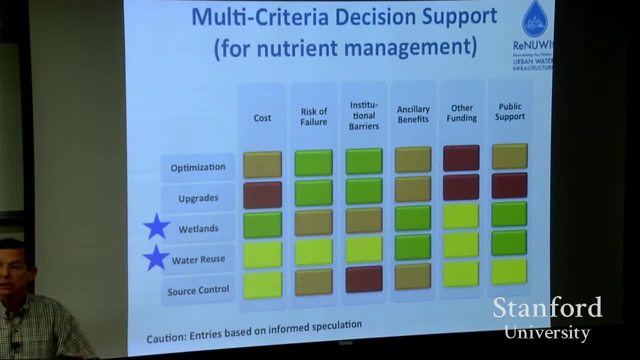 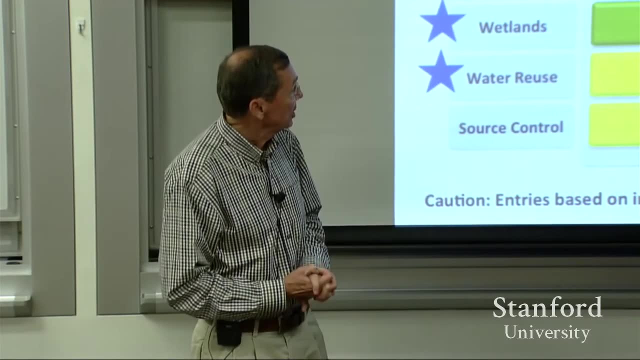 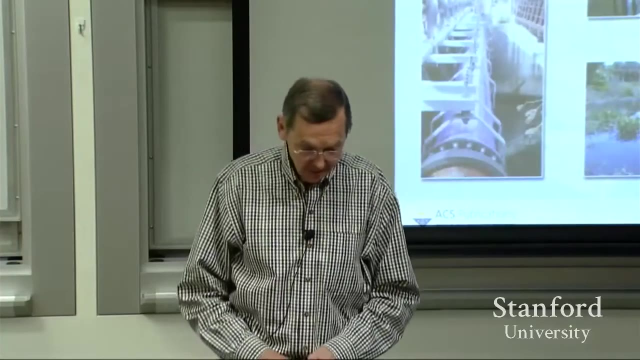 to show that, well, we can actually operate that system in Oraloma reliably to remove nitrate, for example, And that box would go from orange to yellow or maybe green in time. So to sum up then, what's the urban water in the future gonna look like? 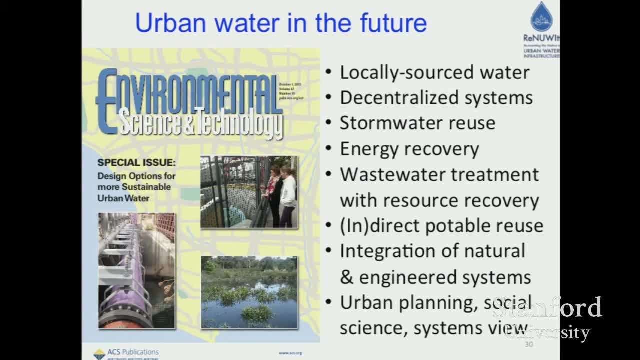 for us in California and the arid West. Well, these are the big points here: More locally sourced water. That means less imports, making do with the wastewater and recycle it and capturing stormwater. But we'll think more about these decentralized systems. 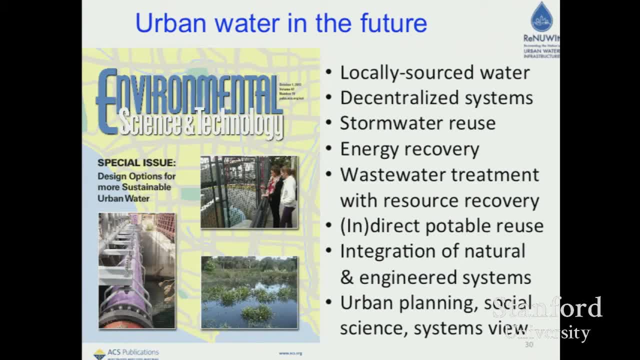 as part of our infrastructure. now We see stormwater reuse. We look at systems that are in which we can recover energy, Wastewater treatment with resource recovery. Right now, when we when I showed you that picture of that San Jose plant. 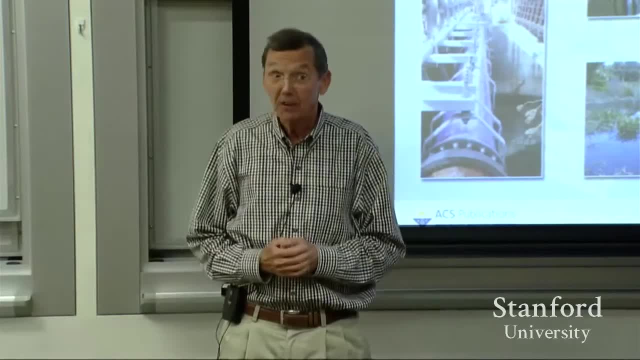 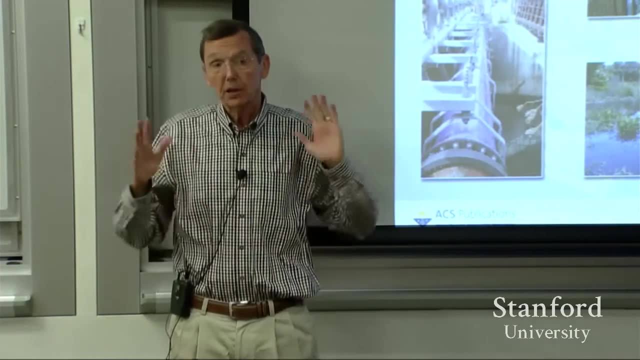 and I said it produces essentially tap water. that really is tap water, But right now it gets blended back into that recycled water. Probably what will happen in the future is, as we learn about that system and how it operates, there'll be something, there'll be another decision made. 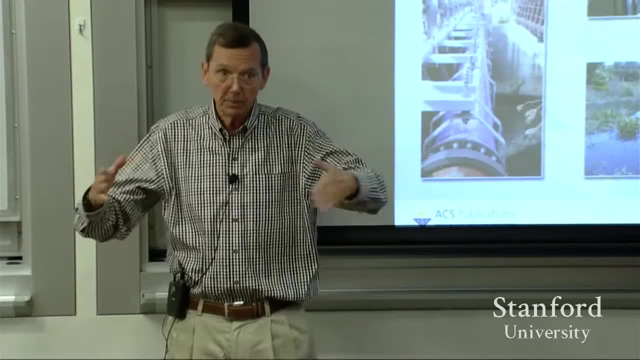 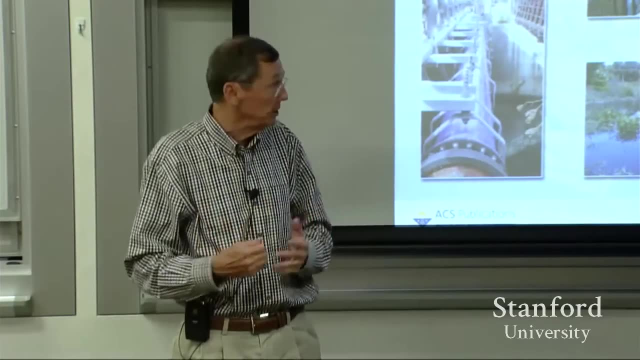 You know, maybe we should put that in a lake or in the ground because it's so good water, Why blend it with that recycled water for irrigation? So there's some combination there between a direct or direct potable reuse, But we'll see more of that. 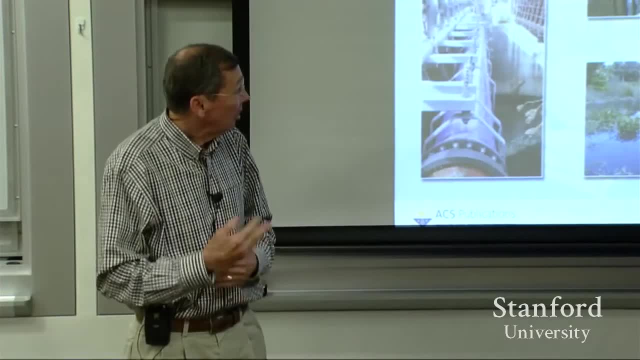 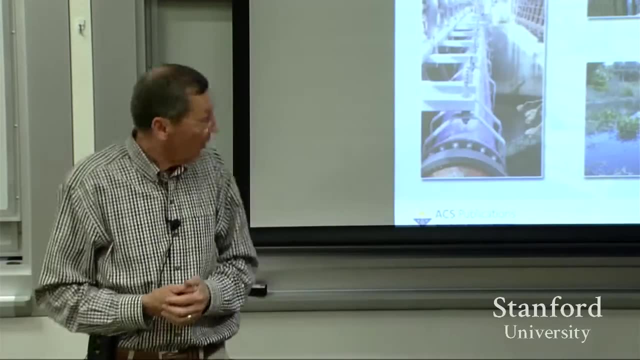 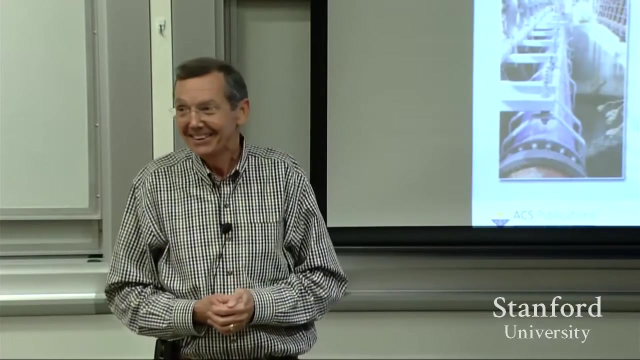 And this integration of natural and engineered systems, all in the context of urban planning, social science and systems-level view. So that's all I wanted to say. I'd be just happy to answer any questions now. We're all done. Yeah, let's see. 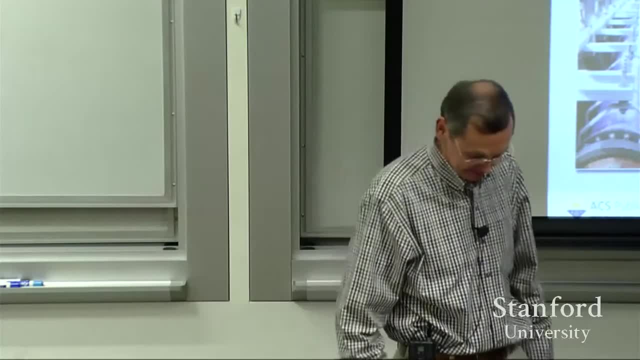 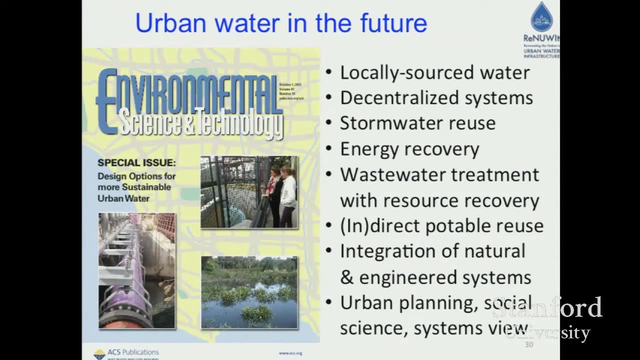 Start with students, please. So I know that among the different options that you sort of showed a bar graph of the energy intensity of different water sources, desalination was sort of the most energy-intensive option. But I know that it's being done in the Middle East. 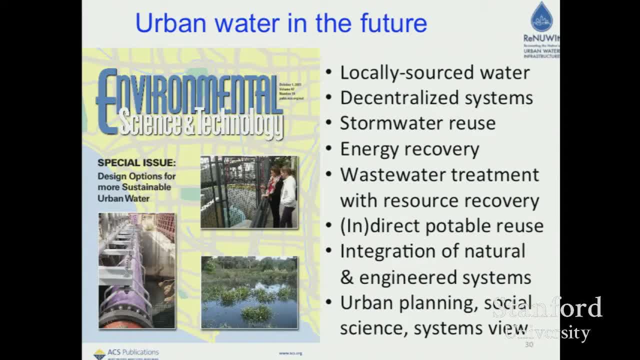 and also in Australia pretty heavily and there's a new plant going in or being proposed in San Diego. Do you see saltwater desalination as a viable option in the future? playing a big piece of the pie? The question was about the desalination. 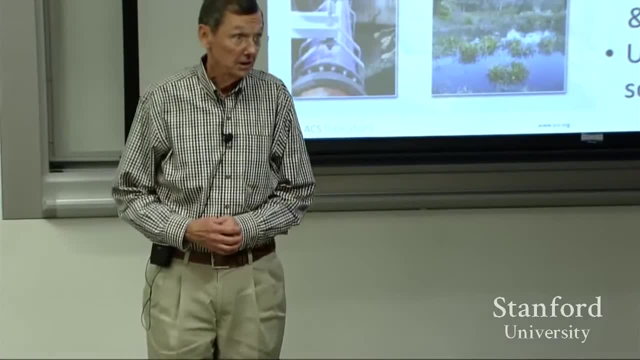 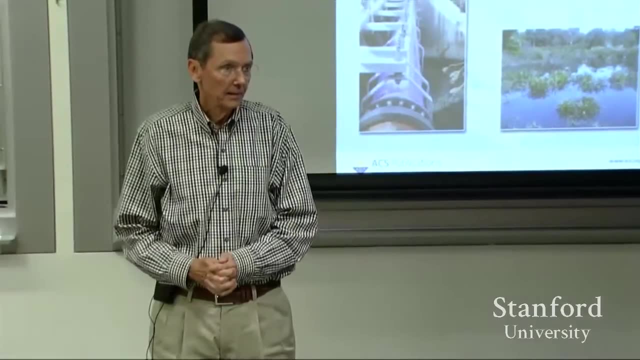 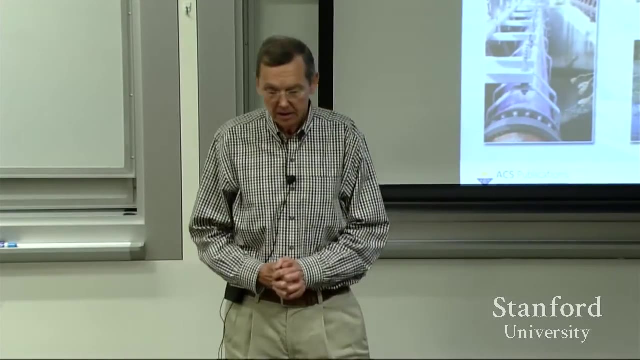 and its role in the future. It does have a role in the future, but it won't be the same everywhere. This RO, this system I showed you for San Jose, that's basically a desal system. The situation in Israel and in much of the Middle East. 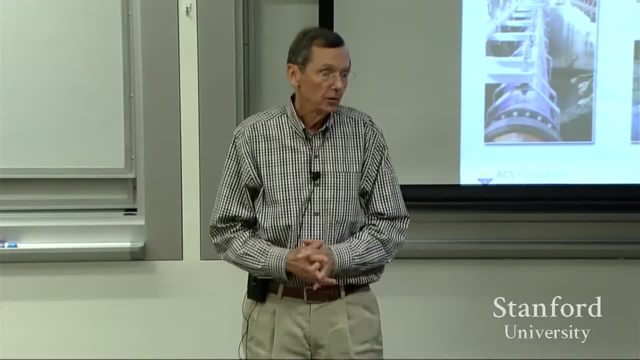 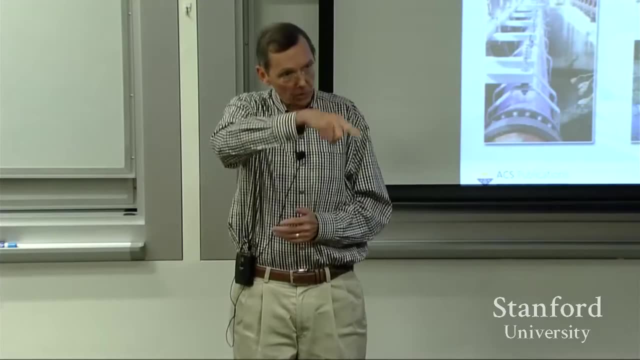 is. there's really no other water around, So they're forced to look at the ocean. When I showed you the pie chart for Los Angeles, you remember all those little wedges there. You'll note that desal is not on not one of those wedges. 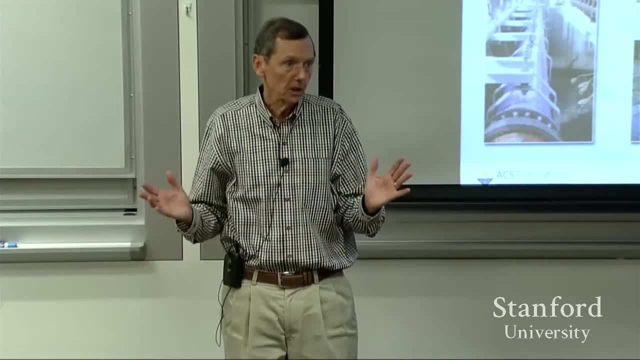 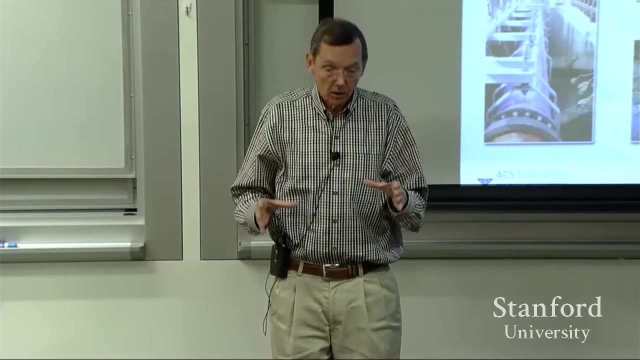 There's water reuse, there's stormwater capture, but there's not ocean desal. And why is that? That's because the community in LA has decided that ocean water desalination for their water supply is too energy-intensive. It's not sustainable. 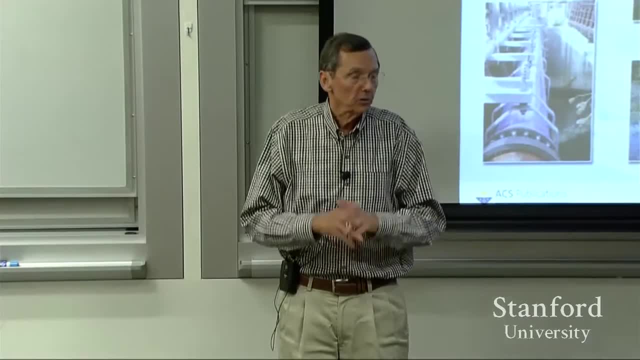 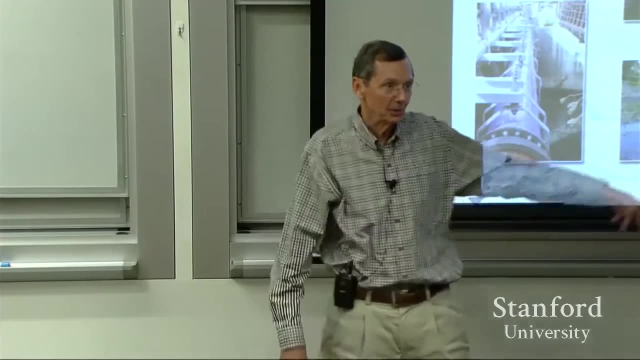 It produces a brine that might harm the coastal ecosystem. So they've decided we're not gonna do it And it wasn't on the pie chart And that's kind of a good question to ask if we had more time. is what's missing here on that one? 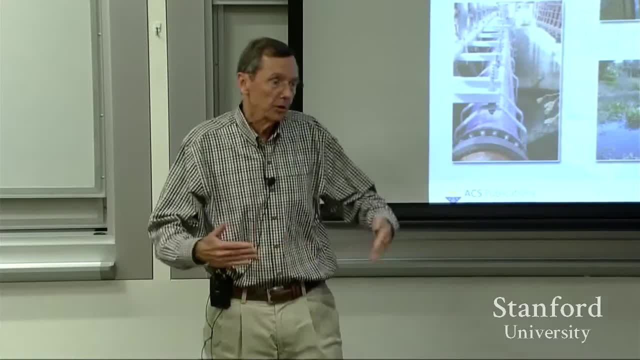 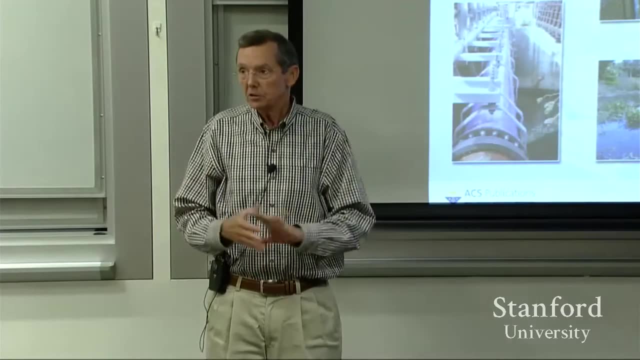 San Diego. they're at the end of the pipeline, so to speak, on all this distribution system And their options are less So. they're building this big ocean desal plant in Carlsbad, which is the largest seawater reclamation plant. 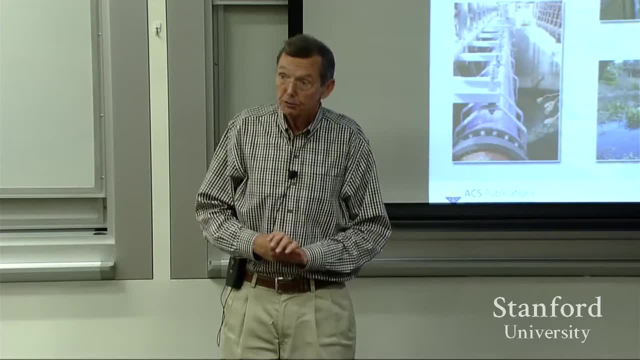 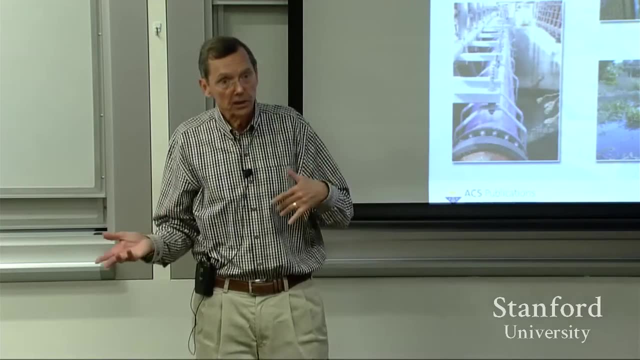 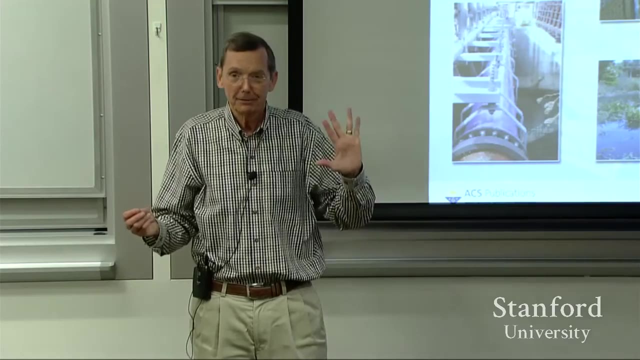 in the Western Hemisphere. Australia went through the millennium drought, 10 years of drought And all the big cities there- Perth, Sydney, Adelaide, Melbourne- I'm missing one, There's five- Brisbane- All the big cities put in these desal plants. No sooner had those been built than they got some heavy rains. So what's happened in Australia now is because of the crisis, is that we need to build big desalination plants, But now they're not operating, So they're very intermittent. 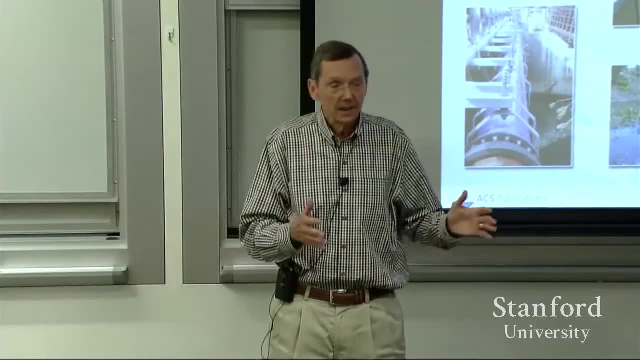 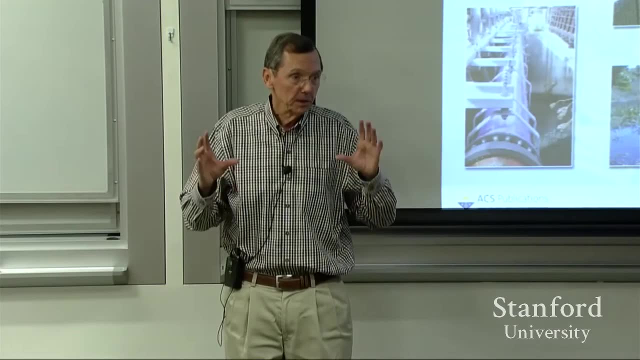 But you have to pay the capital costs. So this, to me, is a little lesson in what happens when you get into a crisis. and about these big public investments. I'm not saying that desal is wrong. Perth needs it, That's for them. 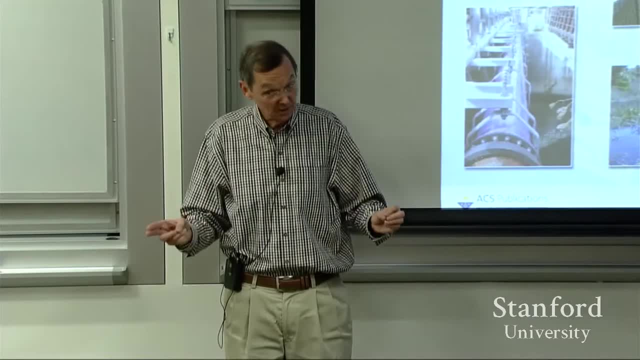 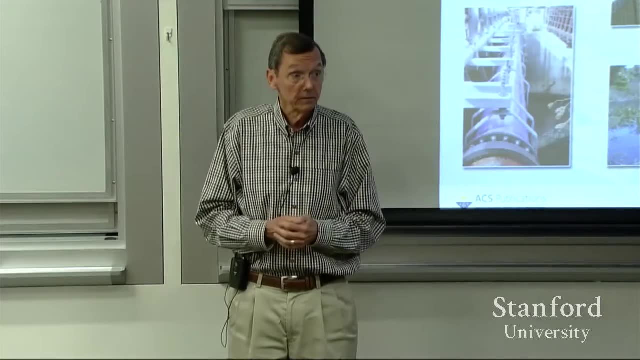 But you might think, well, maybe we built these plants too big. We could have done something better with better systems, management of our whole water supply. So in Australia there's a little bit of head-scratching then about we're paying a lot for those plants. 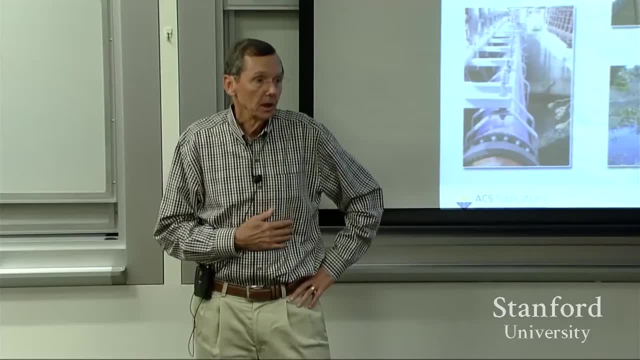 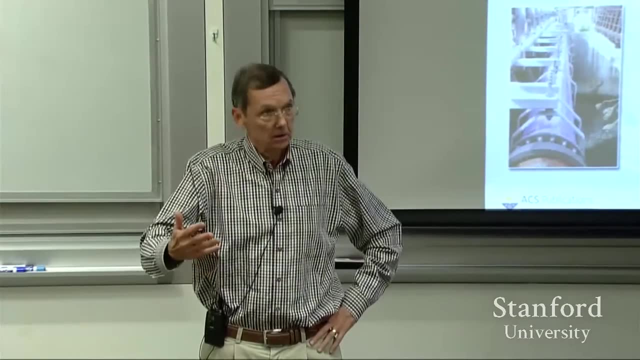 but they're not running. So it's different, And I guess my own view here is that we don't have to work with seawater. You have salts and wastewater. You have brackish water. Work with that And the energy that's required. 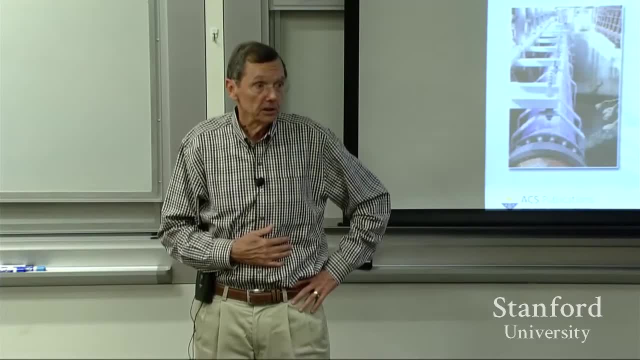 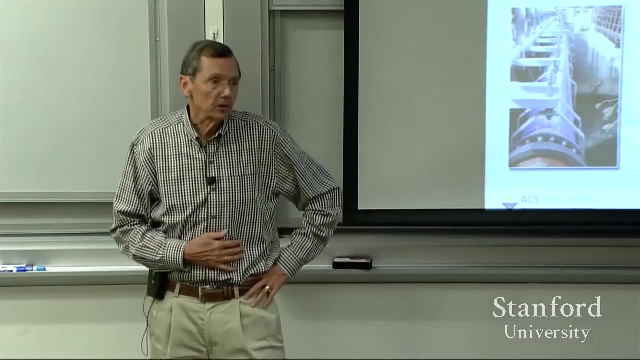 to take the salts out is directly proportional to salt content. So that's why water reuse makes so much sense. Or water of impaired quality. Think of it that way: Brackish water, That's say, one-third or one-fifth seawater. 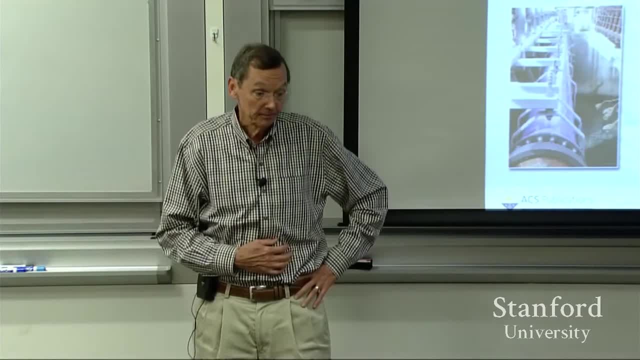 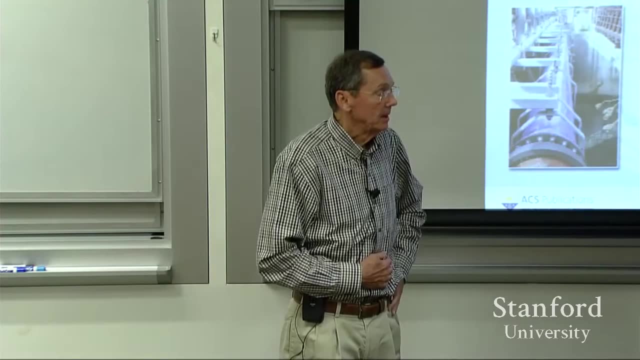 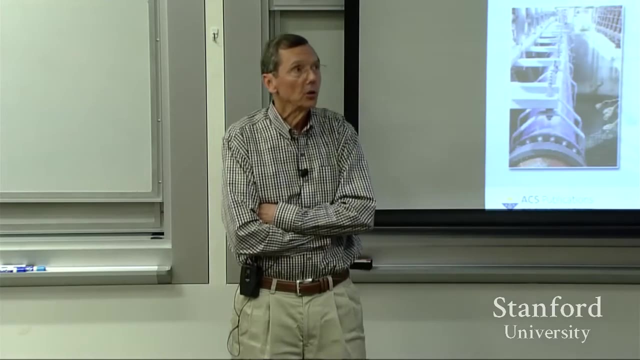 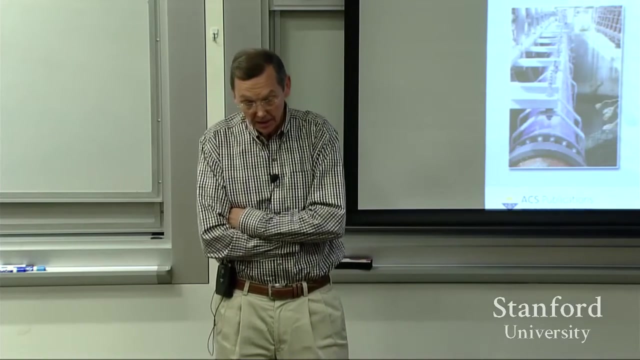 something on that order. Yes, What's being done to improve the efficiency of these desal plants in terms of using less energy? Well, basically, there's been a whole lot of engineering tweaks over the years, And there were advances in membrane technologies. that reduced the pressure requirement across the membranes. And then there was big advancements in energy recovery. Basically, you have to pressurize water to a high degree to force it through these little membrane membranes And you end up with a reject stream that's more salty. 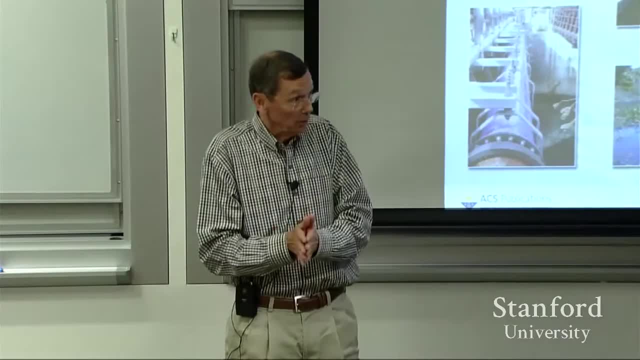 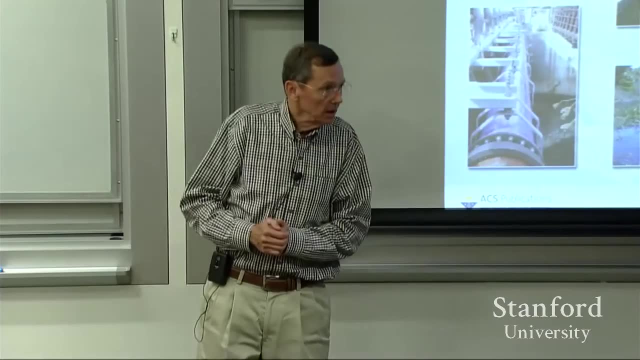 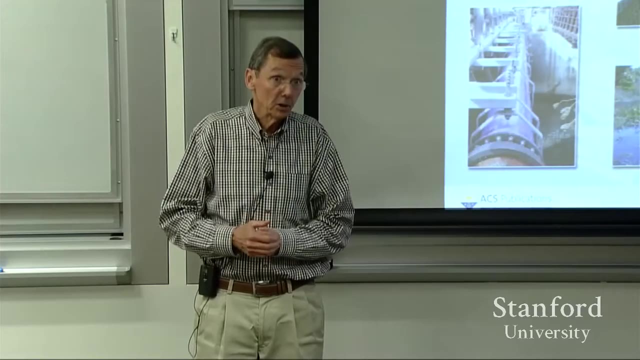 but it's at high pressure And through smart engineering you say, well, I have high-pressure water, I could run some turbines off of that, And so that energy recovery has That played a big role in improving these energy efficiency of these desal plants. 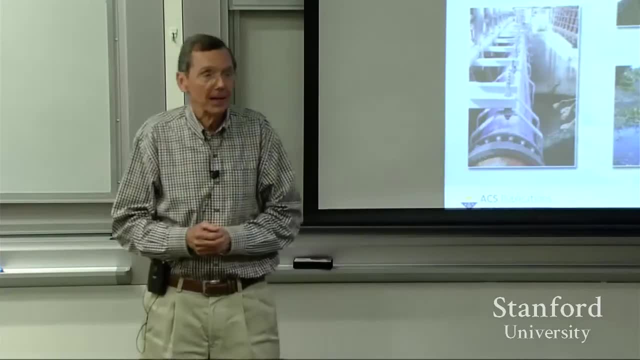 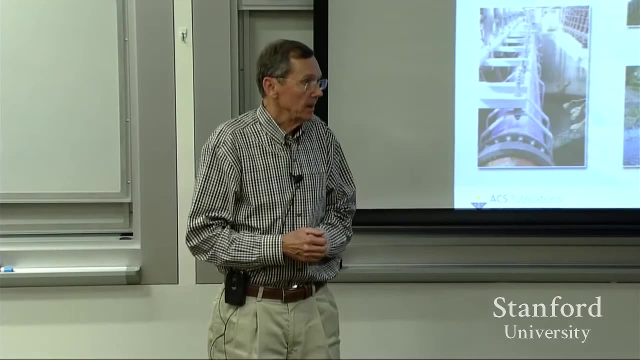 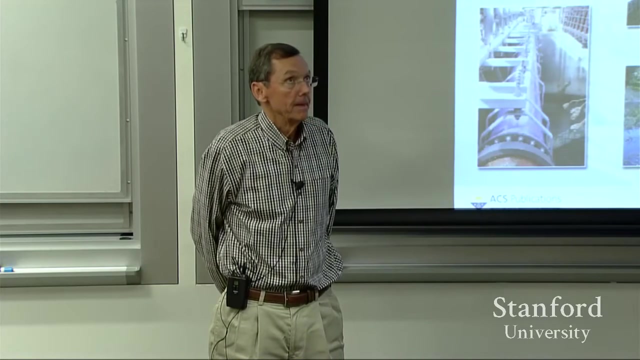 And maybe they're. How much is it? The units are just a little odd here, But it's, But there's. It sounds like there's been no high-risk, high-reward-type research In in desal. Yes, 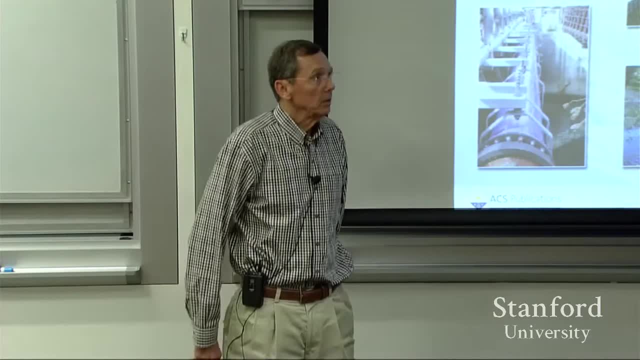 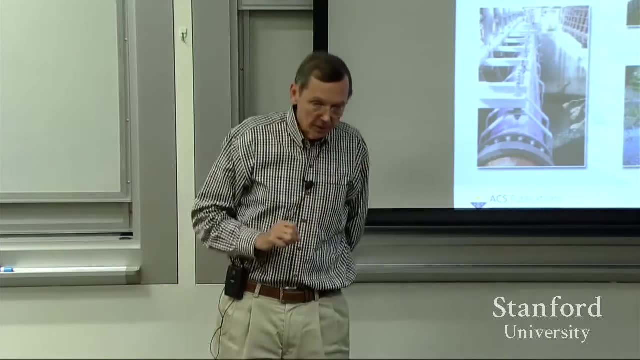 It's been Very incremental. Yes, that's right, It's been incremental. When they came to these very thin polyamide membranes, that was a breakthrough. You know, that was 20-some years ago and the other one was in all these pumps. 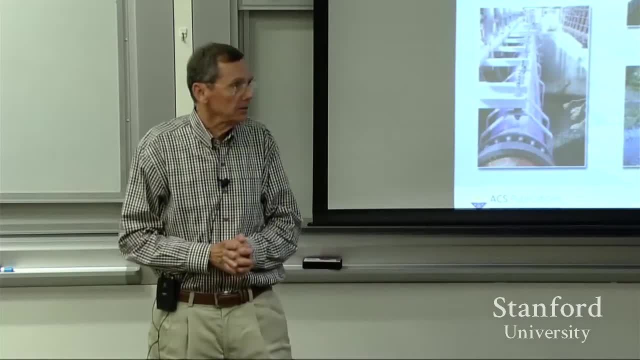 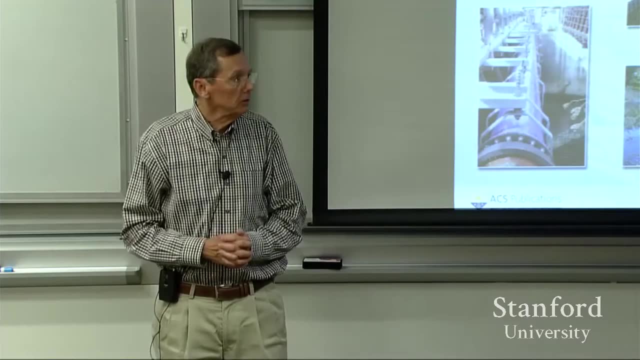 And when you have a high-pressure stream, how do you capture the energy out of it? Yeah, Basically it's the. We are living with systems that we knew about, say, two decades ago, but have made them more energy-efficient and more reliable. 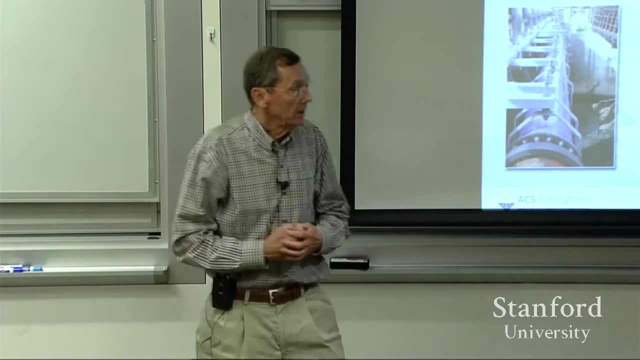 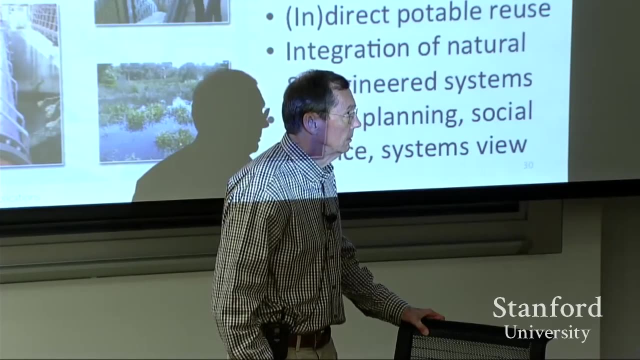 It sounds like RBE has not had any real interest in this area. The what RBE has not had any real interest in this area. RBE, RBE, right, RPE and the Department of Energy. Oh, I'm sorry. 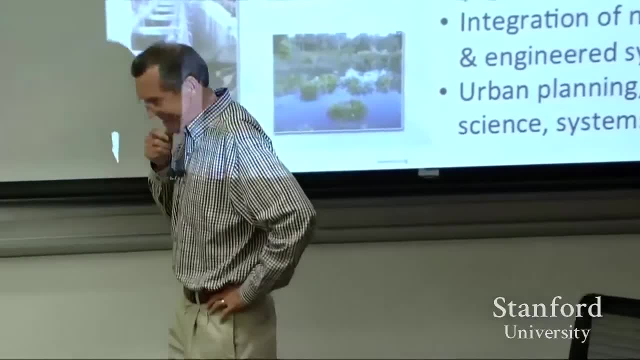 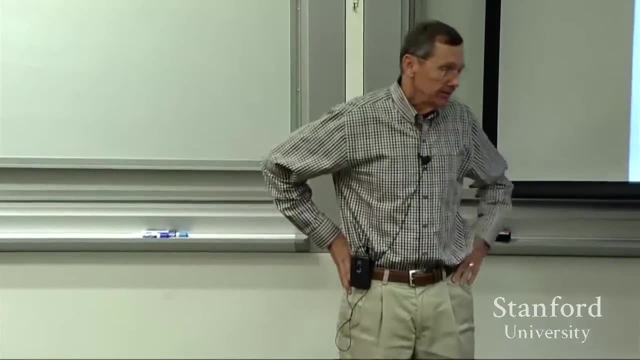 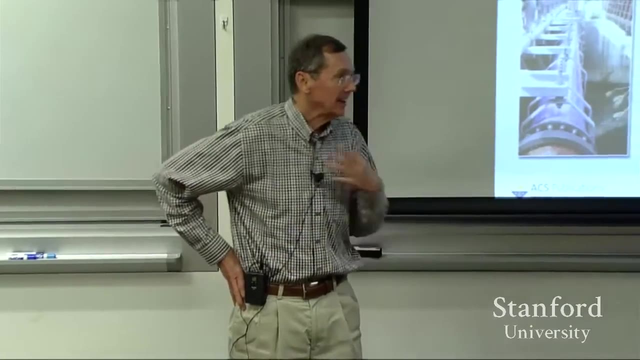 I didn't understand what you were Not directly. you know We in our field look very much at, You know, the sort of energy that's in water. That's kind of our perspective And that's an important wedge. but maybe a few percent. 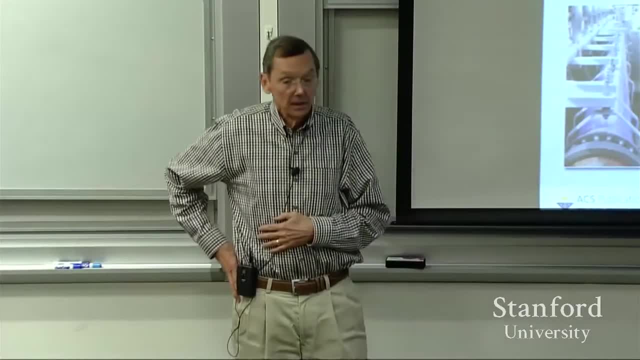 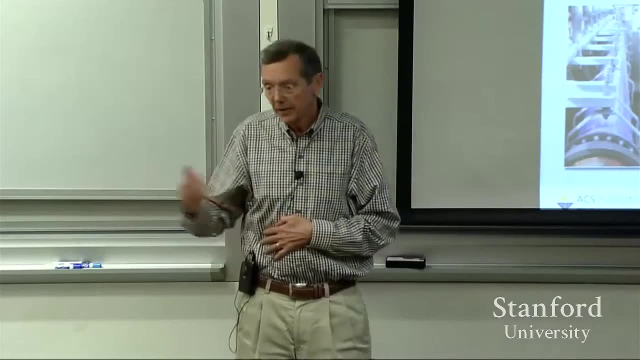 It was something that would show up on a pie chart, but it's a small wedge. The water required to make energy, Now that's a different one. You know, that's where you have all the big cooling towers and you may have the frac water. 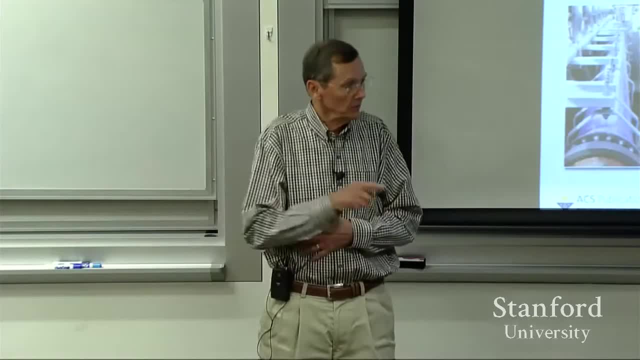 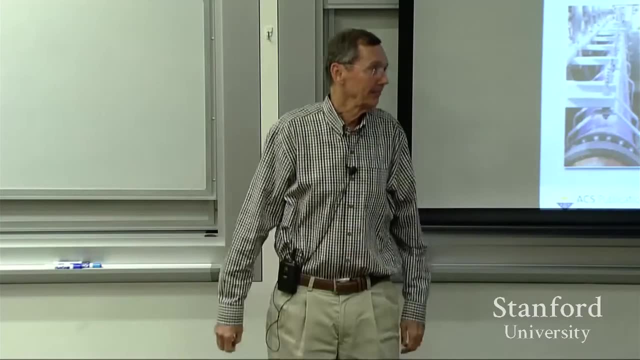 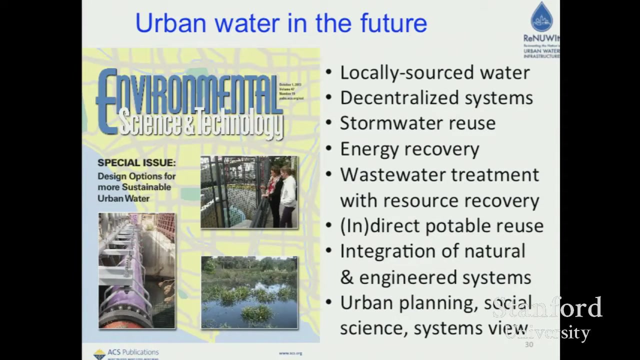 and that kind of stuff. So I think the DOE or RPE is more interested in the water to make energy. Ours is the energy in water, Right? I mentioned the CANDU project in the flow competition. Yeah, So I'm interested in the energy. 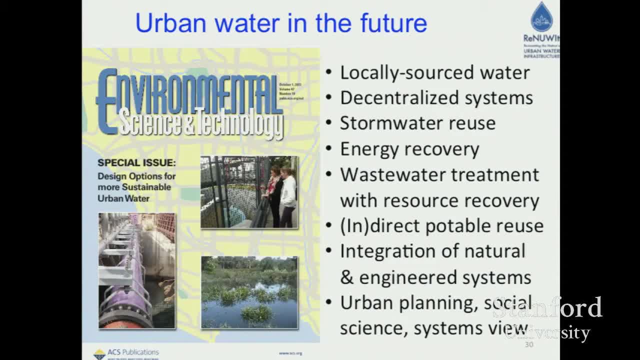 you know creating energy out of water. You were down in LA for Caltech for that. No, I was here, but I I helped him in that competition. Oh Yeah, Um, All right, let's step back for a second. 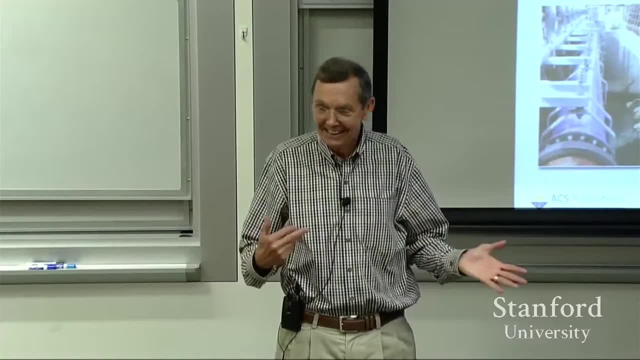 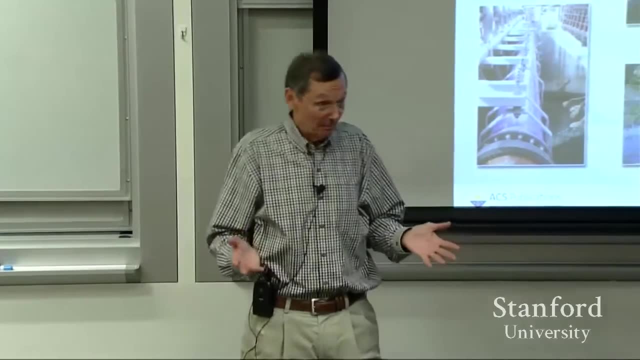 I gotta give a talk like this to the alums. you know, Uh, We touched on a lot of things here, And one of them is like energy positive treatment. How does that really work? Well, I don't think I can put up a bunch of slides. 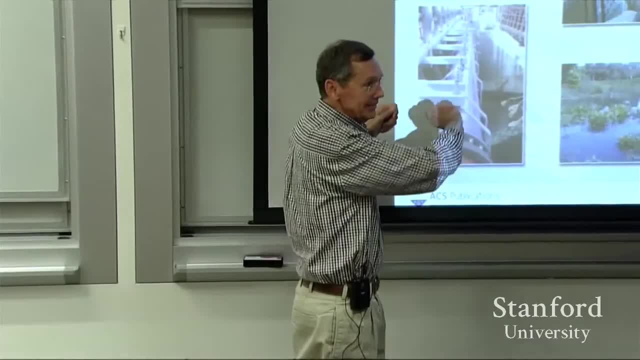 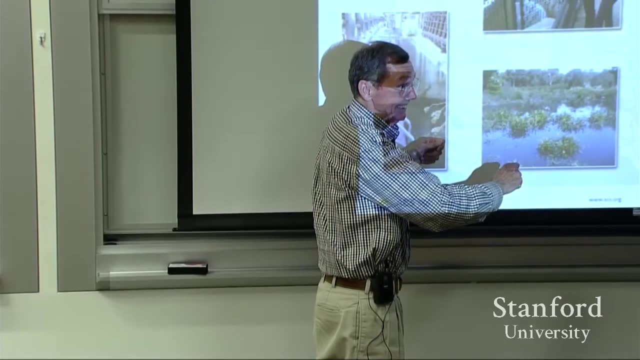 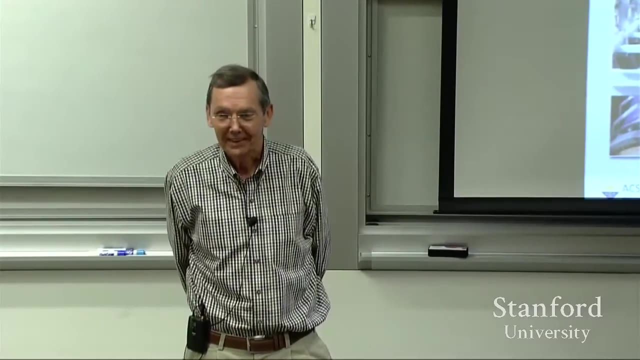 with some ammonia going to nitrous oxide, putting that down in a combustor, and No, I try to. I want to communicate that How, like nitrous oxide is in rocket fuel and stuff, because I think people visually have an idea. 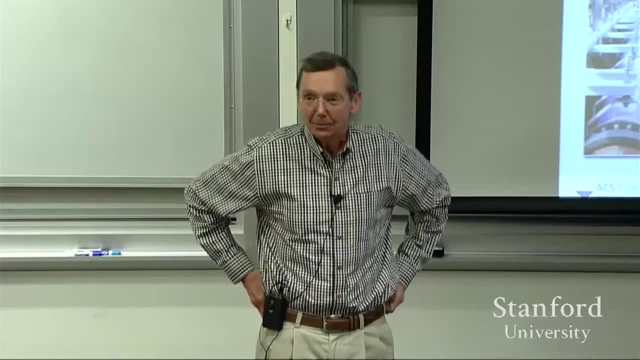 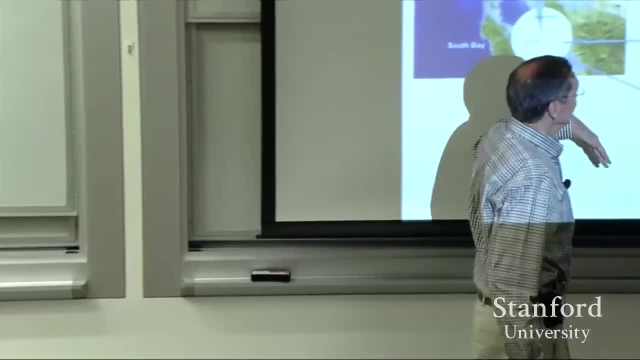 of what kind of force that creates or something. Yeah, maybe I can go back to that and say: capture ammonia is When we looked at. Yeah, this is like: uh, You know how do we deal with the nitrogen problem in the bay? 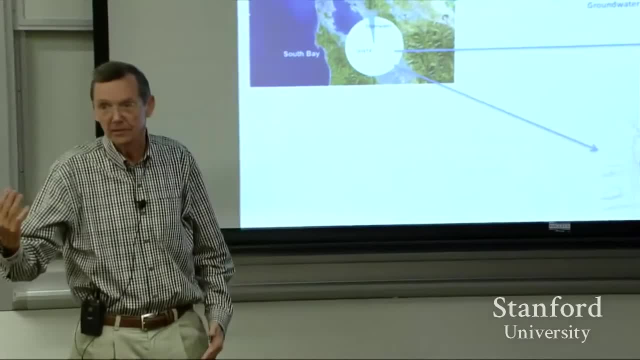 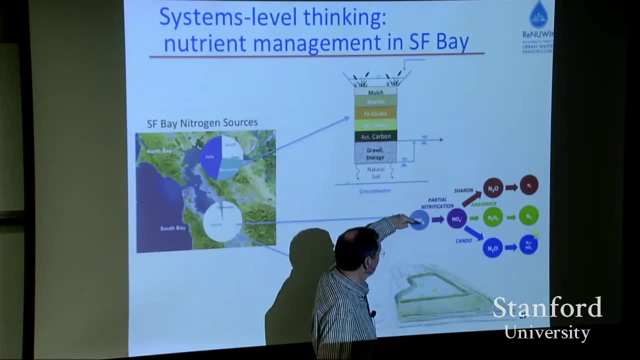 Another one is is: if you go to a complete anaerobic system for this energy recovery of the carbon, you end up with a whole lot of ammonia And there are ways- and this is what we've researched here at Stanford- is to take that ammonia. 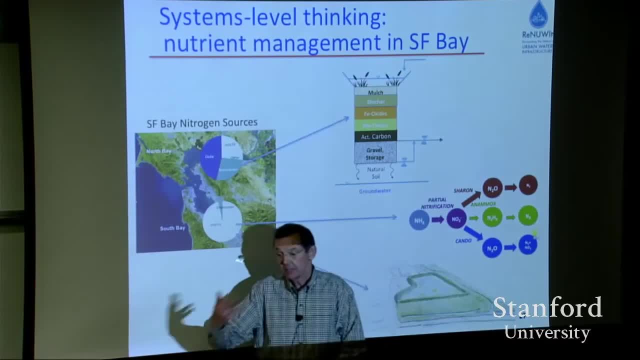 and make it to nitrous oxide And you can blend that in with the methane and you get an energy boost. It acts as a. You know it takes the place of oxygen in the combustion process. Yes, Last year you hit more on those chemicals. 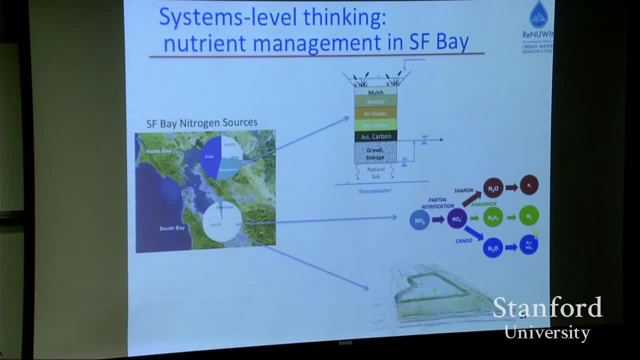 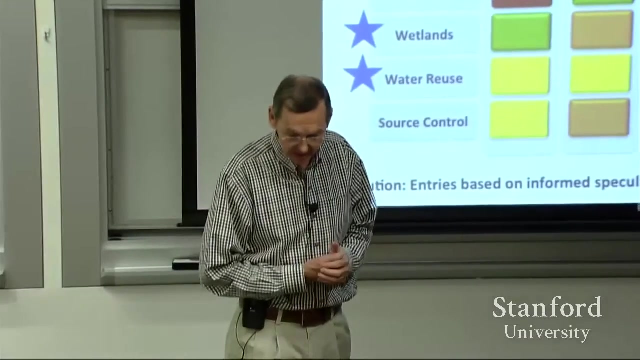 pathways and I- It seems like you've got time. That is a fascinating thing to add. Okay, I can put that in there. I'll say you have. There are different ways to address this, so maybe I can say Um. 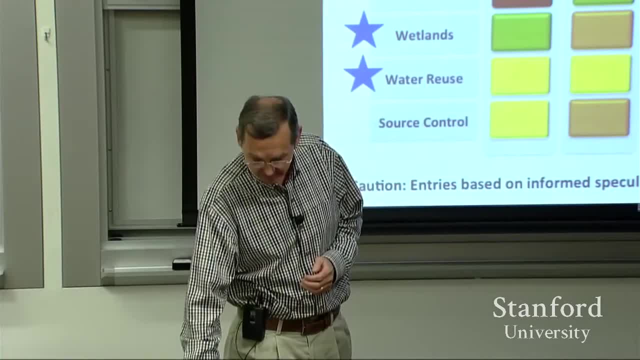 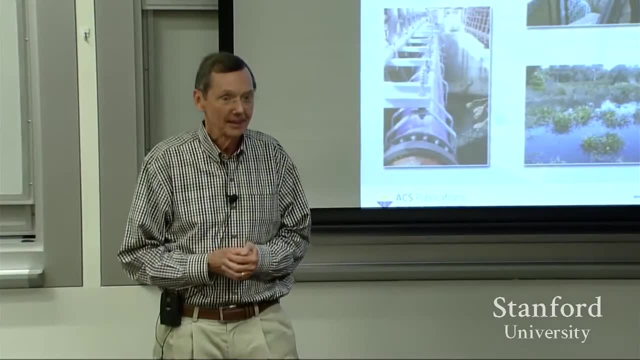 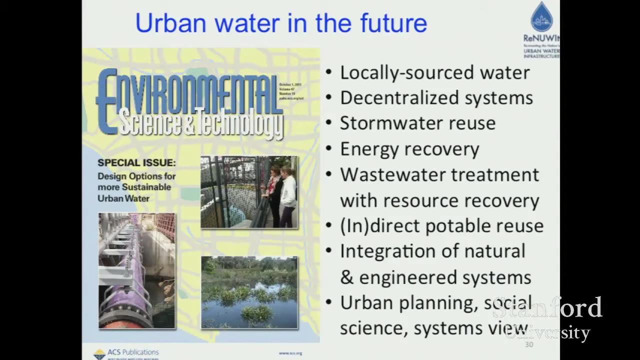 Yeah, I'd also say tying in with climate change a little bit more, especially for this class or interested you know what can you say about cities, coastal communities worrying about rising sea levels, about more severe storms, about variability of when it's going to rain or when it isn't? 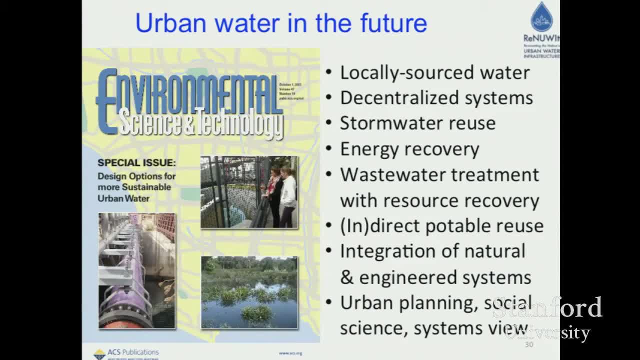 so dealing with floods and droughts with much more frequency. Things like that are just of keen interest, right And really important. Well, that's exactly. the problem we have is the variability in our water, And you know we have wet years and dry years. 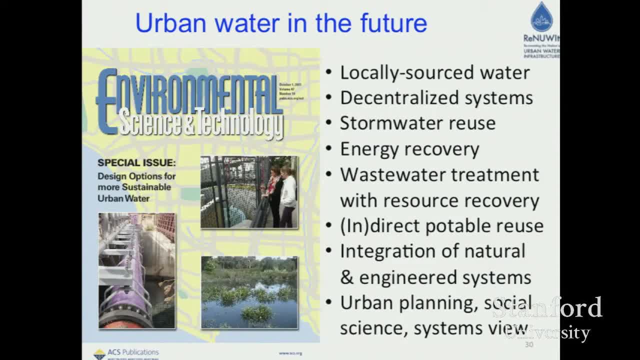 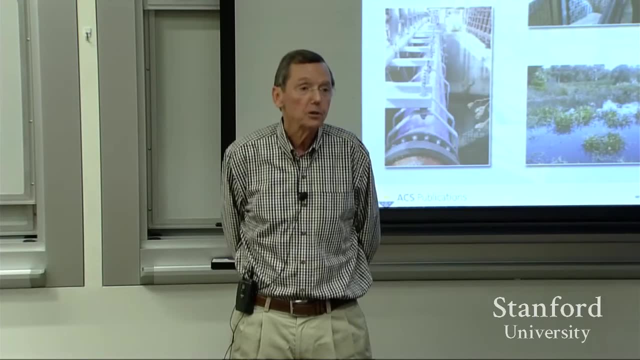 With greater decentralization and more reuse. you're kind of waterproofing yourself against that right, Right, I guess there are lots of ways to think about it. but you want to think about the resiliency of your system And water reuse. 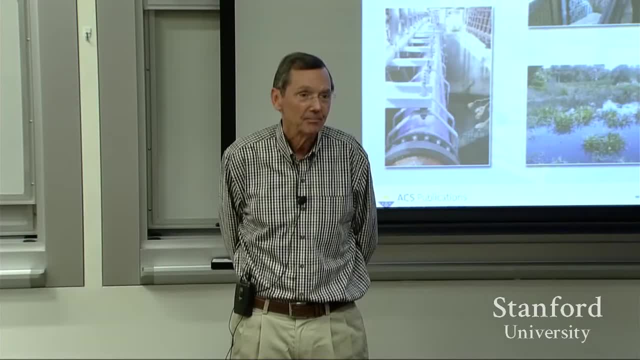 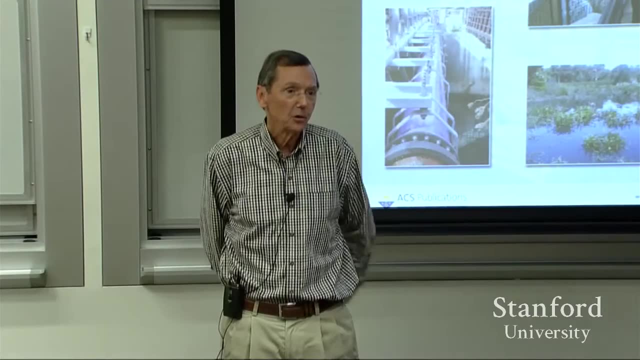 is a good, assured water supply. Stormwater capture is making use of water that's currently available, but we're not using it. So those things have, you know, saying oh gosh, we should be doing that to a larger and larger degree. 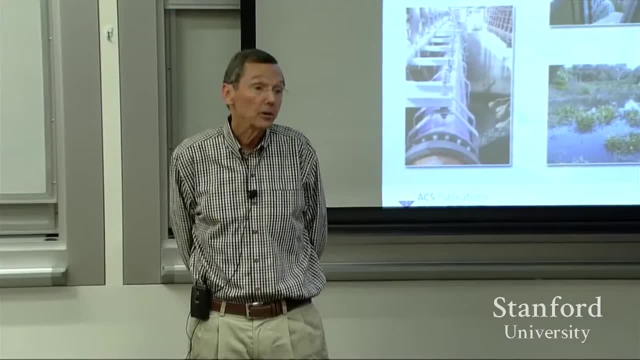 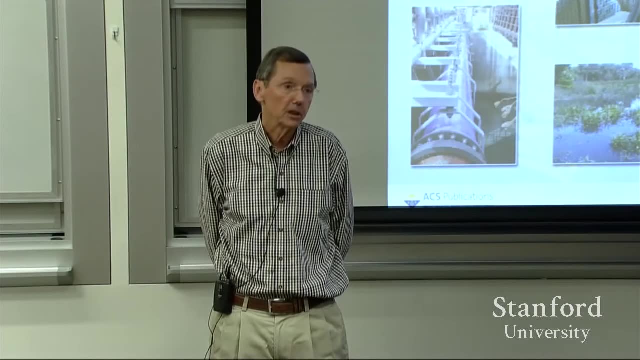 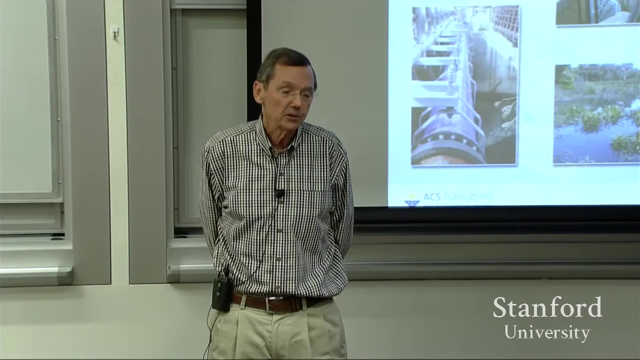 And that means we're less dependent on the water imports, And the water imports are hugely affected by climate change, And that's water from the Sierra Nevadas, the snow melt or from the Colorado River. So the future here is: there's a lot of challenges. 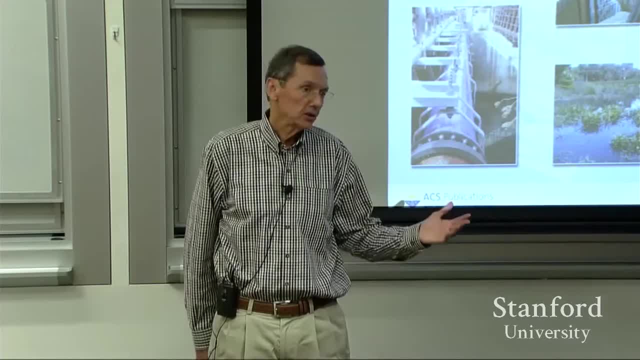 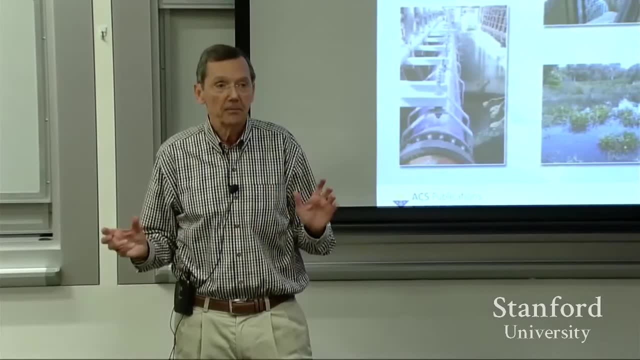 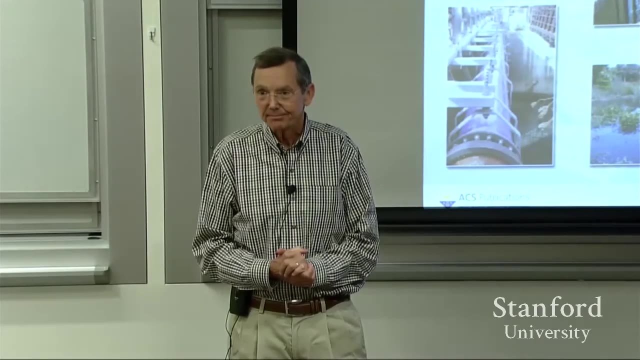 about how we manage those systems And historically it's been the tension between agriculture and cities Who gets the water. But there's a third claimant now. I was in school when the Clean Water Act was passed And basically it said you couldn't. 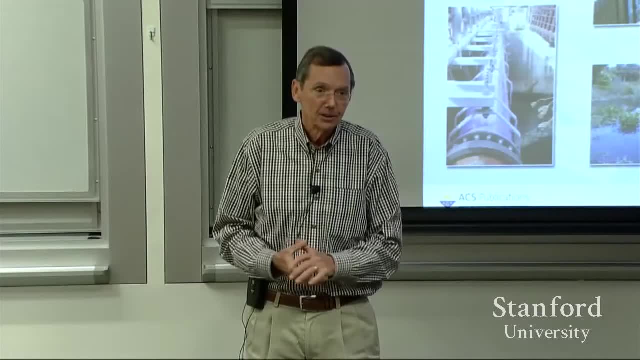 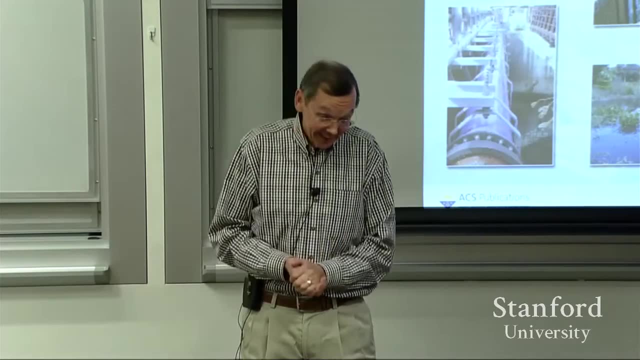 kill the fish, you know, with your waste, But there was nothing in that act that said you couldn't take all their water. You know? Yeah, Now we realize we can't take all the water, So we need to provide more water. 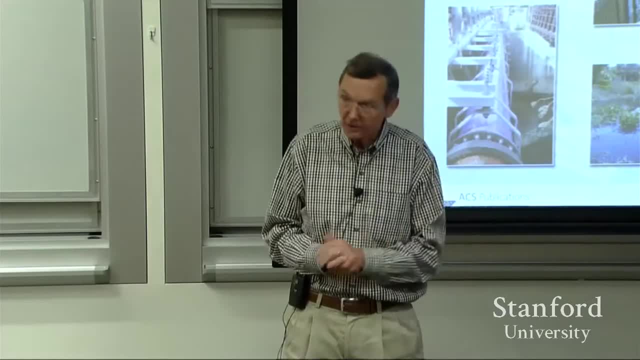 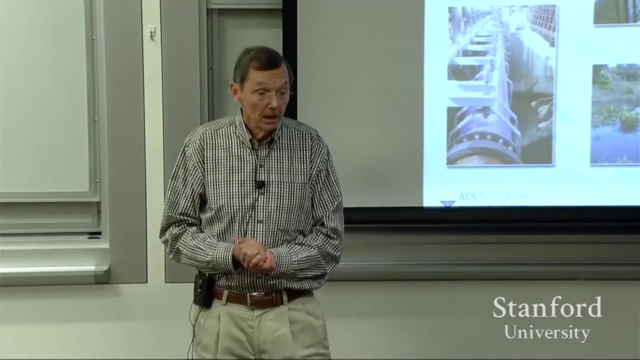 for ecosystem services. In other words, the San Joaquin needs to flow And right now it's. you know the water. you have these diversions and there are places where it doesn't flow in the summer. Another example: 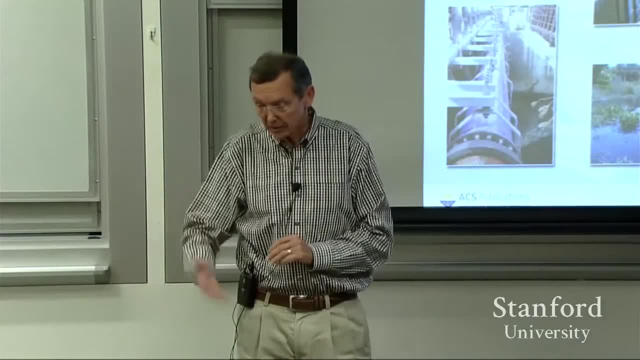 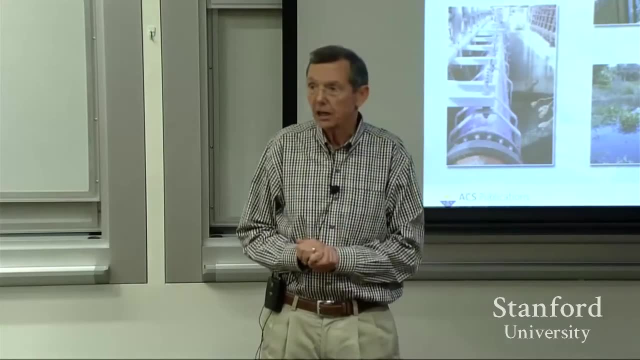 is the Carmel River where they would put so much of that. those groundwater wells were pumped to such an extent that in the summer the Carmel River would go dry. And then there were. this was, it's the peculiarity. 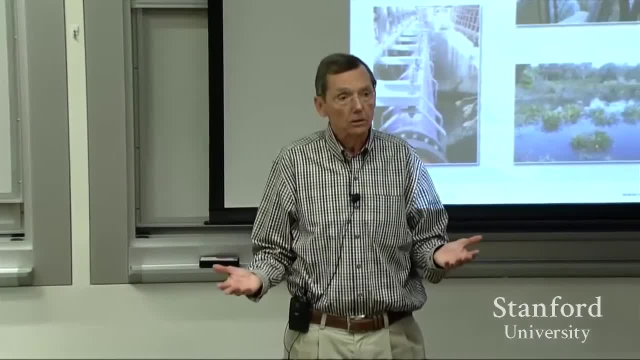 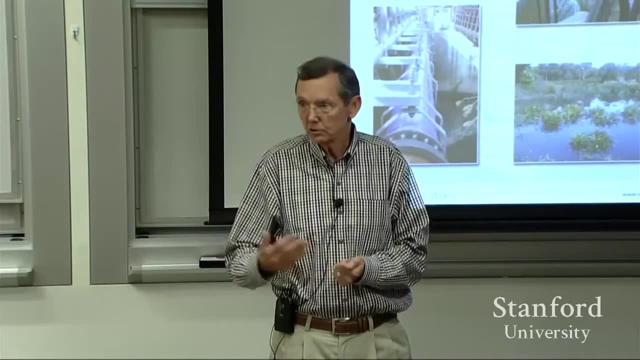 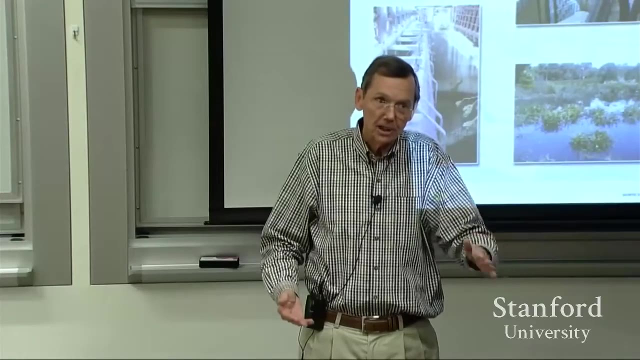 of California law that groundwater uh is not managed except in certain situations. But surface water is Surface water. that's what you can go out and see. That's managed and highly regulated Groundwater. it all depends on where you are. 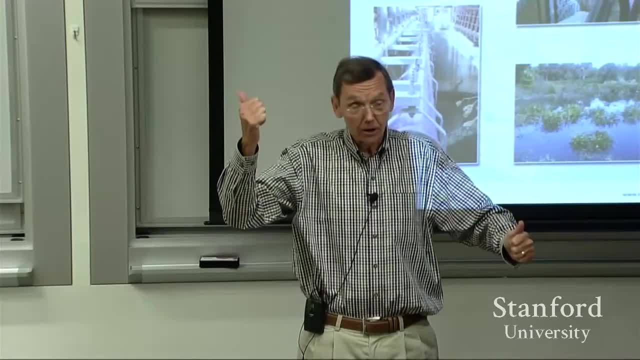 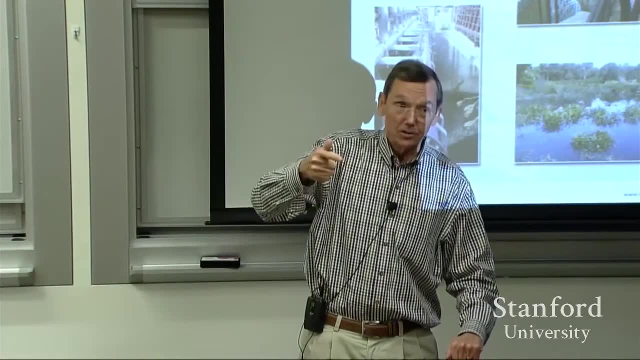 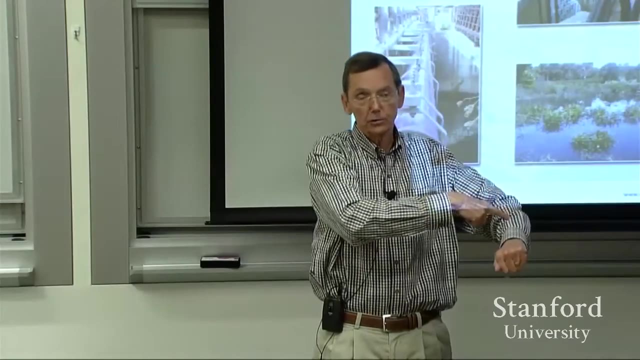 So what happened there is that the pumping of the groundwater in Carmel depleted the Carmel River, So Carmel's water supply. you know this is California, American water. they said you gotta stop pumping your wells because you're impacting the surface water. 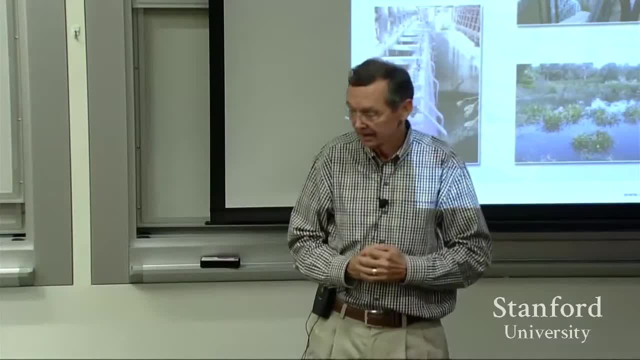 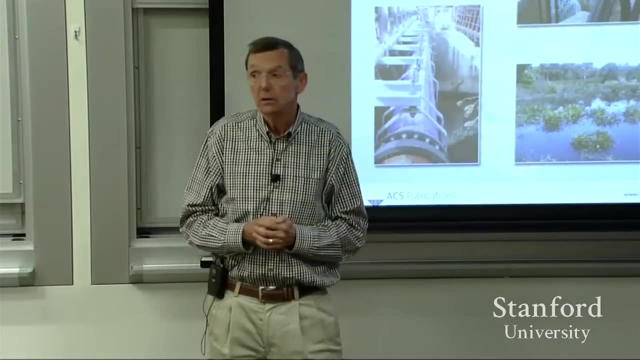 here And they could show the direct connection between the two And for them then now they're looking at lots of alternatives. What do you do in Monterey and Pacific Grove? And again, it's not gonna be one answer. It's a combination of more recycle. 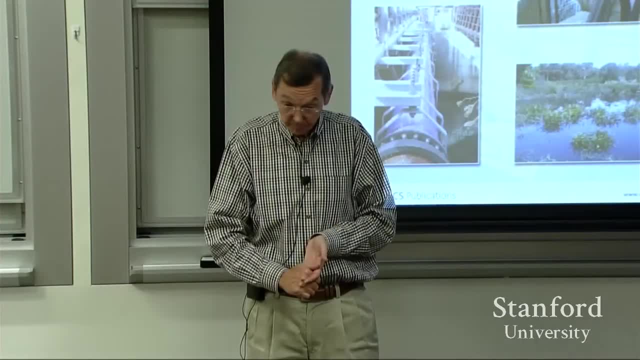 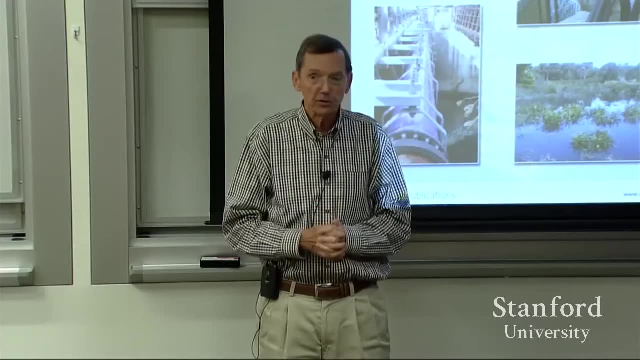 it's a combination of cities working together of um the stormwater capture and a desal facility And the desal will go. I think it's called Sand City. You know that's isn't that the place just north of uh. 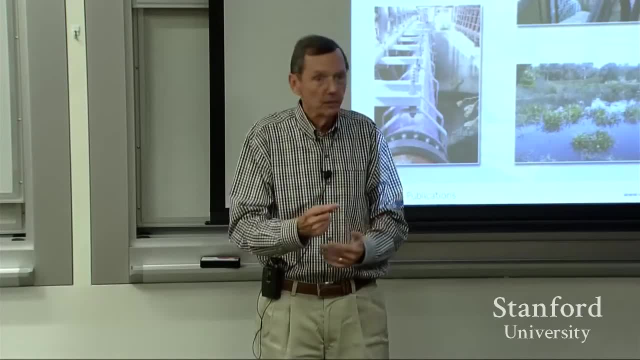 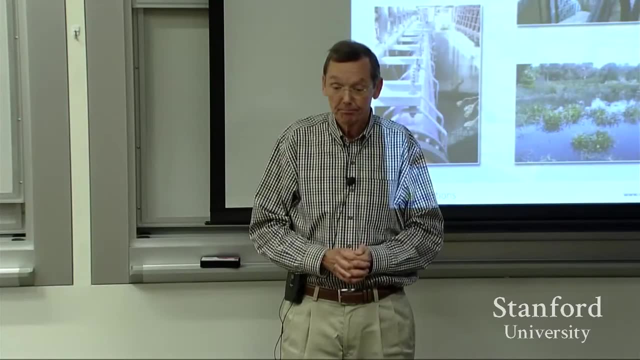 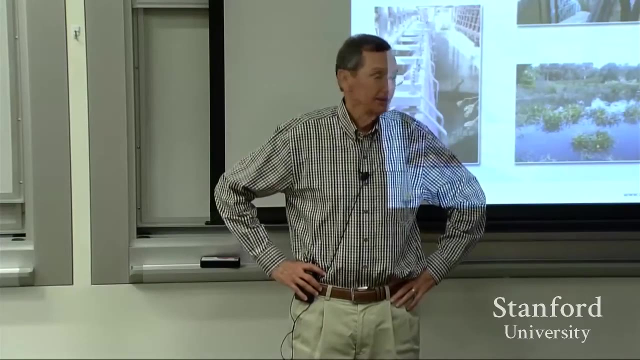 along the coast there, But there isn't a. there isn't, you know, one solution. It's: how do these different pieces work and fit together? I guess I could throw in the Carmel River one. I find that fascinating, you know. 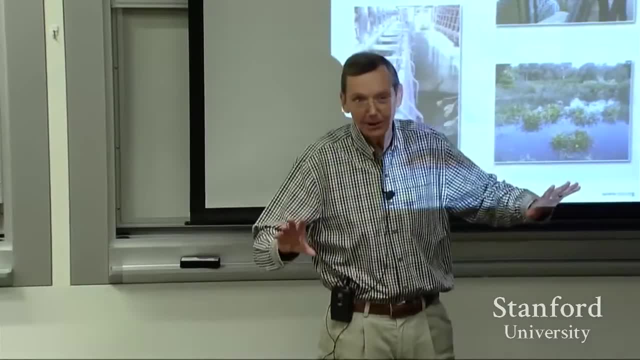 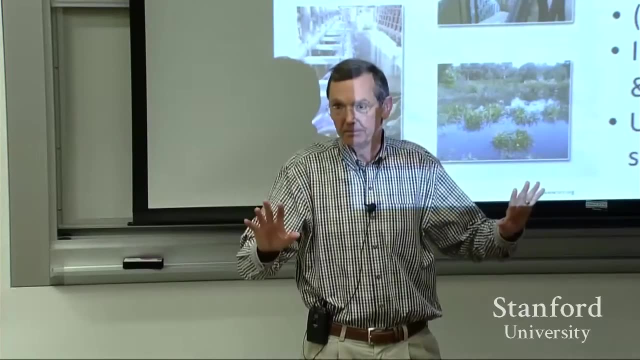 Yeah, Oh, one last thing about Carmel and the whole Salinas Valley. When they put in the State Water Project, uh, they didn't want to be a part of it. You all know where 152 is. You go over Pacheco Pass. 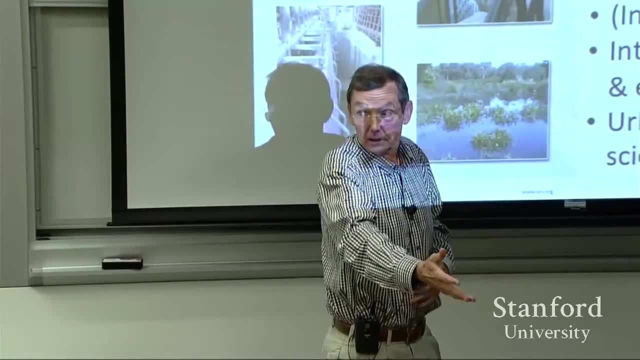 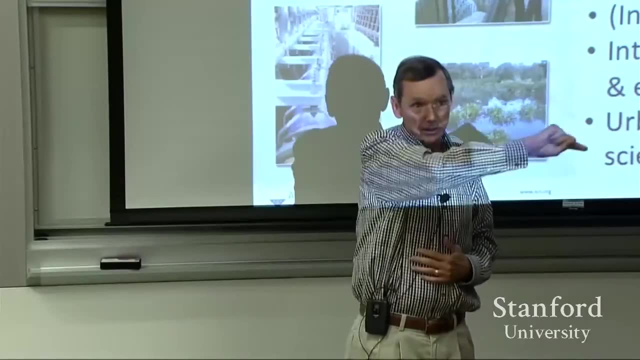 you know and you get there and you see the San Luis Reservoir. That's diverted water from the State Water Project. It's storage. We're tied into that. They built a little pipeline to take that water and put it in the Anderson Reservoir south. 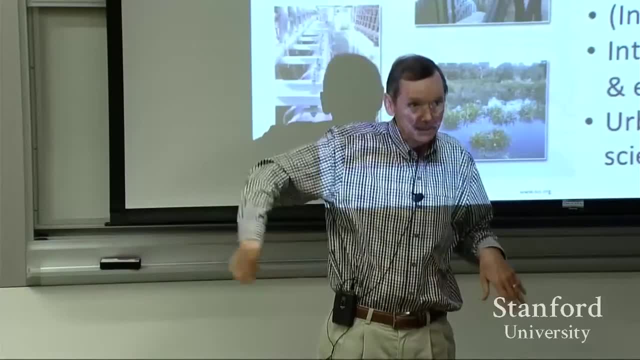 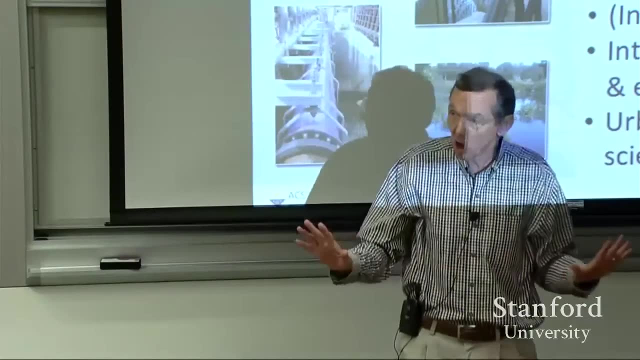 of San Jose, Monterey, when they were, when they were building that pipeline, Monterey had the opportunity to say: well, do you want us just to take a little extension and pull it over to you guys? They said no, Now we're going back. to when I was in high school. okay, Why did they say no? It's the same reason that Marin says no to lots of things about water: because they don't want. they didn't want urban development. More water would mean more development and they didn't want. 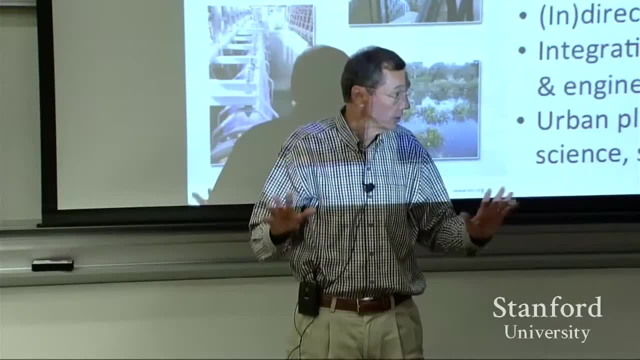 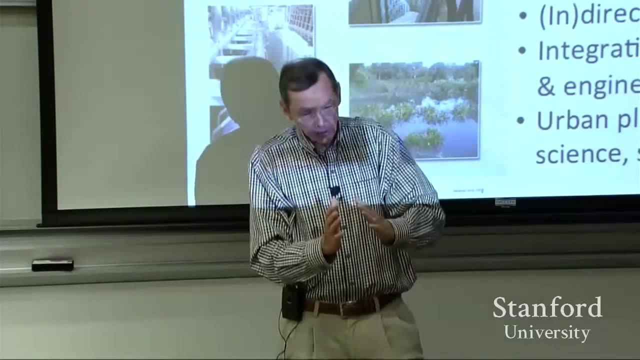 that Or there was a fear that one would lead to the other. So it's really interesting when you look at the Salinas Valley and Monterey as a piece of the state, they're really on their own. You have all this massive plumbing that can move water all over the state. 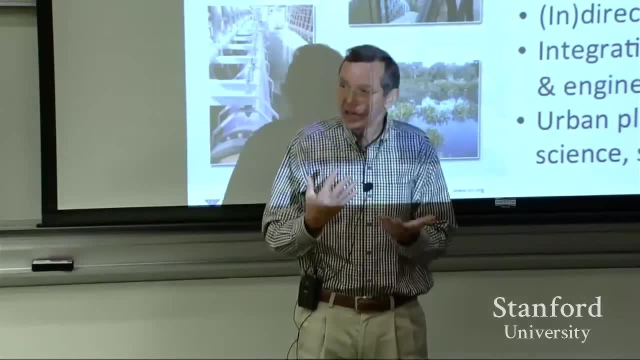 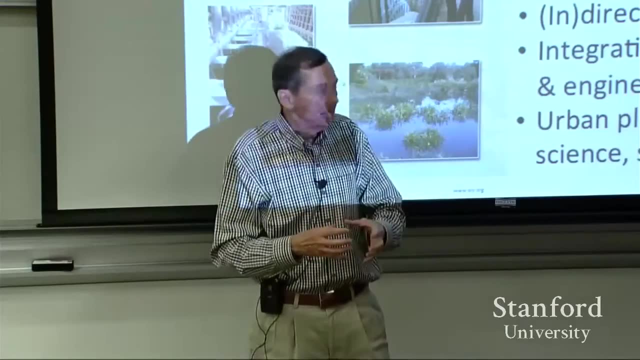 except right in there And I don't know. to me the Salinas Valley, Carmel, Monterey, Sand City, they're kind of like a little microcosm for the whole state. in a way, They're throwing the Carmel River instead. 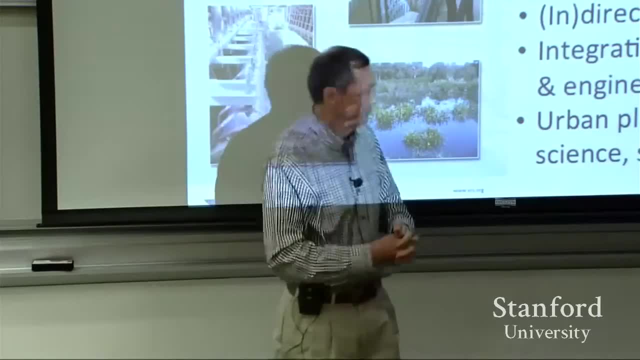 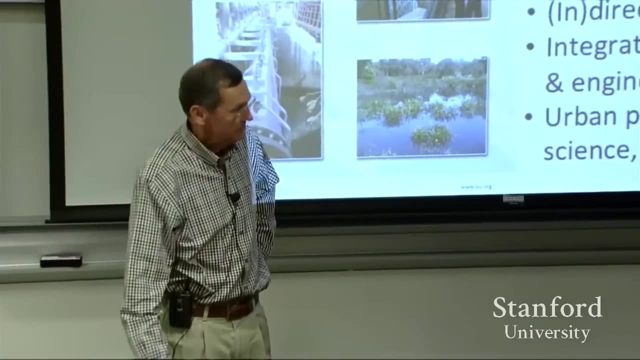 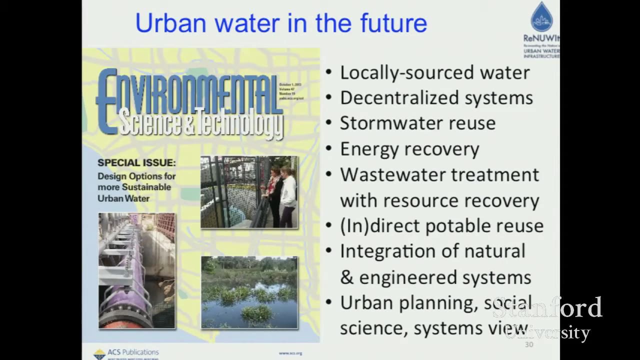 of the San Joaquin or Sacramento, Alright, So it sounded like the motivation for the distributed treatment network was largely the energy cost of pumping it over further distances. It's the energy cost and the reverse plumbing system that's needed. So I mean, it sounds like we already 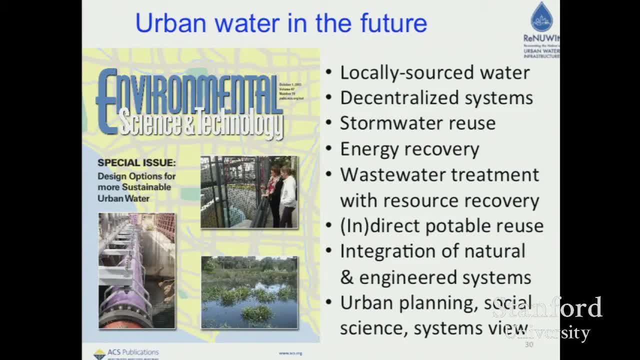 have a reasonable network set up for distribution based on the more centralized treatment. So I guess my question is: has the? has there been a consideration or study of what the costs are, from a financial standpoint and a carbon emission standpoint, of building all of these new decentralized treatments? 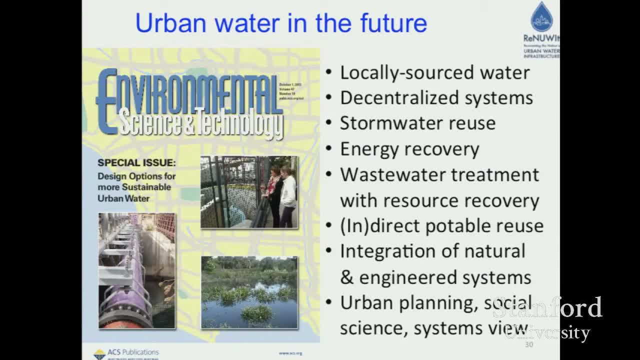 versus just installing, you know, clean energy sources to push the water around through the network that we currently have, because it seems like then you could have a more decentralized storage network that would be a lot less financially and energetically intensive process to set up. So 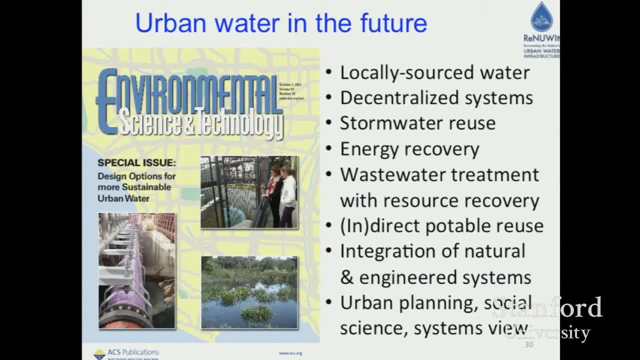 I mean, this is like dump trucks and all the stuff that you need is still going to burn a lot of carbon and can cost a lot of money to put in. No, that's part of the analysis that you do on this and when you look at these, 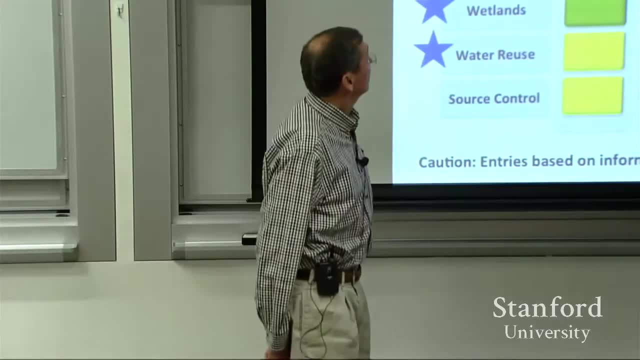 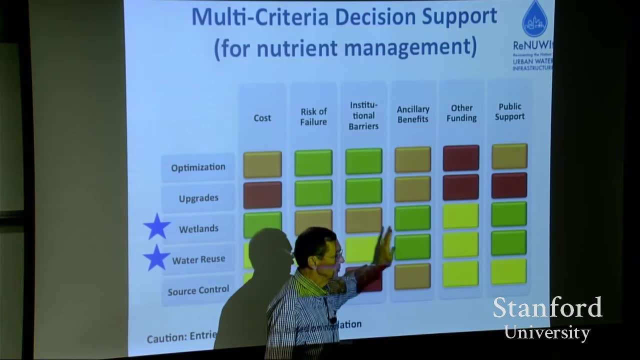 decentralized systems. you could put different categories here- Carbon emissions, capital costs, operating costs, public acceptance- and you have to step back then and say what does the community want, What would be value to them and what would work. So there isn't. 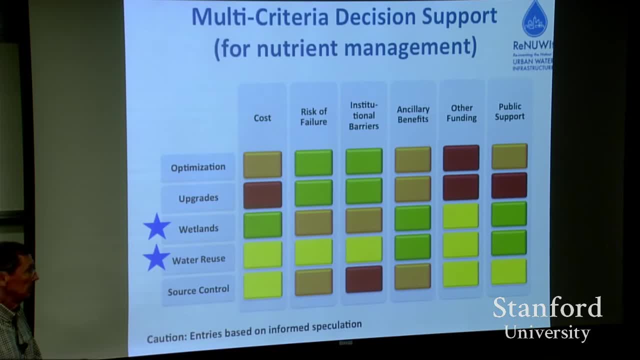 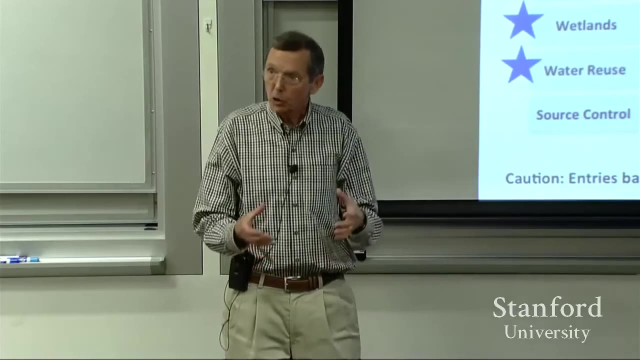 just one simple answer to your question. but it does come down to this: trying to weigh one alternative versus another And what's politically feasible. So I used the Stanford campus as an example. We're quirky here in the water reuse sense. Why are we quirky? 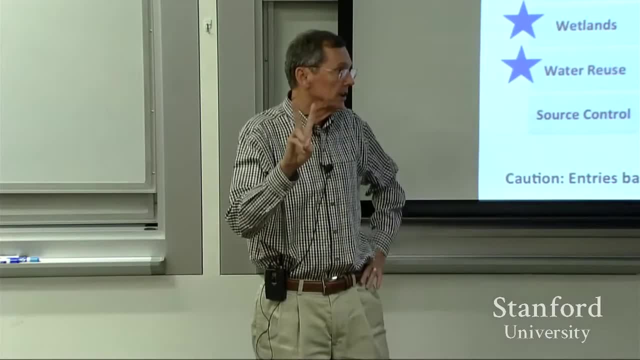 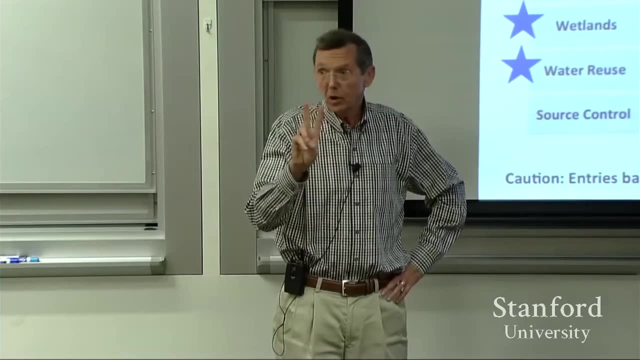 We have two water distribution systems on campus. Right where we sit now There are two water distributions. One of them is the water we drink. It's the water that comes from the Hetch Hetchy system, from the Yosemite National Park. Then there's another system. 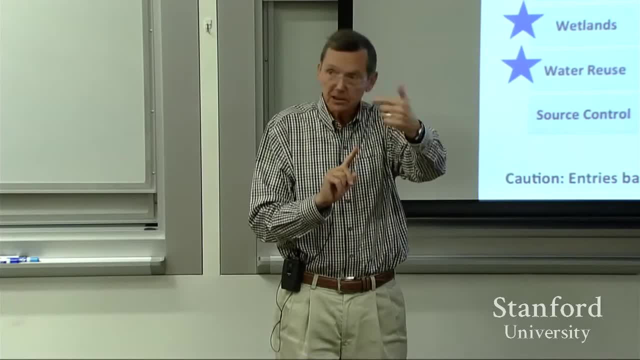 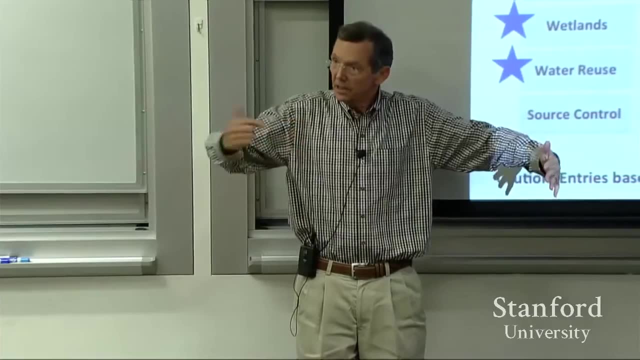 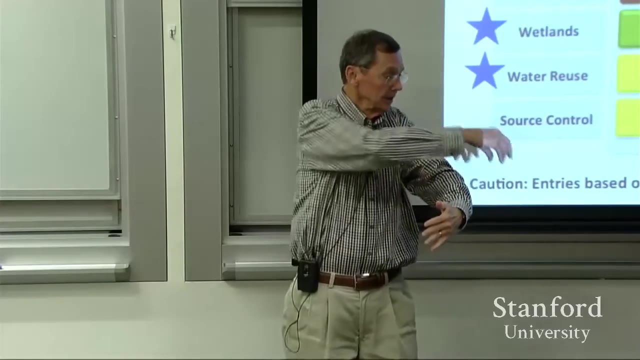 that's lake water from Felt Lake That comes over here and it's used for irrigation all around. everything inside the campus drive loop is on its own irrigation system with lake water. So imagine we take all of our wastewater- a million gallons a day- build. 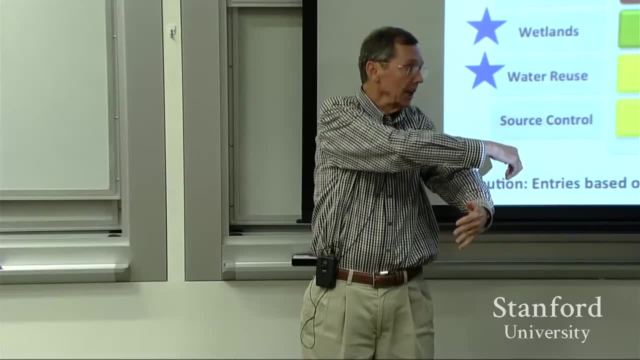 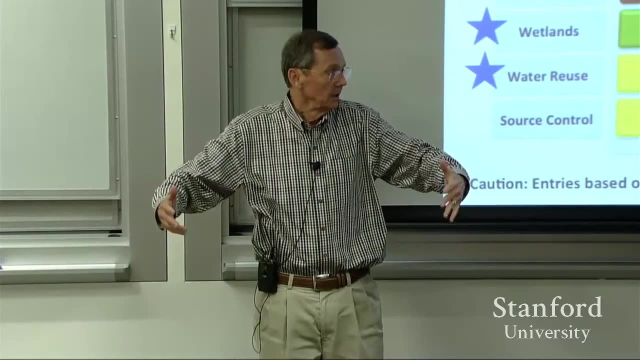 this little treatment system over here, reclaim easily half that water and put it into that irrigation system. Now we don't have to use Hetch Hetchy water So, but we're using that for irrigation. We're using this reclaimed water for irrigation and we just happen to have 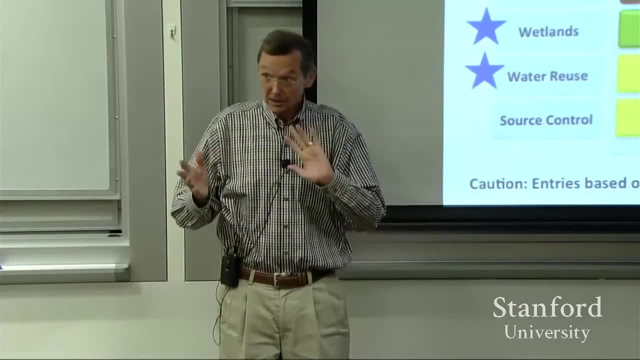 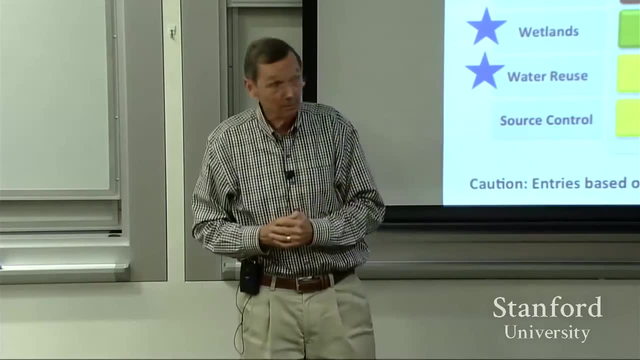 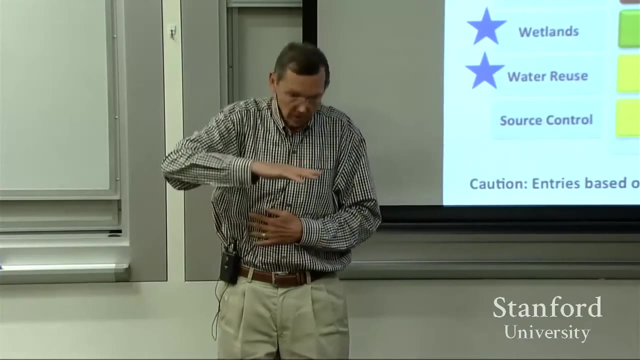 a separate distribution network. So why would Stanford want to invest a few million dollars in this treatment facility? Well, it's say: well, how are we going to meet our water supply needs in the future If we get in drought? your water gets cut back. we're not going to. 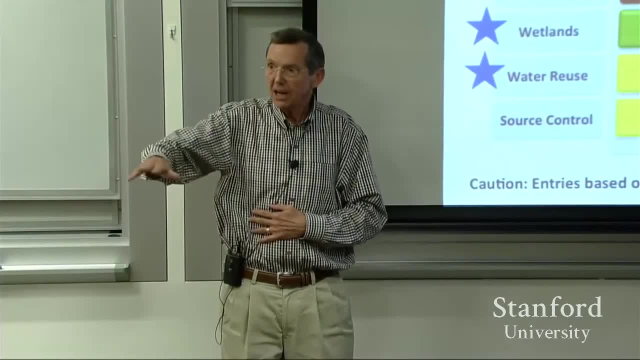 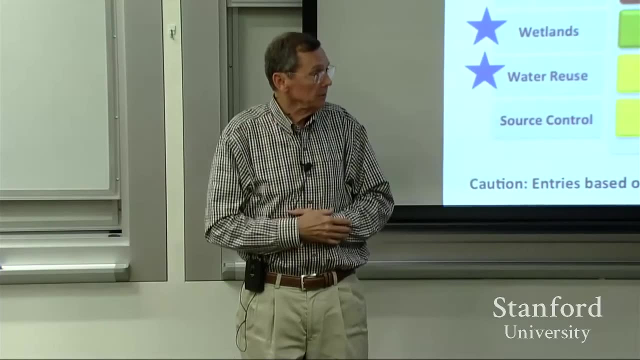 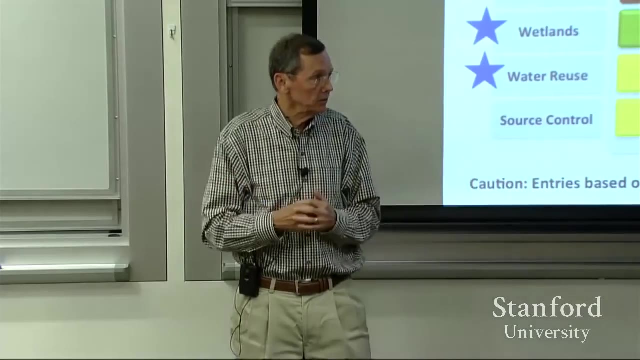 get any more water from the Hetch Hetchy system ever It's tapped out. So our future is like we need to sort of have drought proof water for the Stanford campus, And one way that seems pretty logical here is to think about taking advantage of this second distribution system. 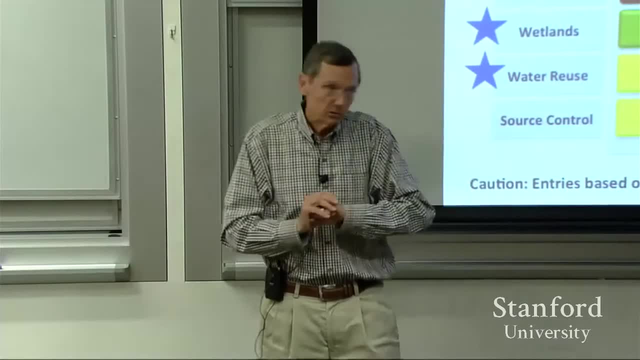 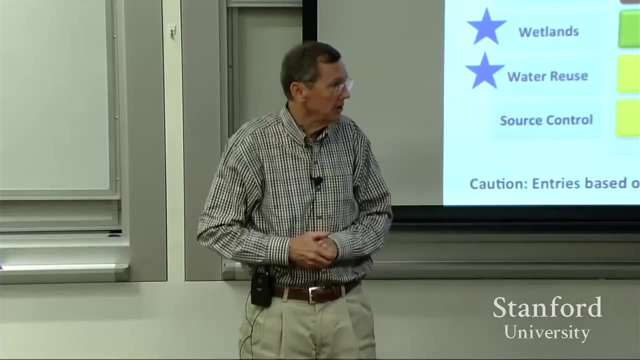 And the other one would be- I live on campus- is extending that over to our neighborhood? They used to do it a long time ago. In fact, I have a spigot in my backyard where it used to come. They cut that pipe, So 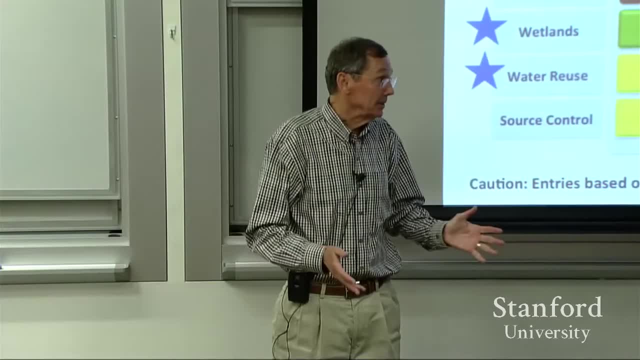 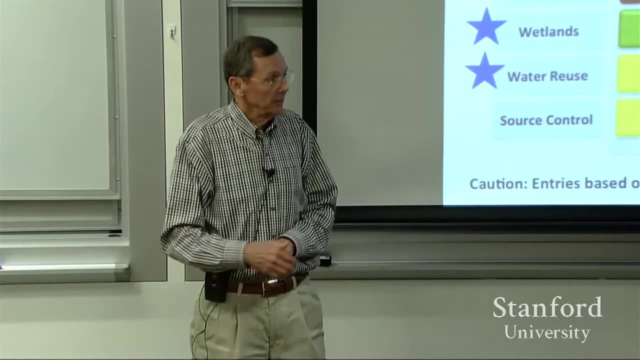 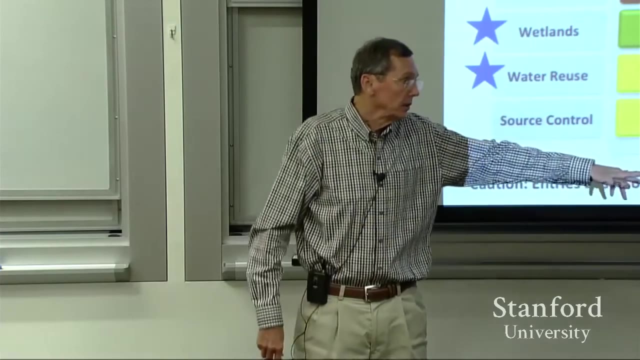 I answered your question by an example, And it's: this idea of the satellite treatment plant is very attractive for the Stanford campus. The other thing is it has low salt content too When you get down near the bay. let's say we did do the centralized treatment. 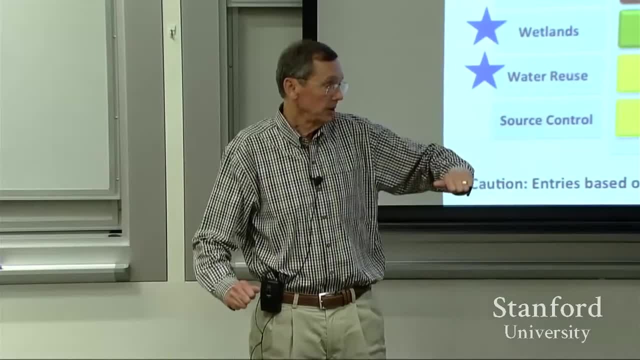 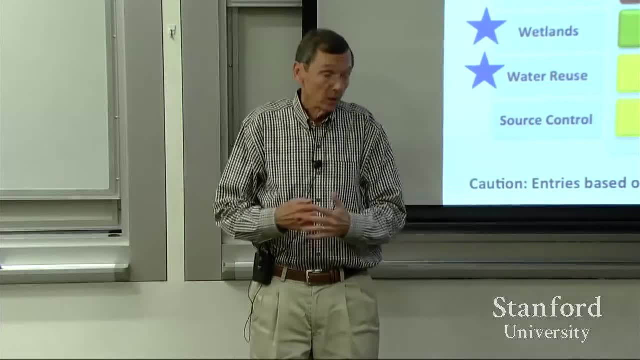 And then you put this big purple pipe up in Barcadero Avenue to the Stanford campus. What you'll find over time is, because of the kind of plants we've put here, like redwoods, the water's too salty for long term irrigation with that. 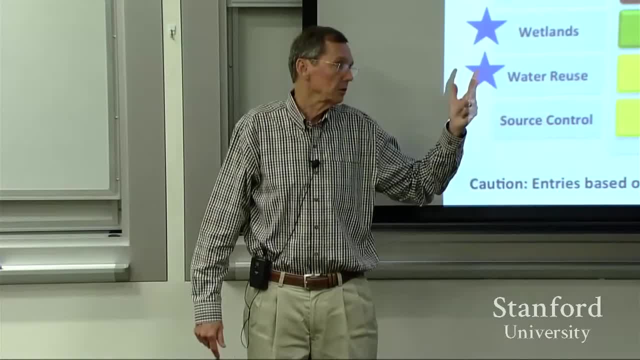 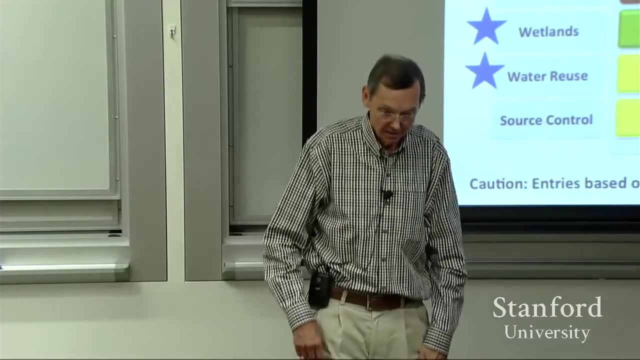 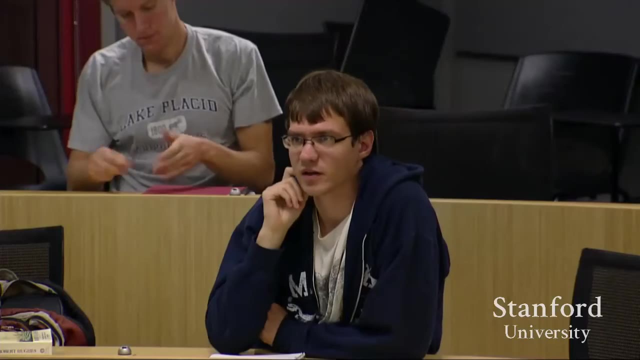 So it's the combination of the purple pipe, the energy backwards and the higher salt. Yeah, I have a basic question on indirect and recycled water. Are you talking about like gray water systems or is this like sewage that you're talking about recycling? Well, a lot of what we're talking. 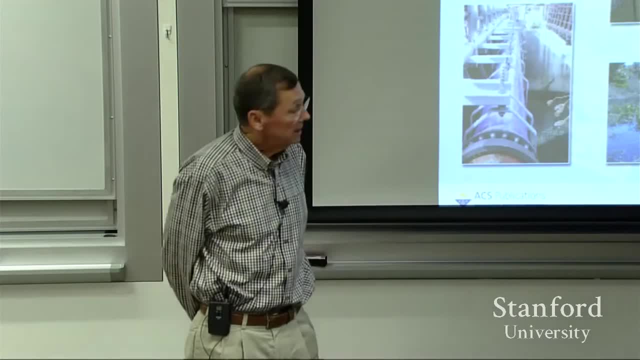 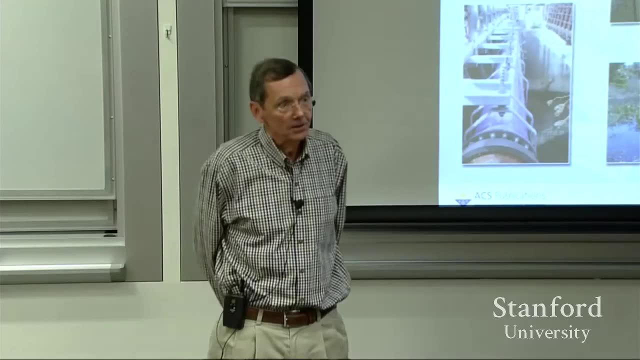 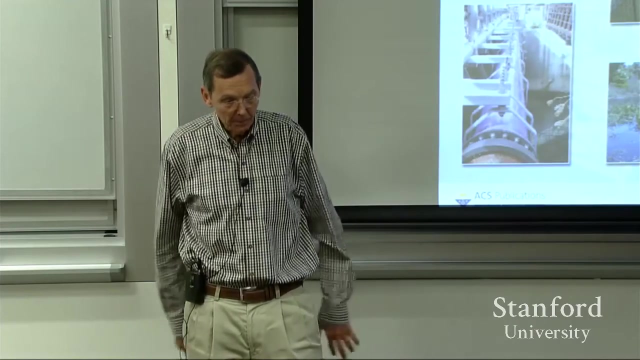 about here are larger systems that would be of some scale. Now, gray water, that's sort of like shower water and that kind of thing, Wash water That's popular at the scale of maybe a home And part of this idea of thinking about decentralized. 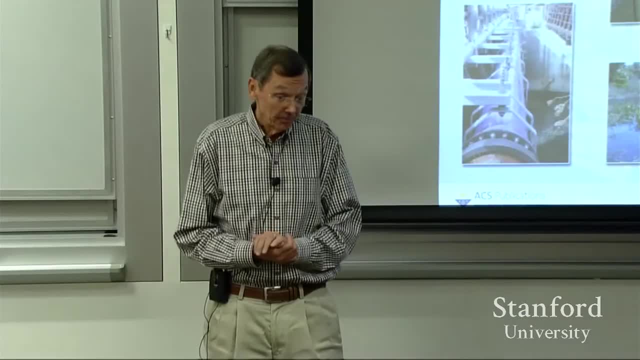 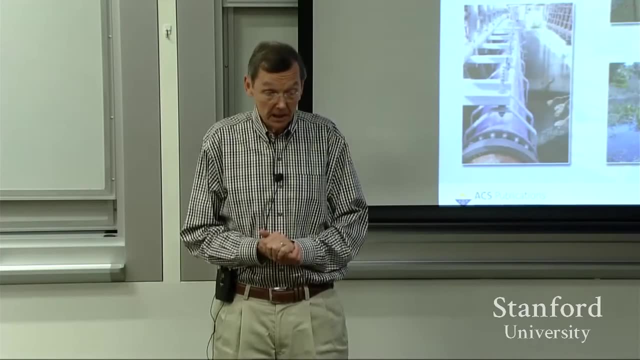 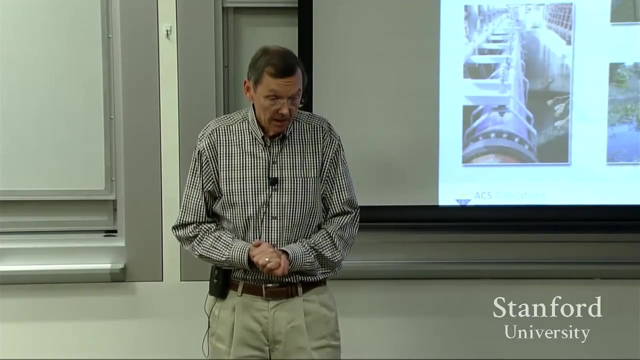 systems is: how decentralized do you want to go? And gray water reuse is something that is attractive with the public. It needs to be done safely And you know and the like, But it's something that's allowed. Maybe, in terms of decentralized systems, you'd probably look. 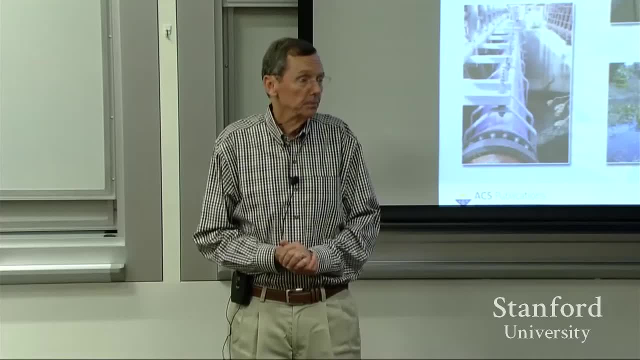 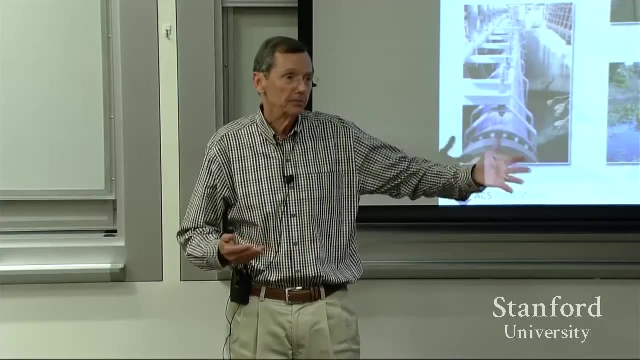 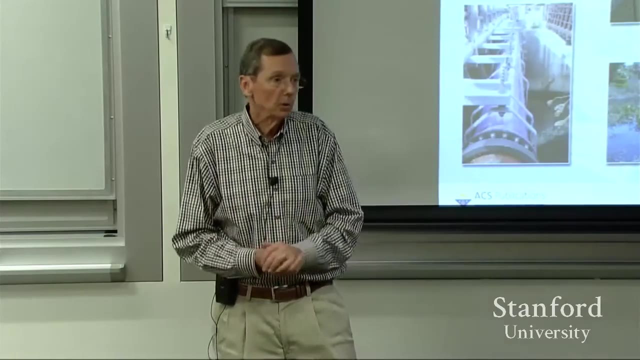 more at. you know new apartment buildings or big office complex or something like that. Or maybe you look at, say the new, you know that new Google, not Google Apple. You know the Apple headquarters that looks like a great big spaceship. Well, there's going to be a lot of water there. 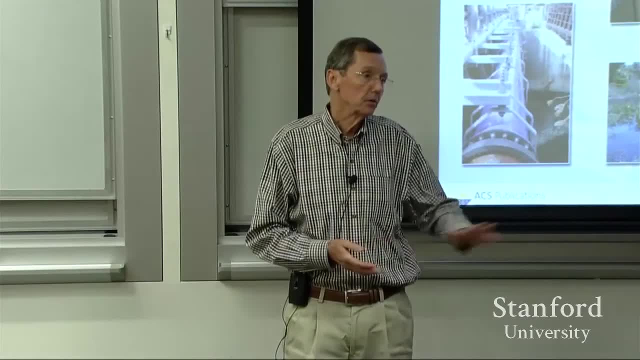 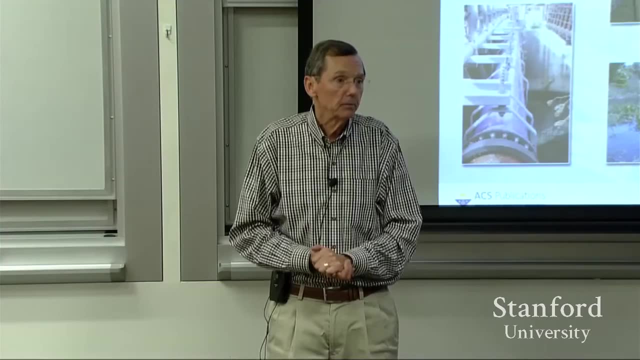 So you say, well, that's a place where you could take all kinds of gray water and do something with it. Or the same thing over with the Google campus in Mountain View. So it's done. And there's a lot of you know it's done. 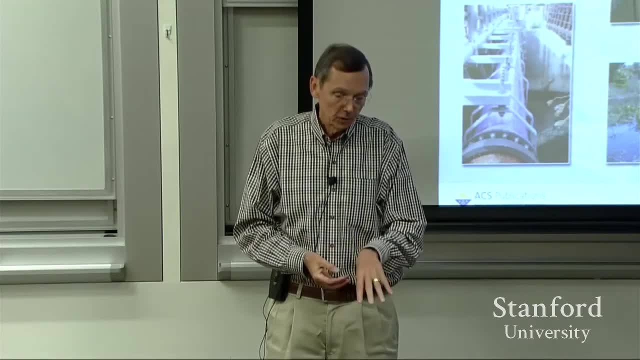 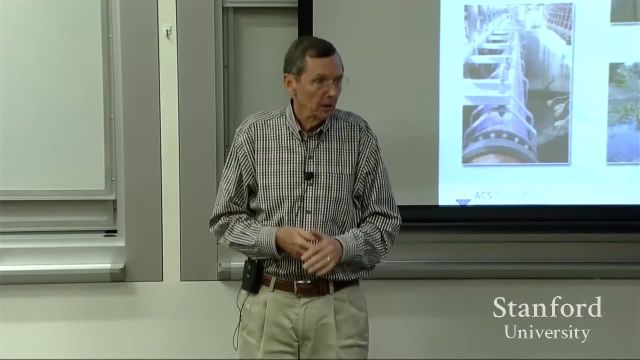 and there are ways you can do this and replumb your house. So it's at the scale of a home. I and some other folks you know always sort of worry a little bit about the public health consequences of it If you, the people that do it now, 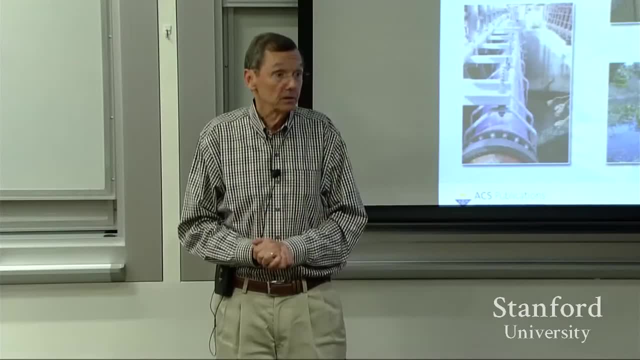 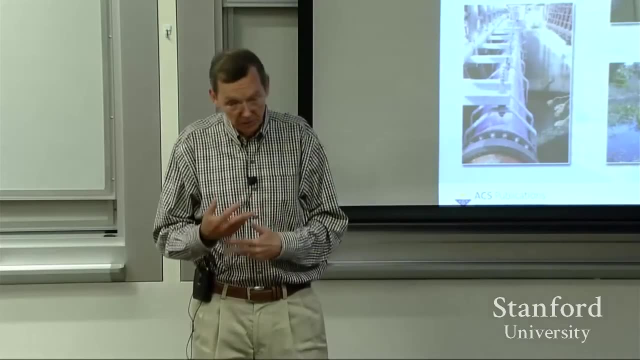 I think, are you know, real conscious of what they're doing? But if you said everyone's going to do this, then all you have to have is some contamination in that water and maybe you need to say: well, I should be concerned about pathogens, It's not chemicals.